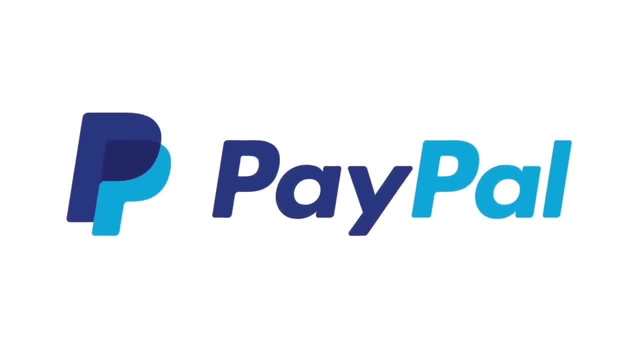 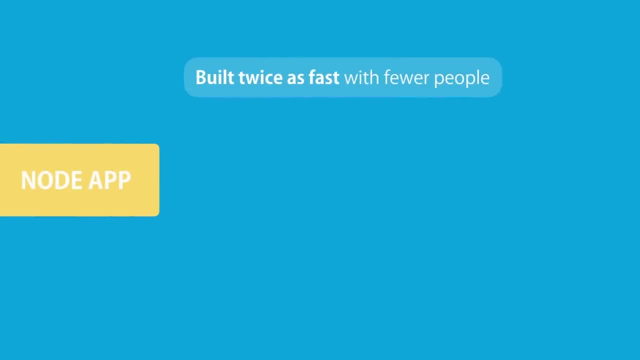 épisodeindexcom page. They rebuilt one of their Java and Spring-based applications using Node and they found that their Node application was built twice as fast with fewer people, in 33 percent fewer lines of code and 40 percent fewer files And, more importantly, they doubled the. 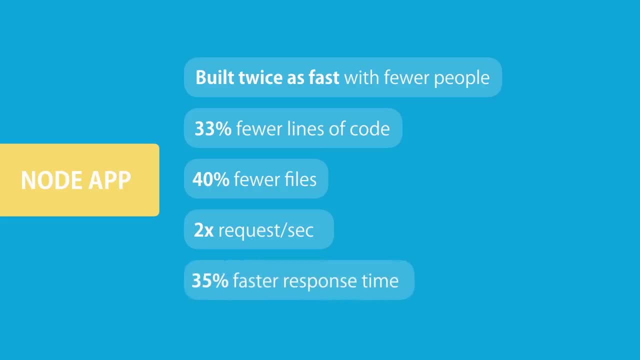 number of requests served per second, while decreasing the average response time by 35 percent. So Node is an excellent choice for building highly scalable services and long-term coding instructions for your câns respirations as well as user Protéger as well as Virtual Gentium, like basically just being able to runきます for every cellаст, like open- какая. 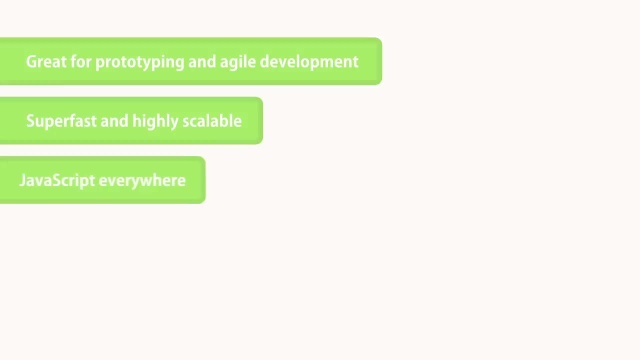 services. Another reason for using Node is that in Node applications we use JavaScript. So if you're a front-end developer and know JavaScript, you can reuse your JavaScript skills and transition to a full-stack developer and get a better job with better pay. You don't have to learn a new. 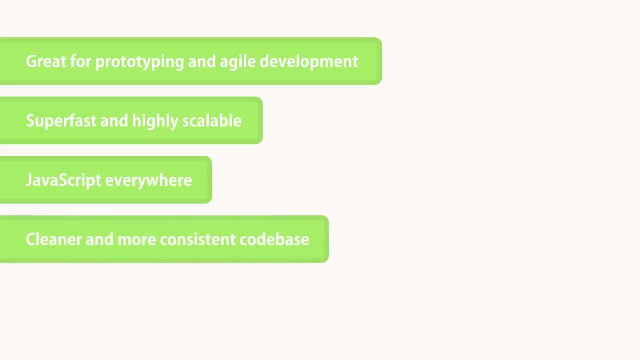 programming language. Also, because you can use JavaScript both on the front-end and on the back-end, your source code will be cleaner and more consistent, So you will use the same naming conventions, the same tools and the same best practices. And finally, another reason for using: 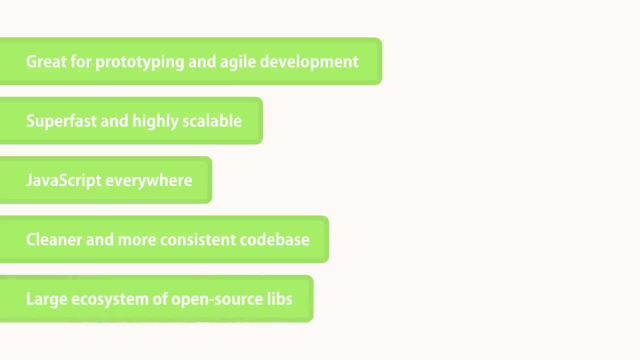 Node is that it has the largest ecosystem of open-source libraries available to you. So for pretty much any features or building blocks you want to add to your application, there is some free open-source library out there that you can use, So you don't have to build these building. 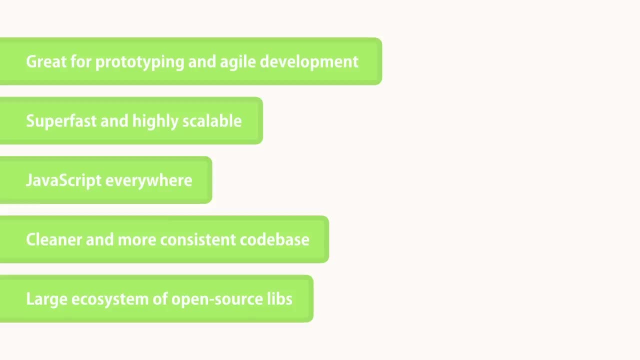 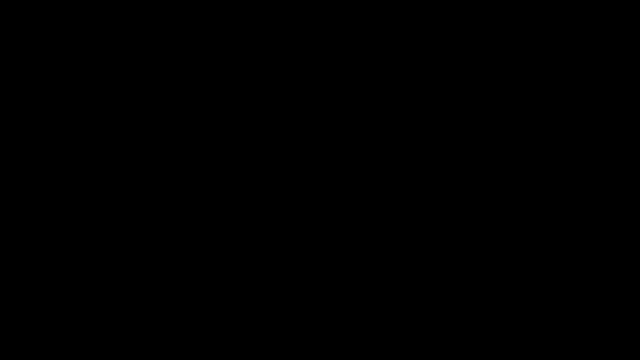 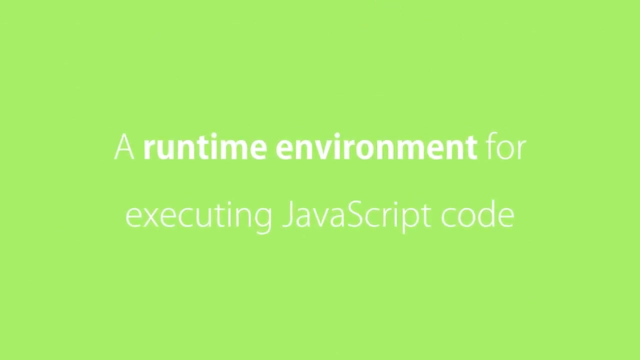 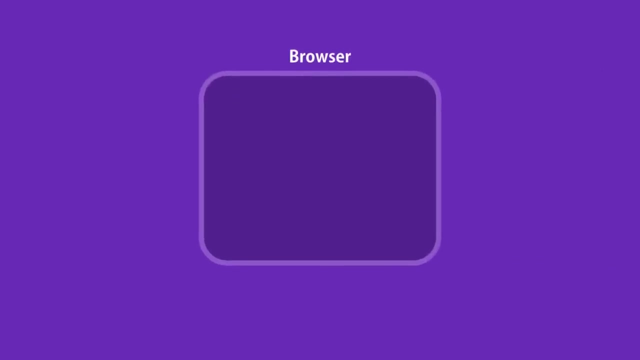 blocks from scratch and instead you can focus on the core of your application. Next, we're going to look at the architecture of Node. So in the last video, you learned that Node is a runtime environment for executing JavaScript code. But what is a runtime environment really? Well, before Node, we used JavaScript only to build. 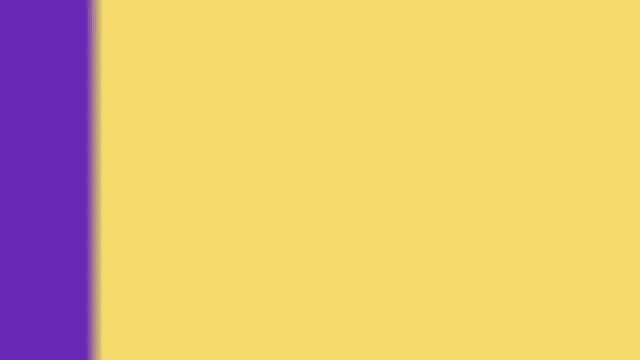 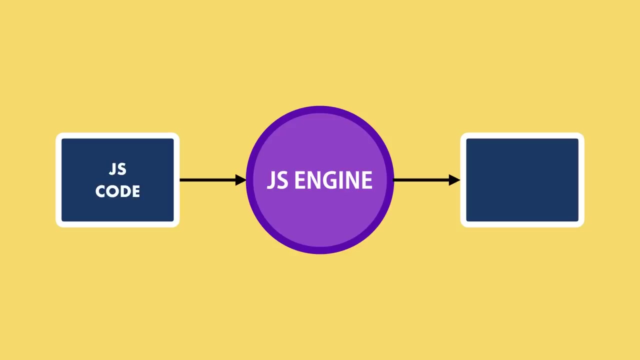 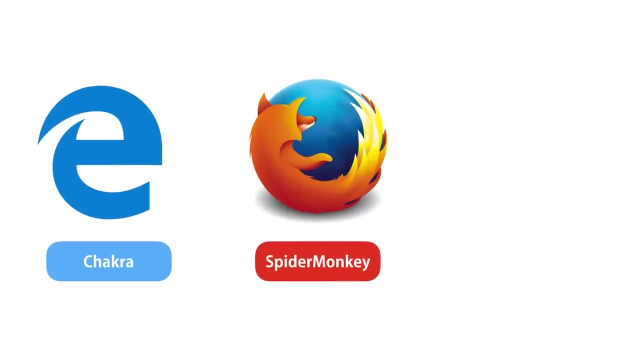 applications that run inside of a browser. So every browser out there has what we call a JavaScript engine that takes our JavaScript code and converts it to code that a computer can understand. For example, Microsoft Edge uses Chakra, Firefox uses SpiderMonkey and Chrome uses V8. And it's. 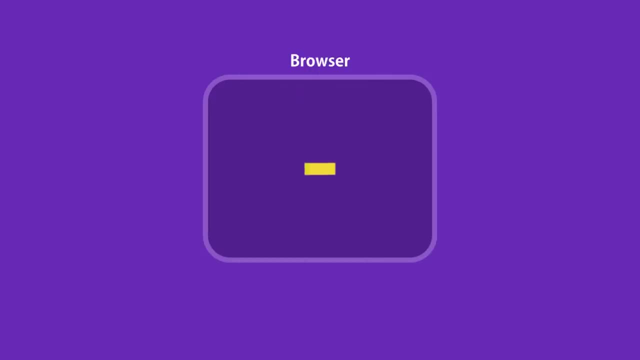 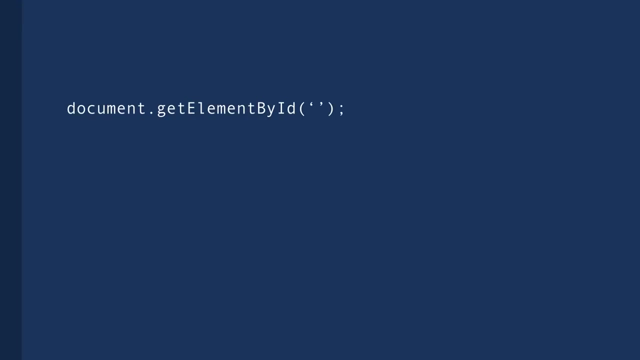 because of these varieties of engines that sometimes JavaScript code can behave differently in one browser or another. Now a browser provides a runtime environment for JavaScript code. For example, you probably know that in browsers we have the window or the document object. These objects allow us to 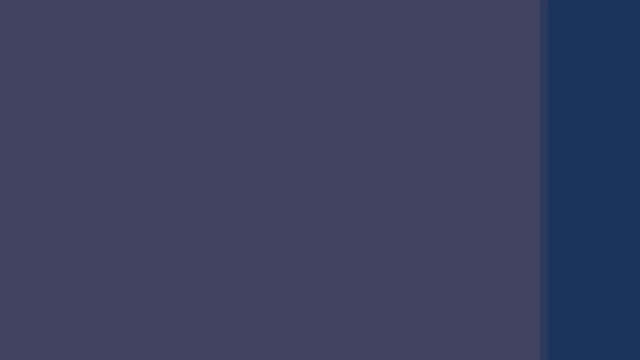 work with the environment in which the code is being executed. So, for example, if we want to run a program, we can run a program in which the code is running Now, after 2009,. the only way to execute JavaScript code was inside of a browser. In 2009,, Ryan Dahl, the creator of Node, came up with a 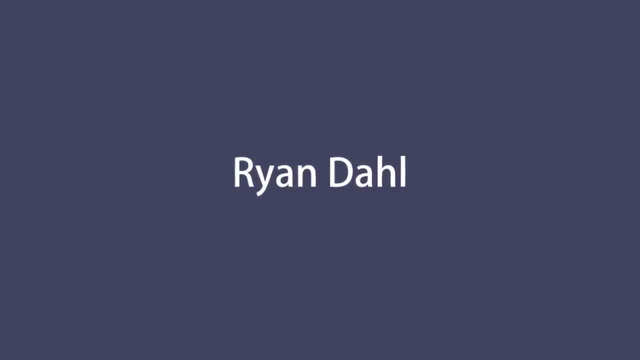 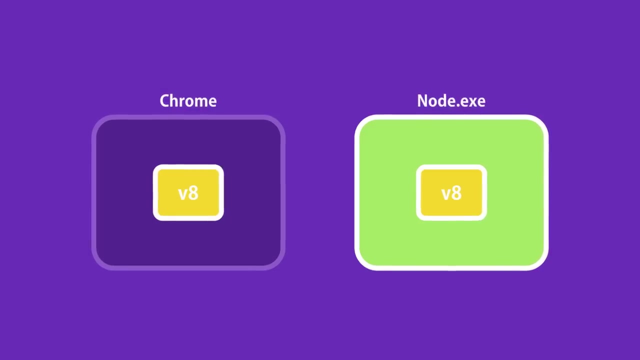 brilliant idea. He thought it would be great to execute JavaScript outside of a browser. So he took Google's V8 engine, which is the fastest JavaScript engine out there, and embedded it inside a C++ program and called that program Node. So, similar to a browser, Node is a runtime environment for JavaScript code. It contains a. 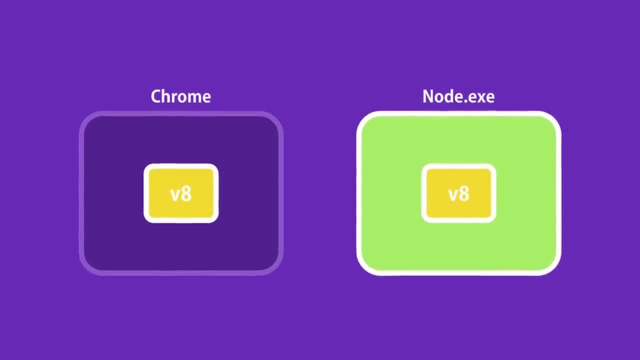 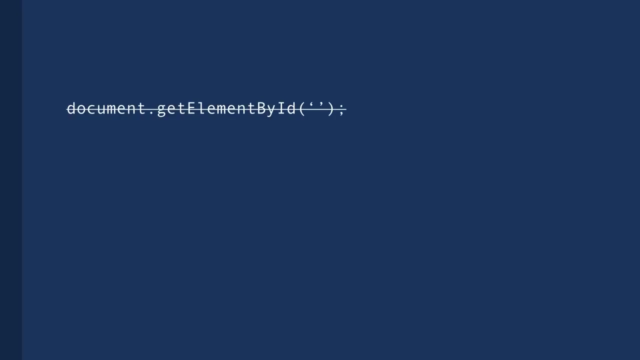 JavaScript engine that can execute our JavaScript code, But it also has certain objects that provide an environment for our JavaScript code. But these objects are different from the environment objects we have in browsers. For example, we don't have the document object. Instead we have other objects. 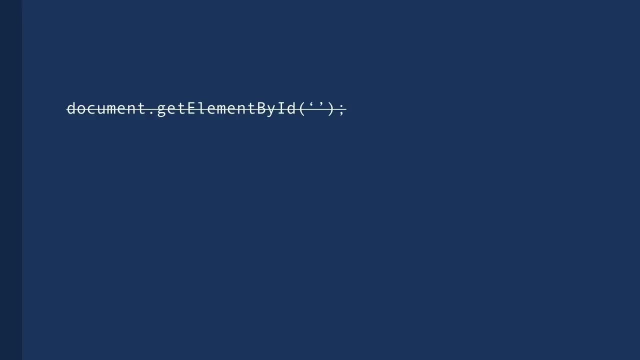 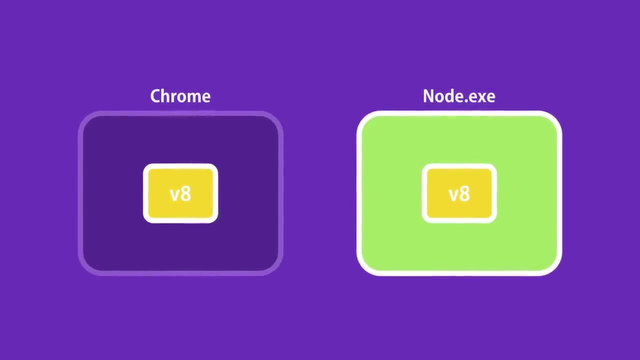 that give us more interesting capabilities. For example, we can work with the file system, listen for requests on a given port, and so on. We can't do stuff like that inside of a browser, right? So, in essence, Node is a program that includes the V8 JavaScript engine plus some additional. 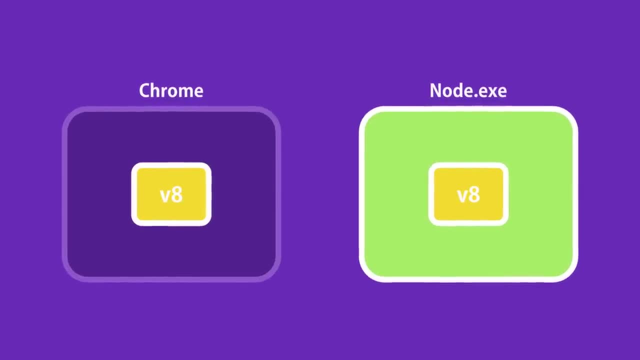 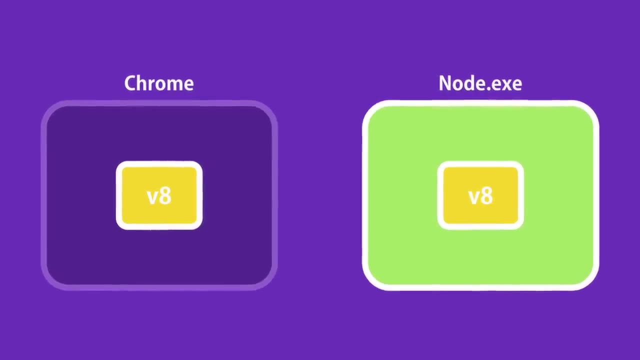 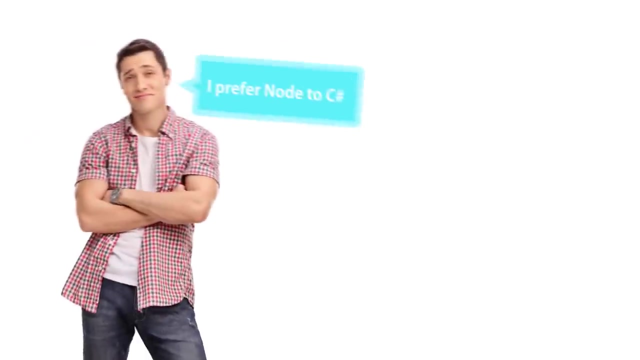 modules that give us capabilities not available inside browsers. We can work with the file system or the network, and so on. Both Chrome and Node share the same JavaScript engine, but they provide different runtime environments for JavaScript. I've seen people comparing Node to C, Sharp or Ruby or some other programming languages. 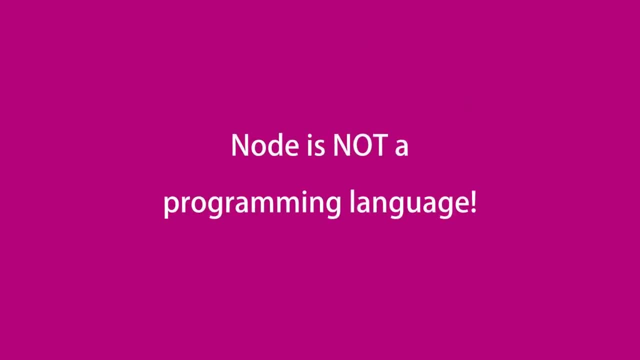 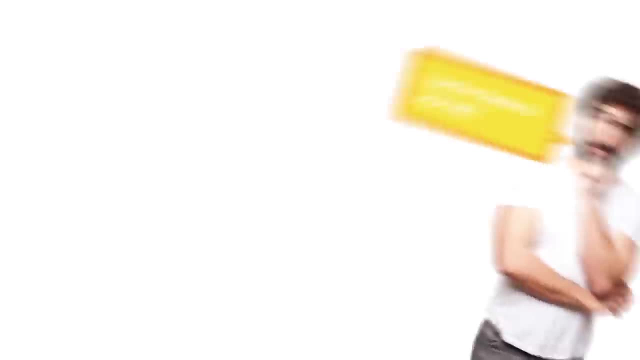 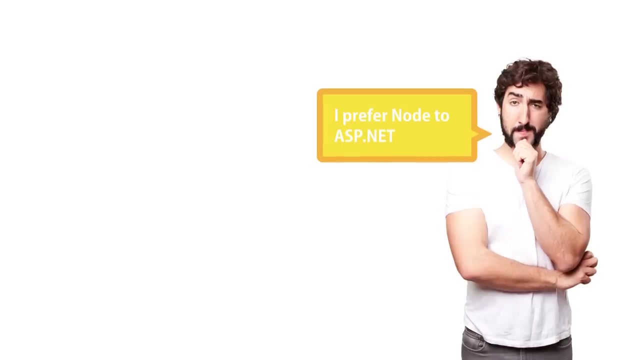 But these comparisons are fundamentally wrong Because Node is not a programming language. It's like comparing a car with an apple. By the same token, Node should not be compared with frameworks such as ASPNET or Rails or Django and so on. These are frameworks for 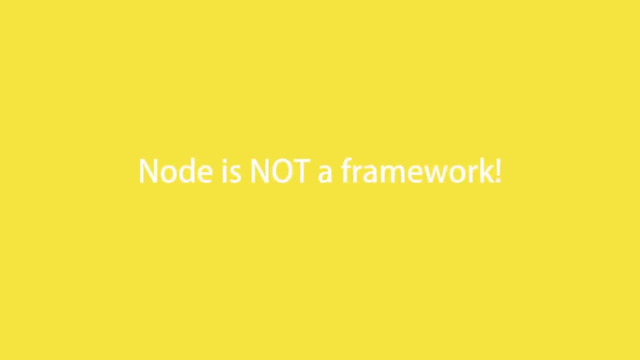 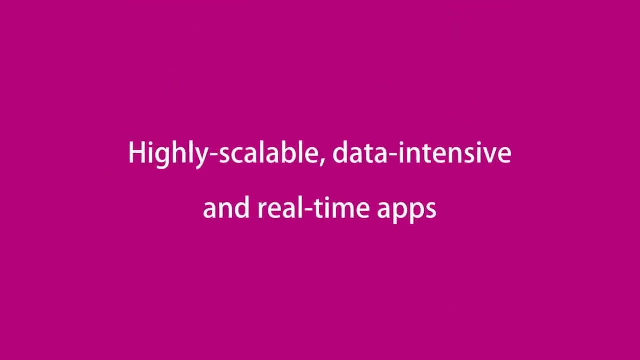 building web applications. Node is not a framework. It's a runtime environment for building JavaScript code. Next we're going to look at how Node works. So earlier I mentioned that Node applications are highly scalable, and this is because of the non-blocking or asynchronous nature of Node. 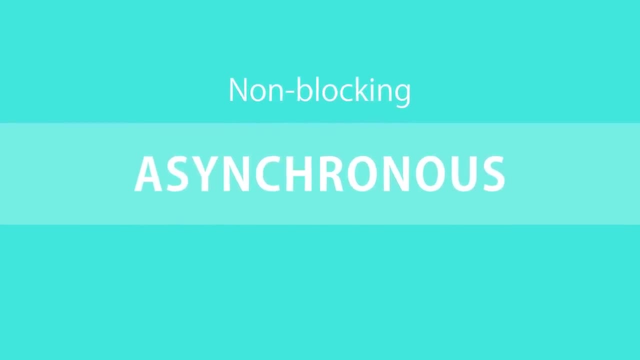 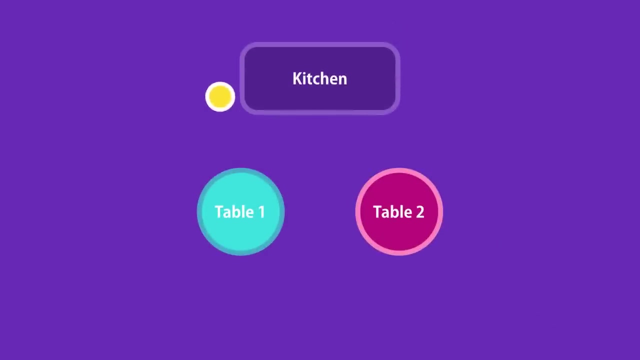 What do I mean by asynchronous? Let me give you a metaphor. Imagine you go to a restaurant. A waiter comes to your table, takes your order and gives it to the kitchen. Then they move on to serve another table while the chef is preparing your meal. So the same person can serve many different tables. 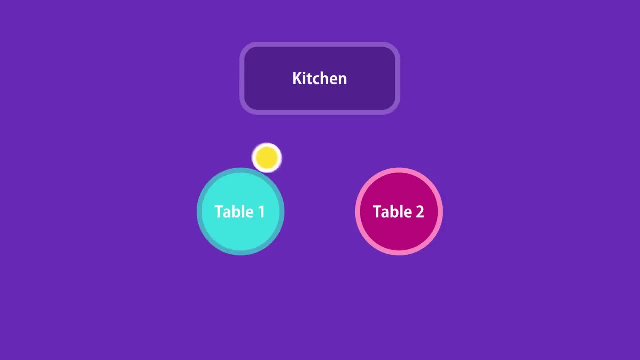 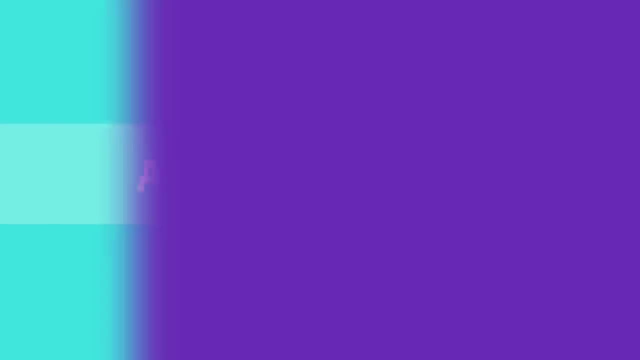 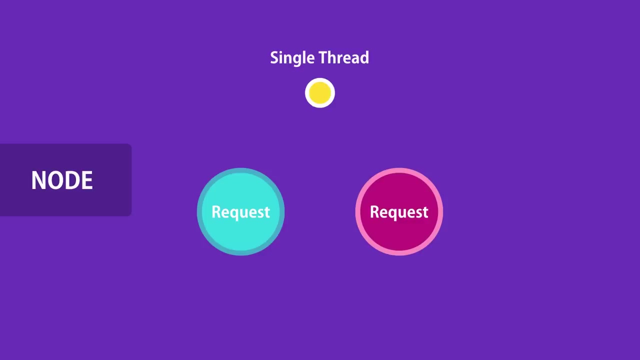 They don't have to wait for the chef to cook one meal before they serve another table. This is what we call non-blocking or asynchronous architecture, And this is how Node applications work. The waiter is like a thread allocated to handle a request, So a single thread is used. 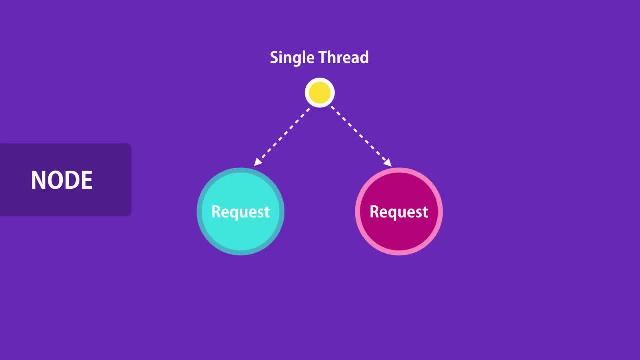 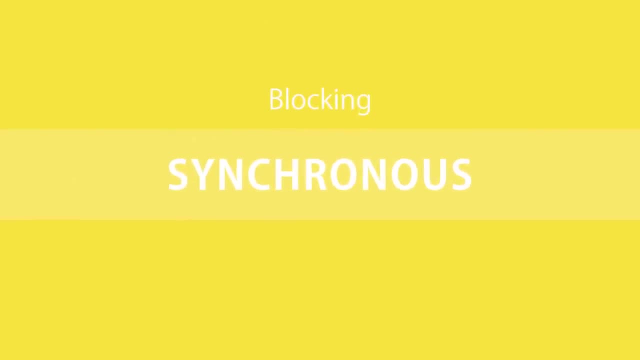 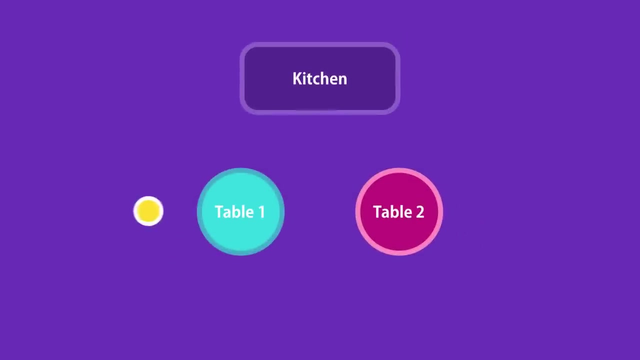 to handle multiple requests. In contrast to non-blocking, we have non-blocking or asynchronous architecture. We have blocking or synchronous architecture. Let's see how that works. So back to our restaurant example. imagine you go to another restaurant and in this restaurant a waiter is allocated to you. 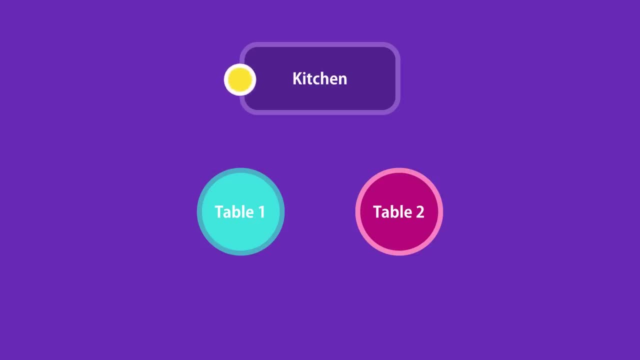 They take your order and give it to the kitchen. Now they're sitting in the kitchen waiting for the chef to prepare your meal At this time. they're not doing anything else, They're just waiting. They're not going to take an order from another table until your meal is ready. 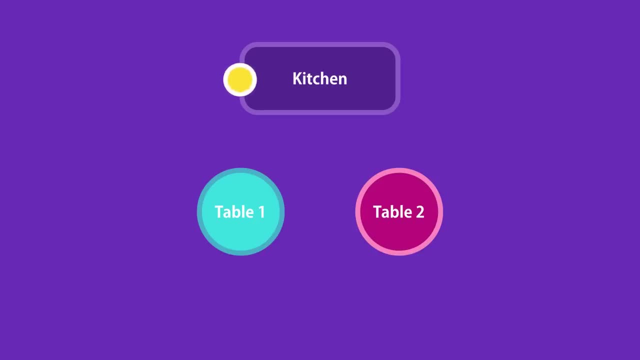 This is what we call blocking or synchronous architecture, And that's how applications built with frameworks like ASPNET or Rails work out of the box. So when we receive a request on the server, a thread is allocated to handle that request As part of handling that request. 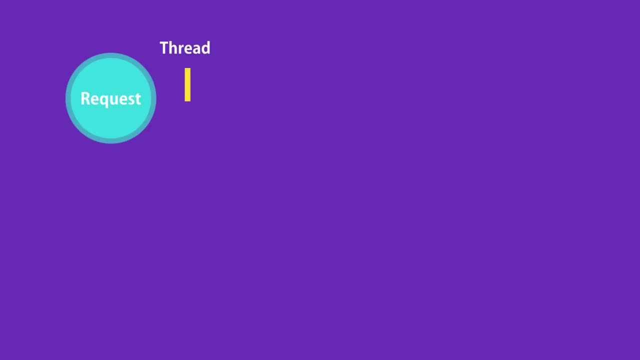 it is likely that we're going to query a database And, as you know, sometimes it may take a little while until the result is ready. When the database is executing the query, that thread is sitting waiting. It can't be used to serve another client, So we need a new thread to serve another client. Now imagine what would happen if we have a large number of concurrent clients. At some point we're going to run out of threads to serve these clients, So new clients have to wait until free threads are available. Or if we don't want them to wait, we need to add more. 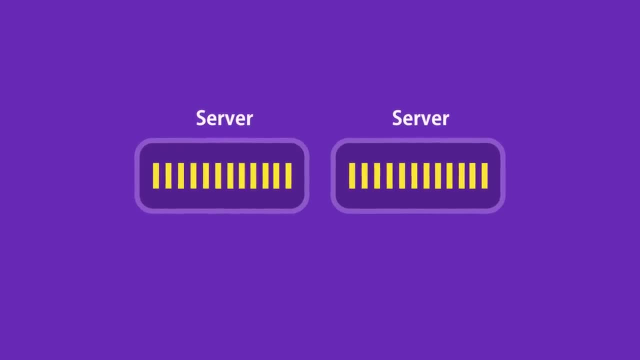 hardware. So with this kind of architecture, we are not utilizing our resources efficiently. This is the problem with blocking or synchronous architecture And, as I explained, that's how applications built with frameworks like as Color, sigh, slash… used ASPnet that work by default. 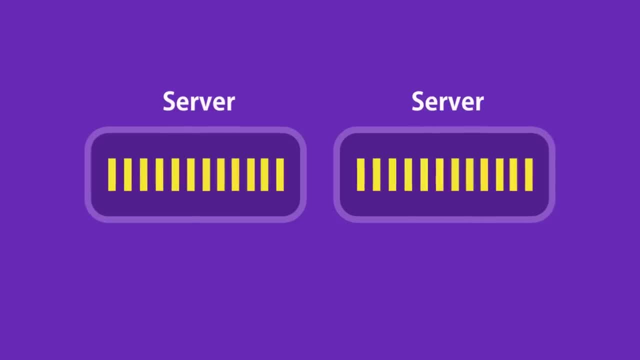 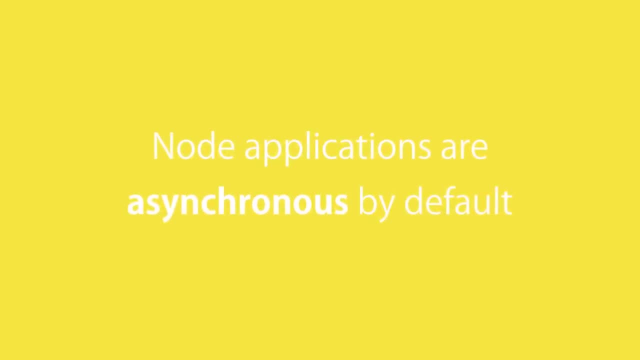 Of course in as bluenet it is possible to use a synchronous architecture, but you will have to do some extra work for that. in contrast, node knows the applications are asynchronous by default, so you don't have to do anything extra. In node we have a single thread to handle all requests. 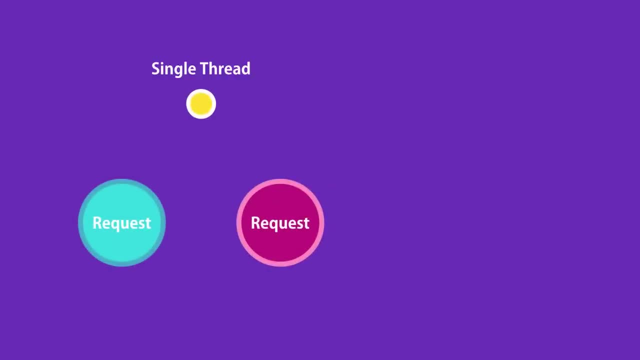 When a request arrives, that sequence goes away. single thread is used to handle that request. If we need to query a database, our thread doesn't have to wait for the database to return the data While the database is executing our query. that 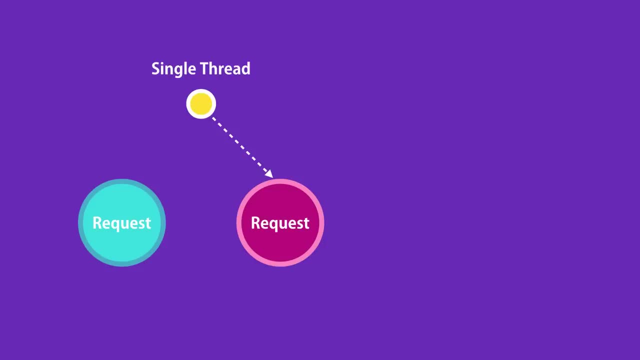 thread will be used to serve another client. When the database prepares the result, it puts a message in what we call an event queue. Node is continuously monitoring this queue in the background. When it finds an event in this queue, it will take it out and process it. This kind of architecture makes 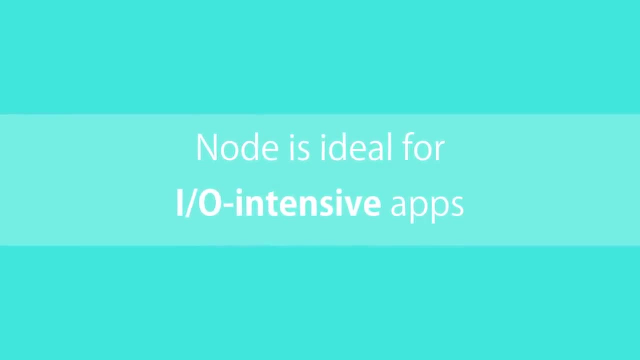 Node ideal for building applications that include a lot of disk or network access. We can serve more clients without the need to throw in more hardware, and that's why Node applications are highly scalable. In contrast, Node should not be used for CPU-intensive applications like a video encoding. 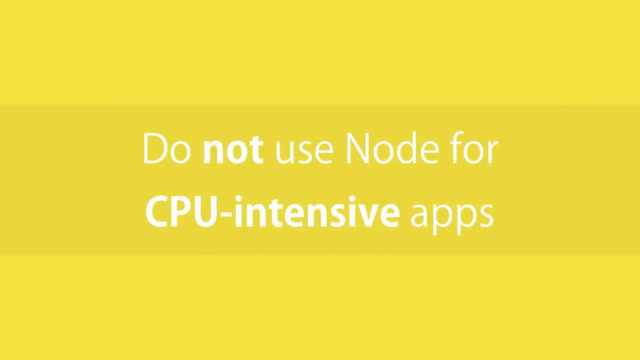 or an image manipulation service. In this context, Node should not be used for CPU-intensive applications like a video encoding or an image manipulation service- This kind of applications. we have a lot of calculations that should be done by CPU and few operations that touch the file system or the network. Since Node 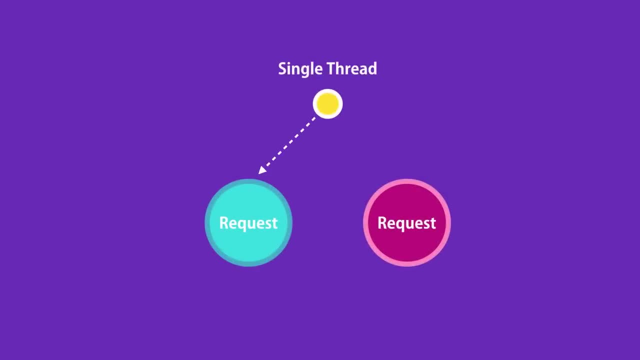 applications are single threaded. when performing the calculations, to serve one client, other clients have to wait, And that's why Node should not be used for CPU-intensive applications. It should only be used for building data-intensive and real-time applications. Okay, enough theory. Next I'm going. 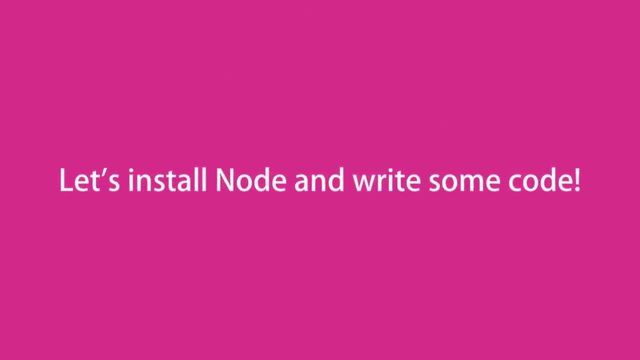 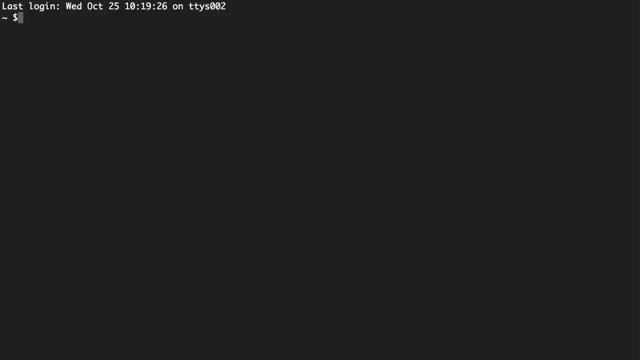 to show you how to install Node and build your first Node application. In this lecture I'm going to show you how to install Node. If you're on Windows, open up Command Prompt. If you're on Mac or Linux, open up the terminal. First, let's see if you already have Node on your machine or not. 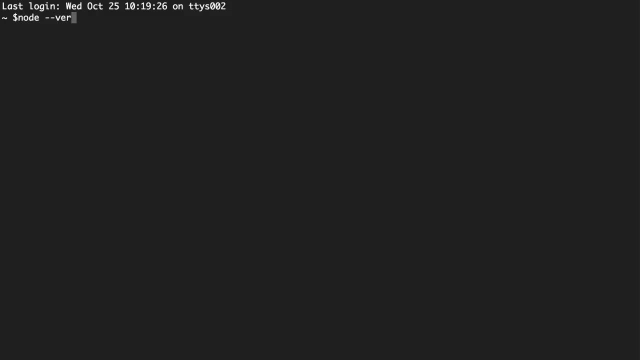 So run node space dash dash version. You can see on this machine I'm running Node. on my machine I'm running Node version 6.10.3.. This is an earlier version of Node. The latest stable version is version 8.. Now on your machine, chances are you may not have Node or you might have an earlier. 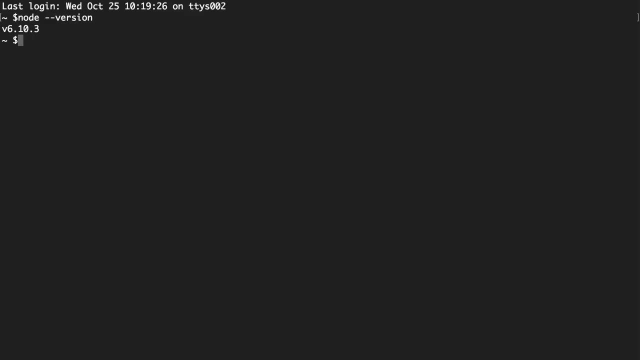 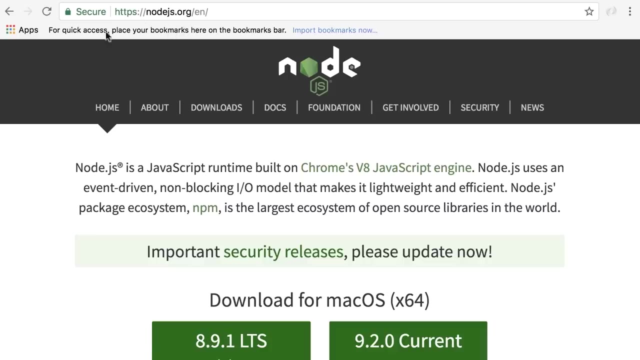 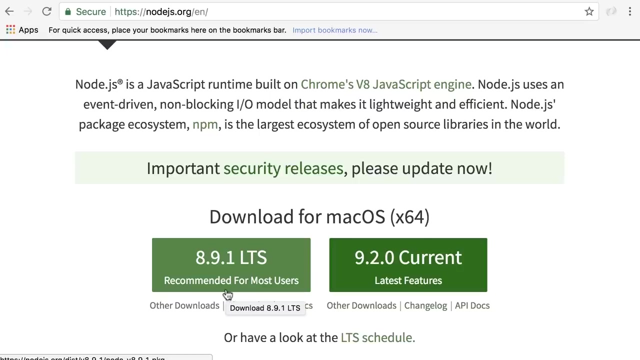 version. Either way, I want you to install the latest version of Node. So open up your browser and head over to nodejsorg On this homepage. you can see we have two versions for Node. One is the latest stable version, which is recombined. 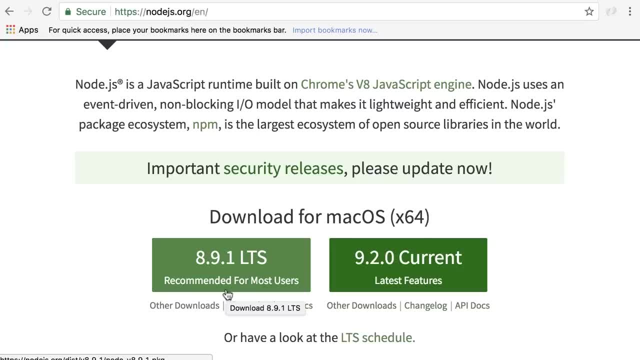 For most users at the time of recording this video, that's version 8.9.1.. And there's always a newer version which is experimental and it might not be stable, So I want you to install the latest stable version. Also, take into account that in the future when you're watching this video. 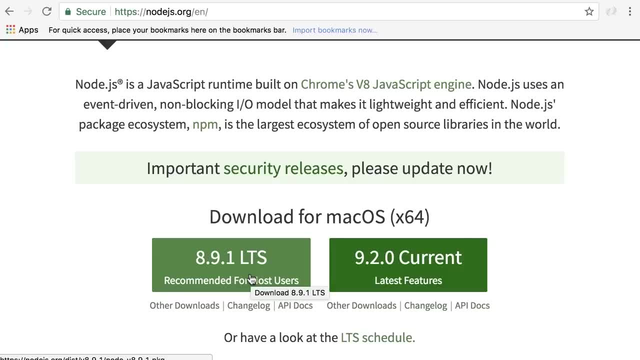 chances are, the latest stable version might be newer. If you're worried that this course is going to get outdated, don't worry, because in this course we're going to focus on the fundamentals. So I'm going to work with the core modules of Node. These core modules are stable. They have been there for a long time. 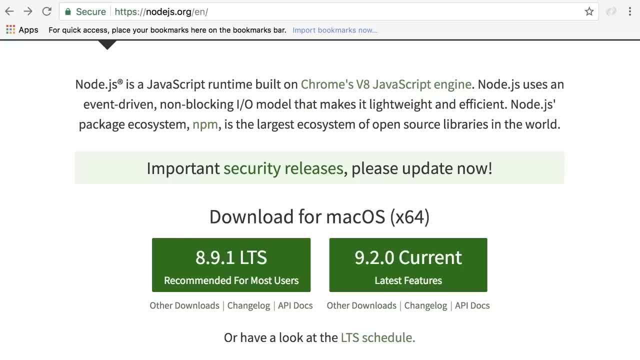 So the code that we're going to write in this course will continue to work with the future versions of Node. Once you master the fundamentals, you can always learn about the new features that come in every version by looking at the changelog, So let's not worry about the fancy new features in. 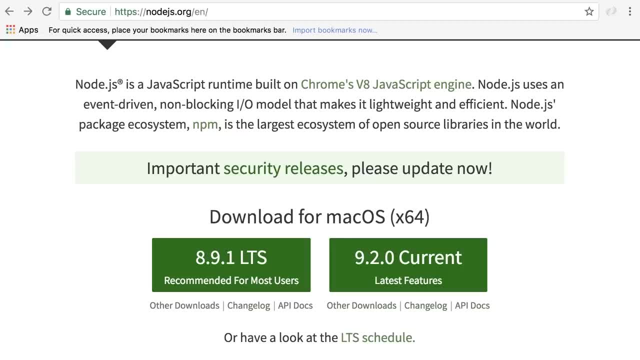 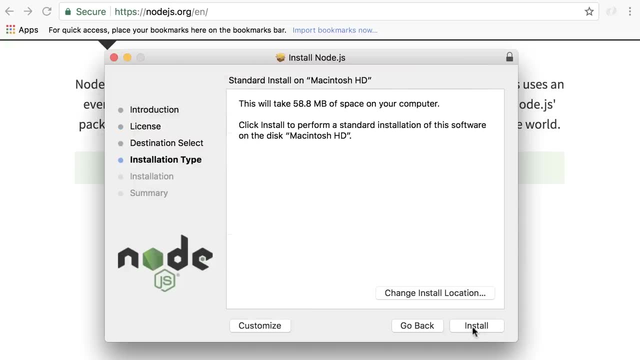 Node and focus on the fundamentals. So let's go ahead and install the latest stable version. You can see here we have a package, We run it. It's an installer. Take a look, Very simple: Just continue, continue, continue, install. We need to enter our password. 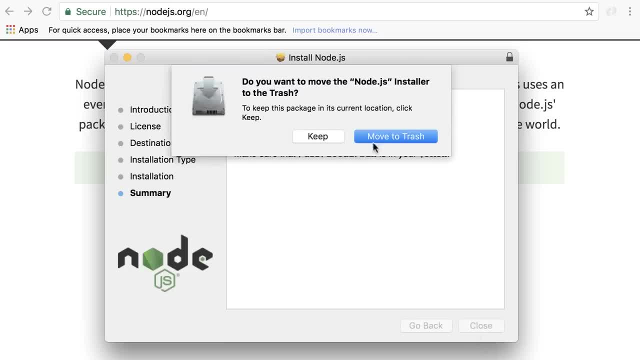 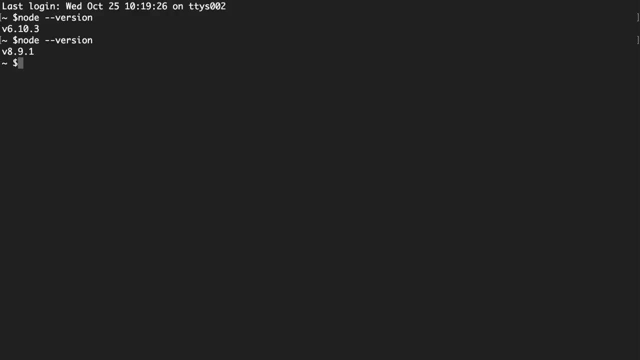 And the installation is complete. It took only a few seconds. So now back in the terminal. let's run node dash dash version one more time. You can see I upgraded my node to version 8.9.1.. Next we're going to build our first node application. 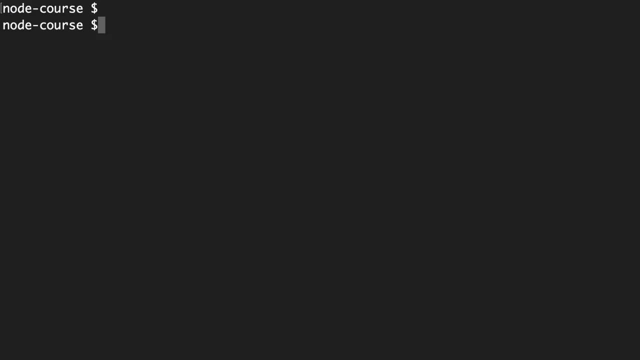 Now we're ready to build our first node application, So I'm going to create a new folder, Call it FirstApp. Let's go to this folder Now. I'm going to open this folder inside a Visual Studio, which is my preferred code editor, So code: 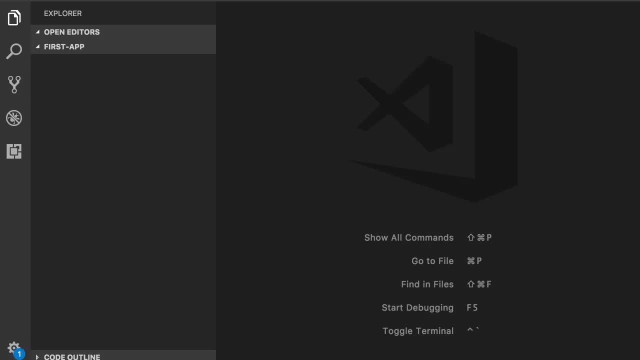 period. So this is Visual Studio Code or VS Code. It's a free, powerful editor, but you can use any editors that you prefer. You can use Sublime, you can use Atom or any other editors. So here in this folder, I'm going to add a new file: Appjs. 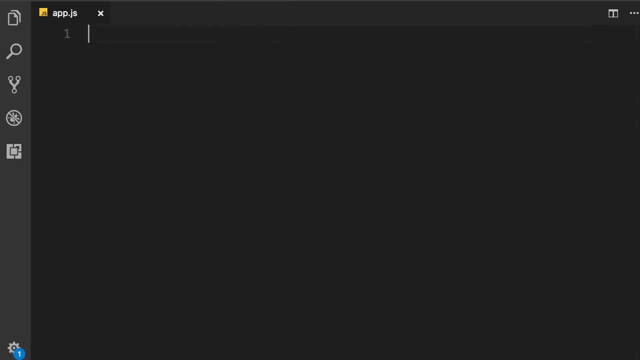 In this file we can write regular JavaScript, Just like the JavaScript that we write for the browsers. So I'm going to define a function, say hello, that takes a parameter name and simply logs a message on the console- So hello plus name. And then we can call this function like this: 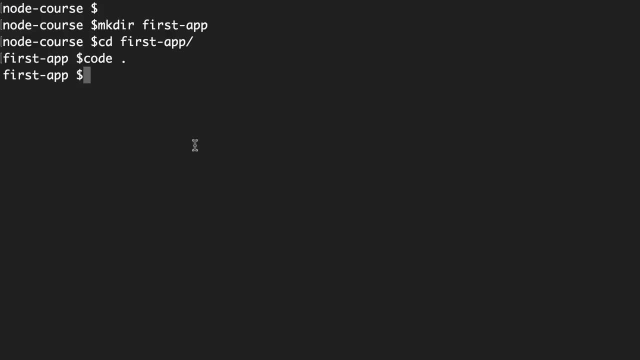 Mosh. Now to execute this code, we're going to go back to the terminal and run node and pass the name of the file as an argument. So appjs. So node, as I told you before, is a C++ program. It includes Chrome's V8. 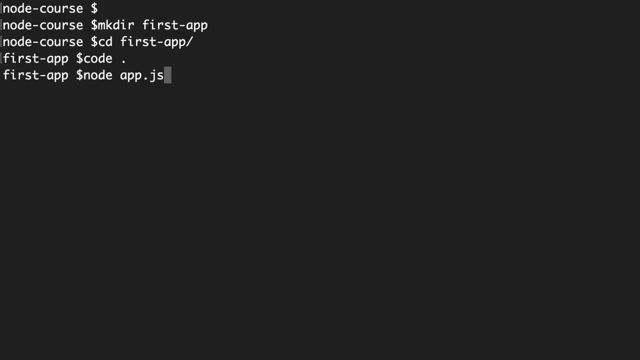 JavaScript engine. So this appjs file that we're going to pass to node Node is going to give it to V8 for execution. So you can see we got hello Mosh on the console. Now let me show you something. So, back in VS Code, I'm going to temporarily. 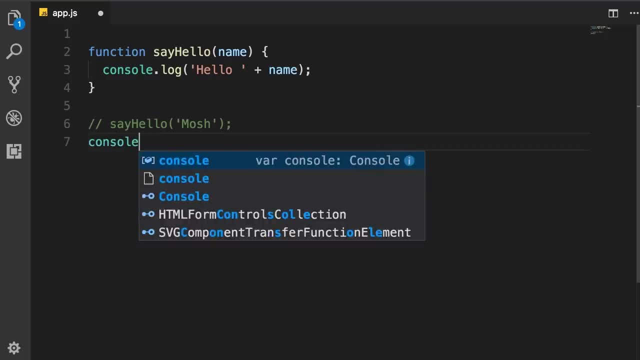 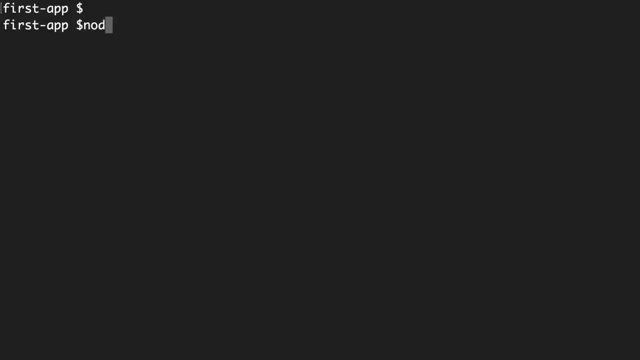 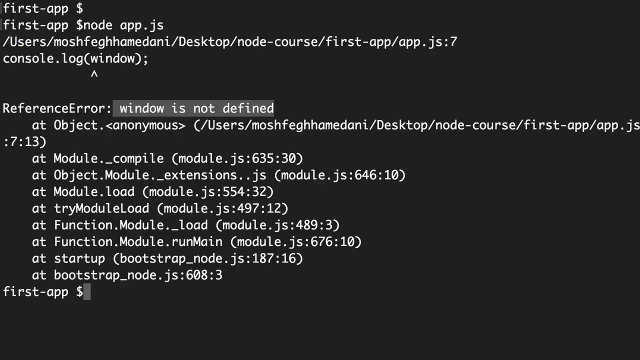 comment out this line and do a consolelog of window. Let's see what happens. So back in the terminal, let's run node appjs. We got an exception: Window is not defined. So, as I told you before, in node we don't have the window or document objects. 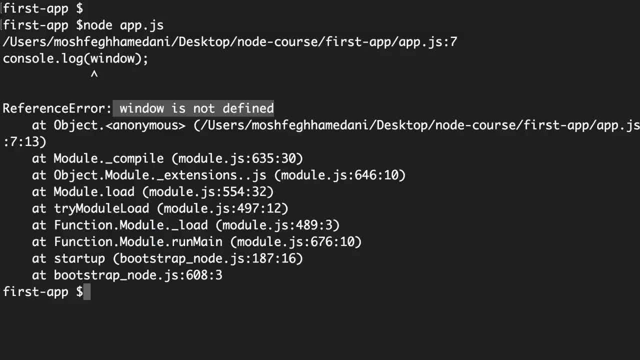 These are part of the runtime environment that we get with browsers In node. we have other objects to work with files, with the operating system, with the network and so on, And that's what you're going to learn about in the next section. 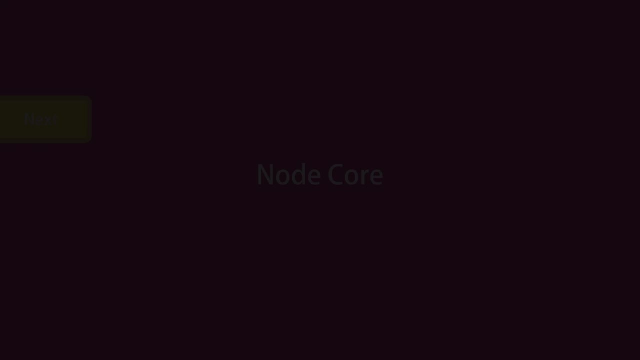 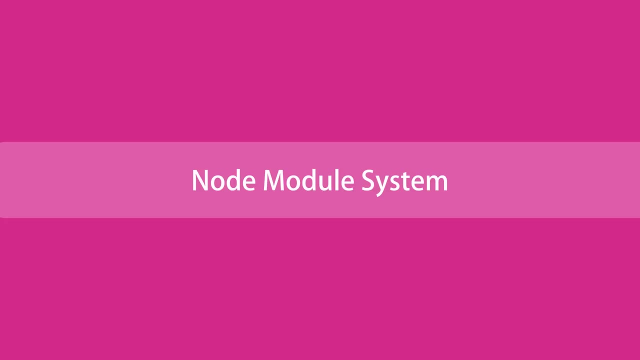 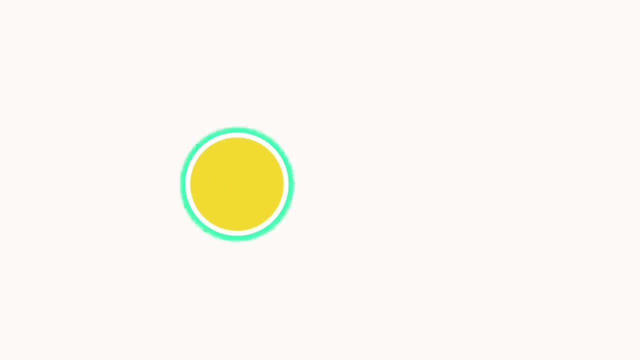 Enjoy this section and thank you for watching. In this section we're going to look at the module system in node. You will learn what modules are, why we need them and how they work. Throughout this section, we'll explore a few of the modules built into the core of node, such as operating system. 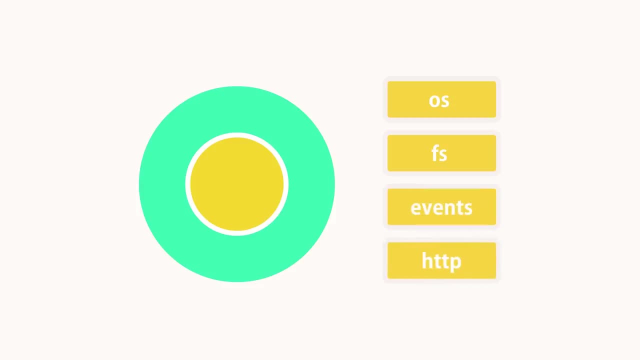 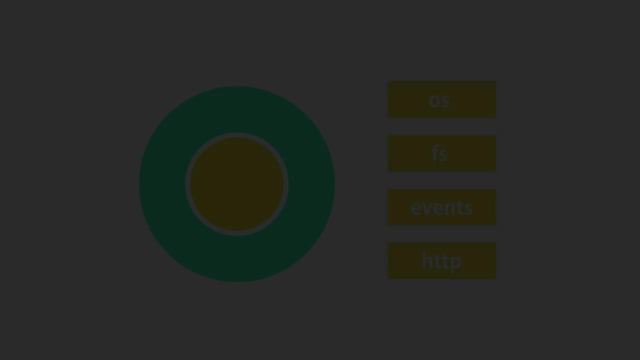 file system events and HTTP. You will also learn how to create your own modules. Let's get started. So in the last section, we use this consolelog function to lock something on the console. Now this console object is what we call a global object, So it's part of the 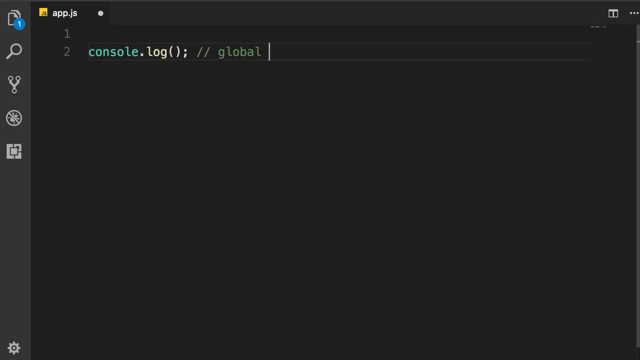 global scope, which means we can access it anywhere, in any files. We have a bunch of other objects and functions that are also globally available in node. For example, we have set timeout, which you have probably seen before. we use this to call a function after a delay, like one. 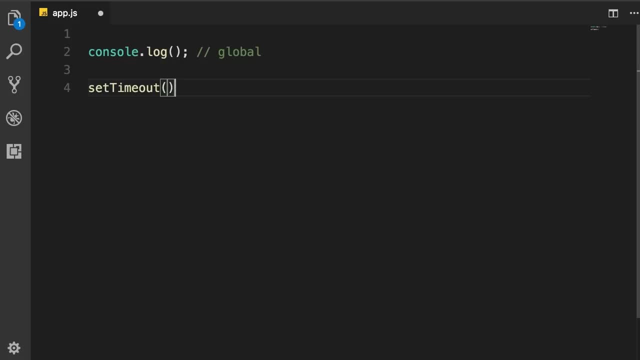 second, two second, whatever. so this is just part of the standard java script. we can use this on the client. we can use this inside of a browser or inside of node. We also have clear timeout. Similarly, we have set interval, which we used to repeatedly call a function after a given delay, to call the field interval. 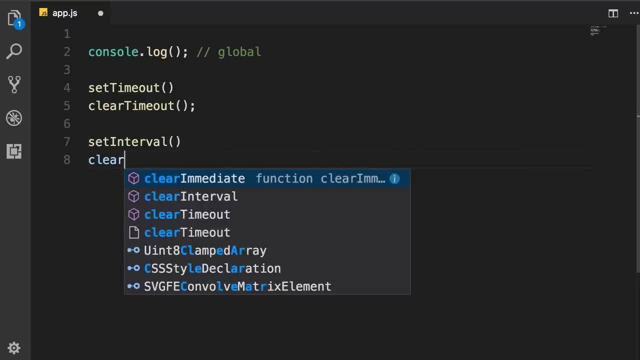 Similarly, we have set interval which we used to repeatedly call a function after a given delay, to call the field interval. We also have clear interval which we use to stop that function from being called repetitively. So these are the global objects in JavaScript, now in node. 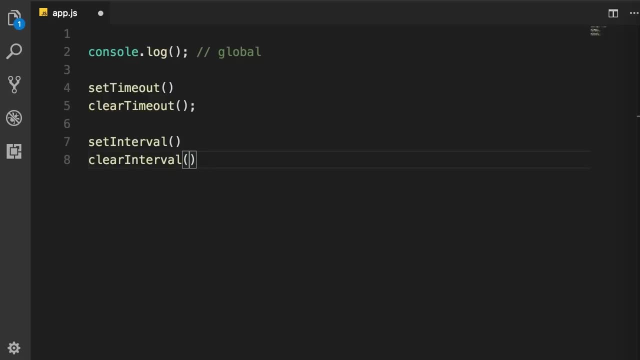 We have a couple other global objects that you're going to learn about later in this section. Now in browsers we have this window object that represents our global scope. So all the variables and functions that are defined globally, we can access them via this window object. So we can call window that console that log, or simply just console that lock. 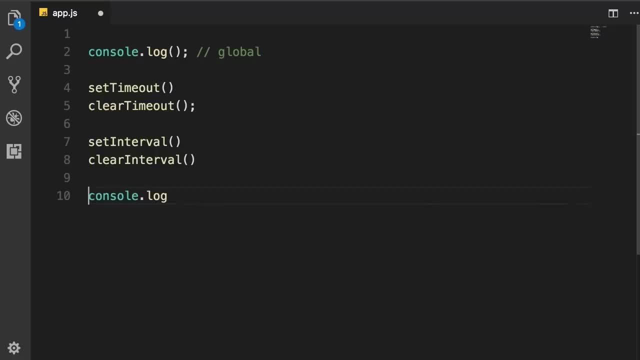 The JavaScript engine will prefix the statement with window, that console, that lock, because that's where this object is defined. Similarly, all these other functions you see here, They belong to the window object, so we can call window Set, timeout or call it directly. by the same token, when we declare a variable, 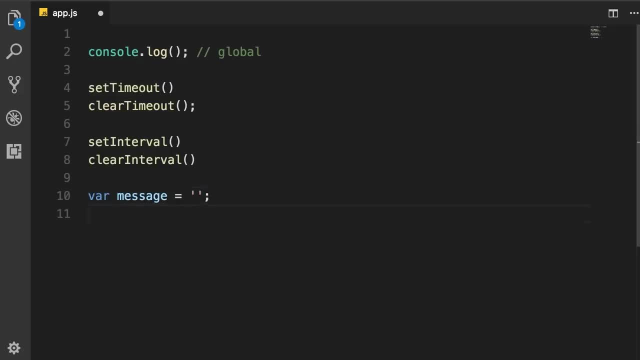 Let's say message, That variable is also available via the window object. Okay. however, in the last section I told you that in node We don't have this window object. Instead we have another object called global. So all these functions and objects we have here, we can access them via the global object. so we can do global. 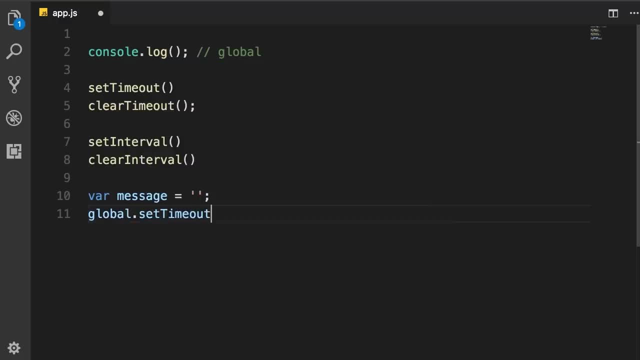 console log or global that set timeout and so on. Of course it's easier to use the shorthand instead of prefixing them with this global. But one thing you need to know about node is that these variables that we define here, They are not added to the global object. in other words, if we do a console dot log of 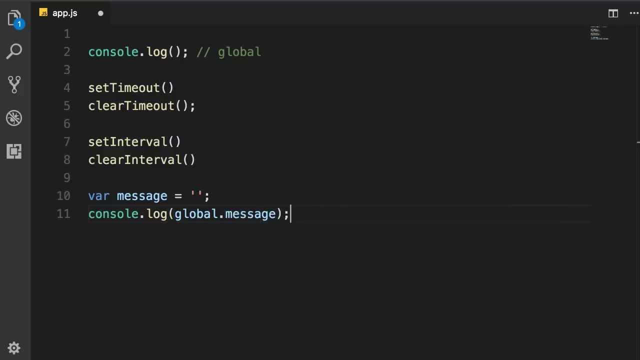 global. that message You're going to see undefined on the console. So let me show you: I'm gonna delete all the code here now back in the terminal and Let's run node app Js So we get undefined in the console. So, as you can see the variables and functions that we define here, they are not added to the global object. 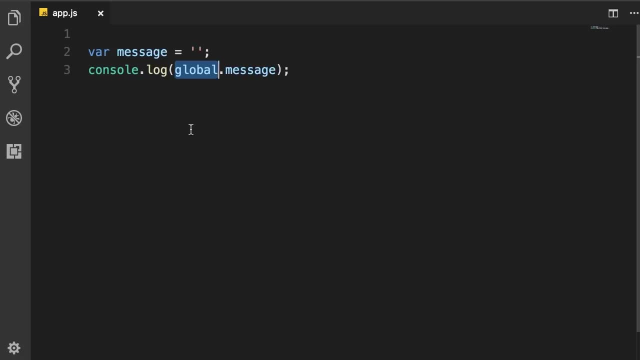 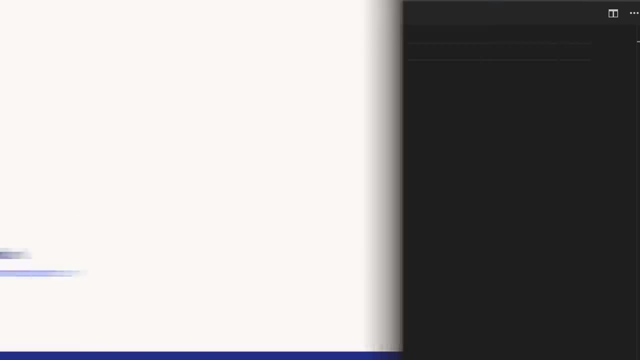 They're only scoped to this file, appjs, So they are not available outside of this file, and this is because nodes modular system that you're going to learn about in the next lecture, and So in the last section you'll learn that in the client-side JavaScript that we run inside of browsers. 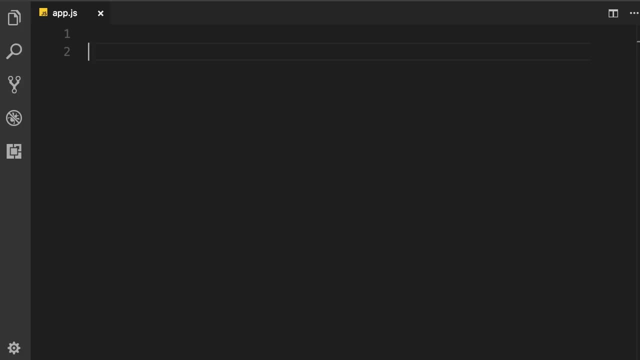 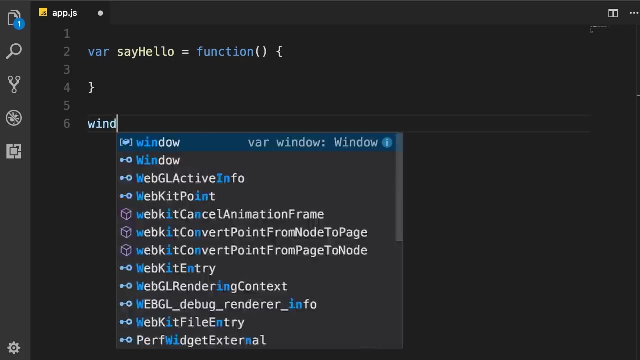 When we declare a variable or a function that is added to the global scope. For example, when we define a function like say hello, That function is added to the global scope and it's available via the window object. Now there is a problem with this behavior in a real world application. 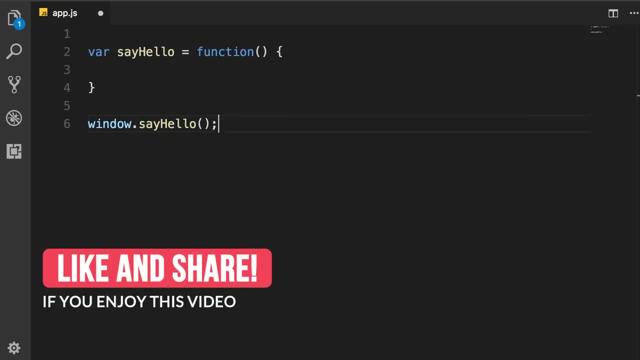 We often split our JavaScript code into multiple files, So it is possible that we have two files and in both these files We define this function. say hello with the exact same name, Because this function is added to the global scope when we define this function in another file. 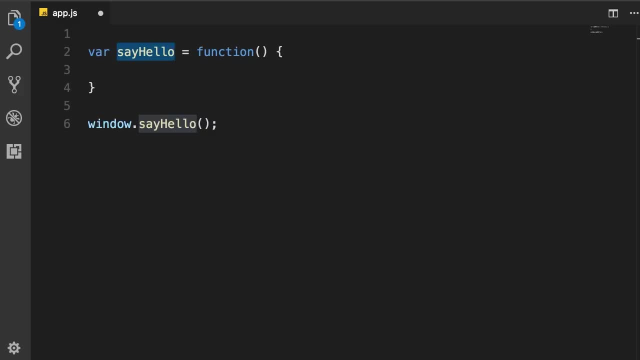 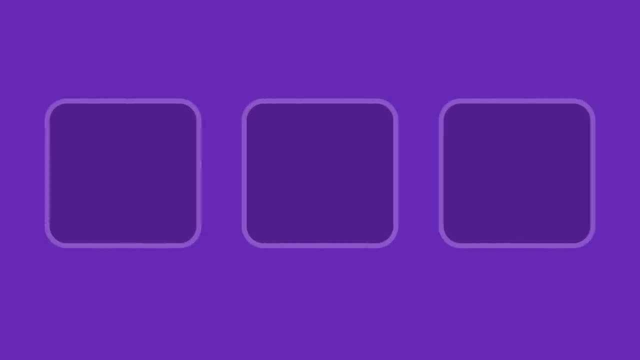 That new definition is going to overwrite the previous definition. So this is the problem with the global scope. so, in order to build reliable and maintainable applications, We should avoid defining variables and functions in the global scope. Instead, we need modularity. We need to create small building blocks or modules where we define our variables and functions. 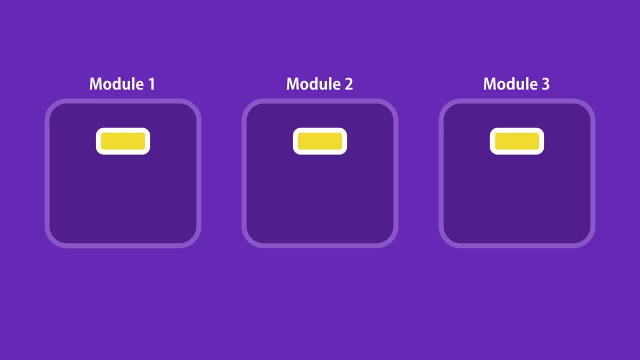 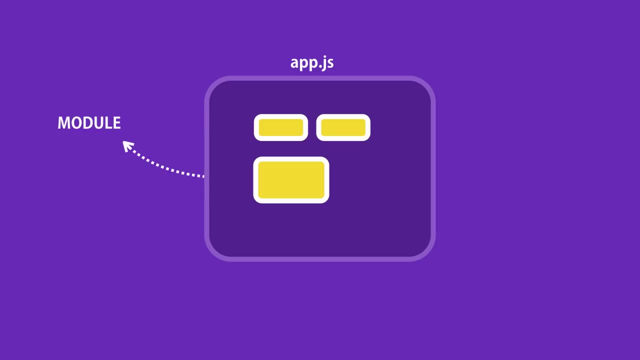 So two variables or two functions with the same name don't overwrite another variable or function defined somewhere else. They're encapsulated inside of that module. Now at the core of node we have this concept called module. so every file in a node application Is considered a module. the variables and functions were defined in that file or that module are scoped to that file in. 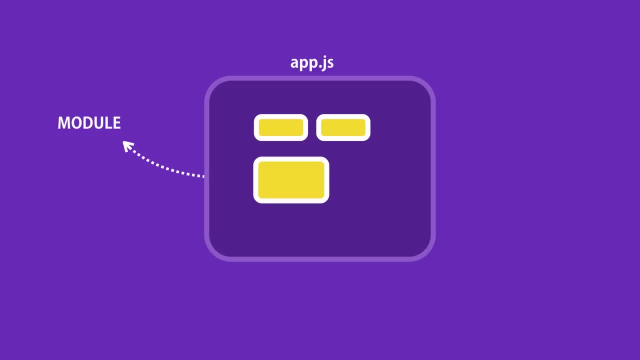 Object-oriented programming terms we say there are private. They are not available outside that container, outside that module. if you want to use a variable or a function defined in a module Outside that module, you need to explicitly Export it and make it public. and we're going to look at that in the next lecture. 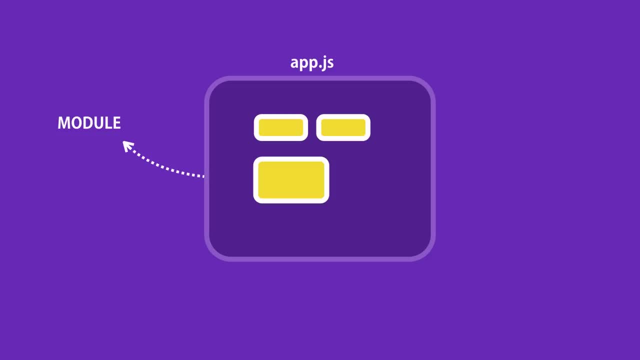 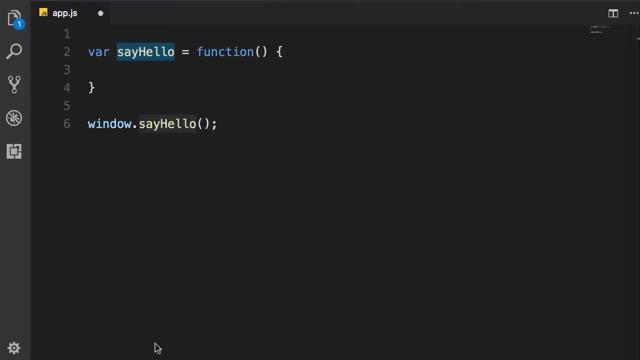 So what I want you to take away from this lecture is that every node Application has at least one file or one module which we call the main module. So in this case, this appjs is our main module. Now let me show you this module. 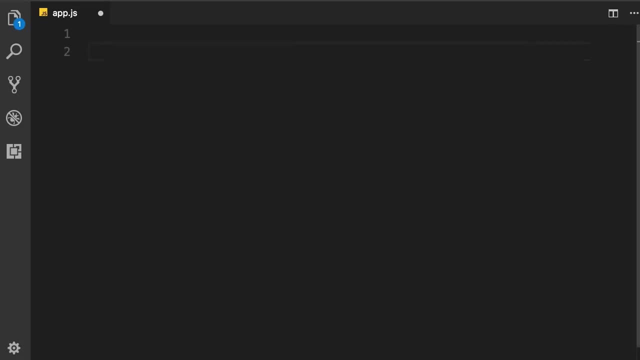 so I'm going to delete all this code here and Do a console log of module. Now this module object here may appear to be global, so you may think we can access it via the global object, like global that console. but Actually this is not a global object. It appears to be global but it's not global, and you will find out why very soon. 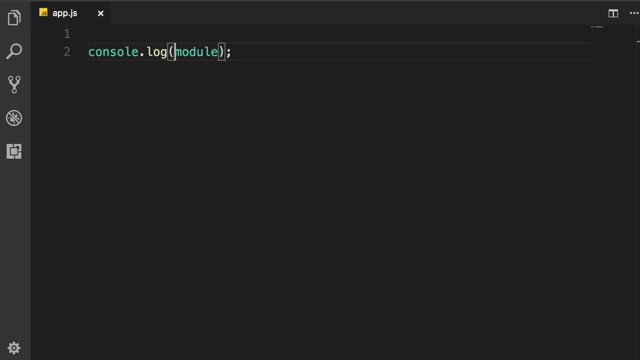 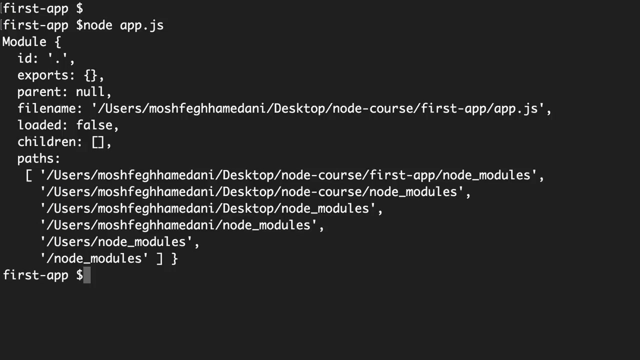 So let's just log this module object and see what we see in the console. back in the terminal node app the JS. So you can see we have an object module. It's a JSON object with these key value pairs. So we have ID. every module has an ID or a unique identifier. We have exports- parent. 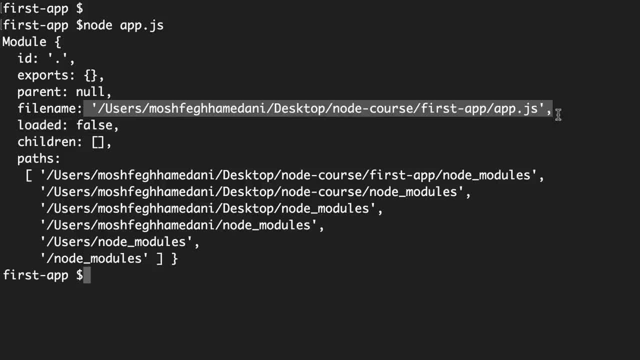 File name, which is the complete path to that file Loaded, which is a boolean that determines if this module is loaded or not. We have children and paths now for now, Don't worry about these properties. as we go through this section, You will gradually become familiar with these properties. 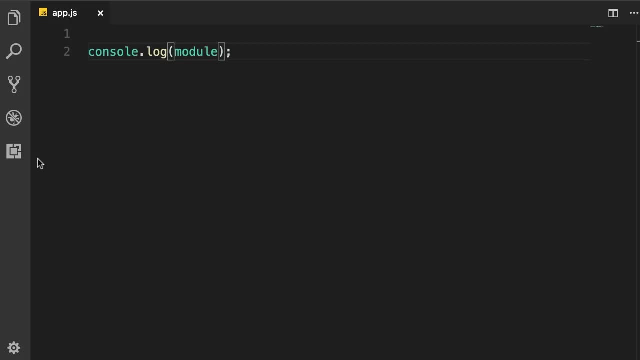 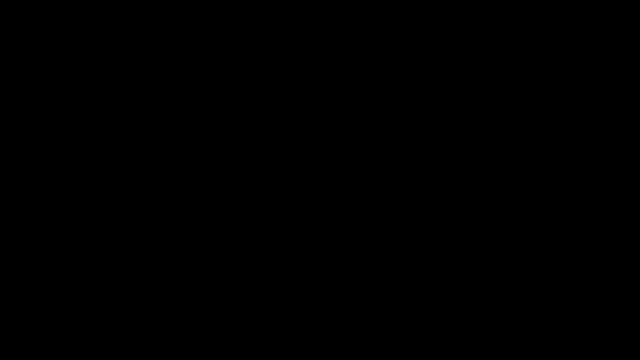 So in node every file is a module and the variables and functions defined in that file are scoped to that module. They are not available outside of that module. In the next lecture you're going to learn how to create and load a module. All right. now let's add a new module to this application. 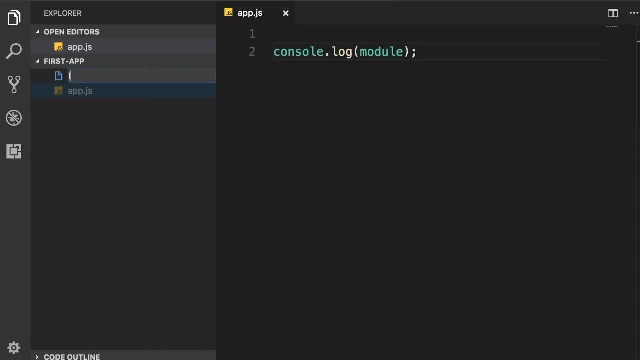 so I'm gonna add a new file: logger J s. let's imagine We're going to create a Module for login messages and we're going to reuse this module in various parts of this application or potentially in other applications. so logger JS Now in this module. let's imagine that we're going to use one of those remote logging services for logging our messages. 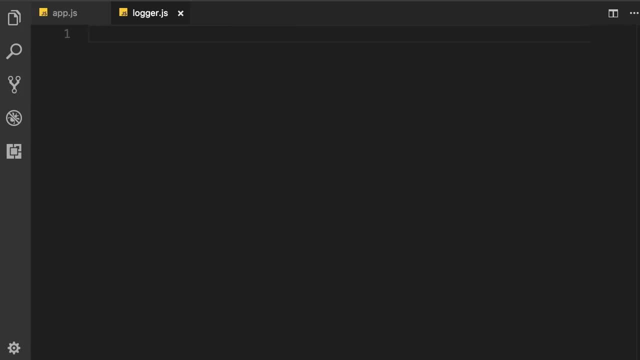 So there are websites out there that provide logging as a service. They give us a URL and we can send an HTTP request to that URL to log messages in the cloud. so here I'm gonna declare a variable like URL and Set it to something like this HTTP: 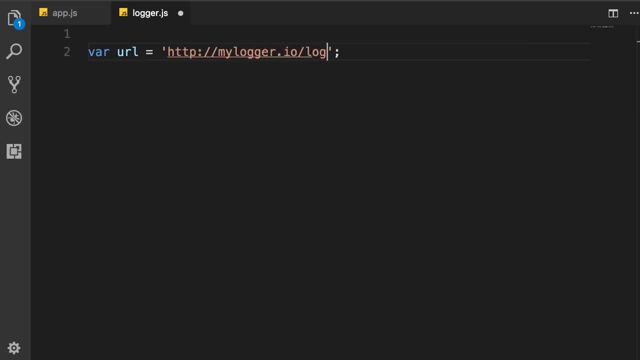 My logger, that IO slash log, and of course I'm making this up. It may not be a true service out there. Well, let's imagine, in this implementation, We're going to send an HTTP request to this endpoint, to this URL. Now we also need a function. 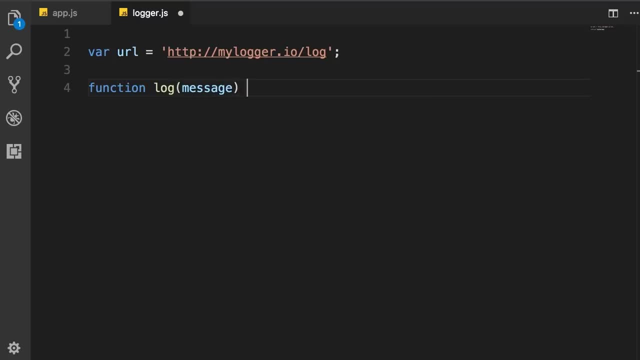 Called log. that takes a message and In this function we're going to send an HTTP request. however, To keep things simple here We just want to focus on the modularity. We don't want to get distracted with all the details of sending HTTP requests, So for now I just want to log this message on the console. So console. 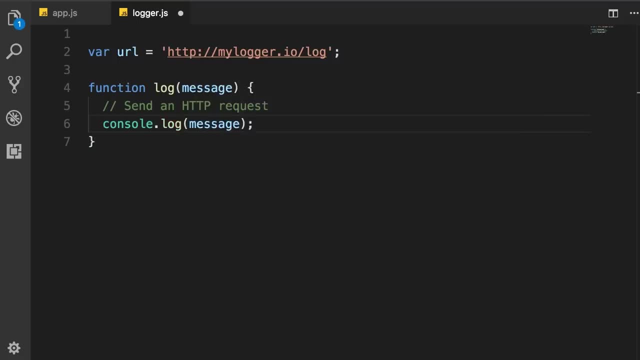 log message. Okay now, This variable and this log function, They're both scope to this module. They're private, They are not visible from the outside. however, in appjs, Which is our main module, We want to use this logger module, So We should be able to access this log function. We should be able to call it from the app module. 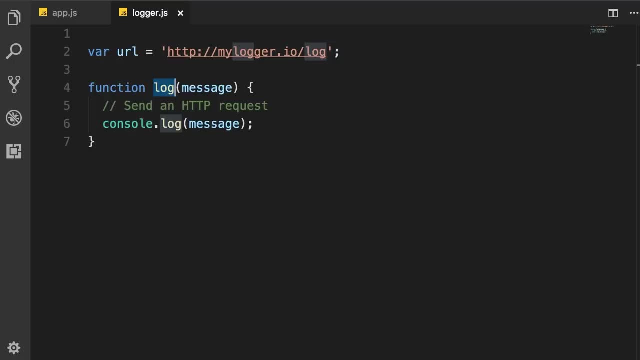 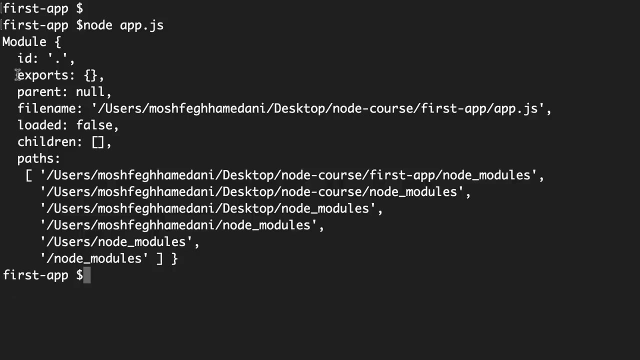 So we need to make this public. We need to make it visible from the outside. Now, in the last lecture you saw this module object. one of the properties we have here is exports. you can see this property is set to an empty object. anything that we add to this object will be. 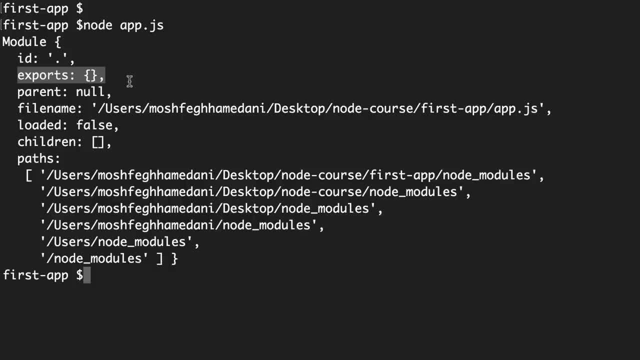 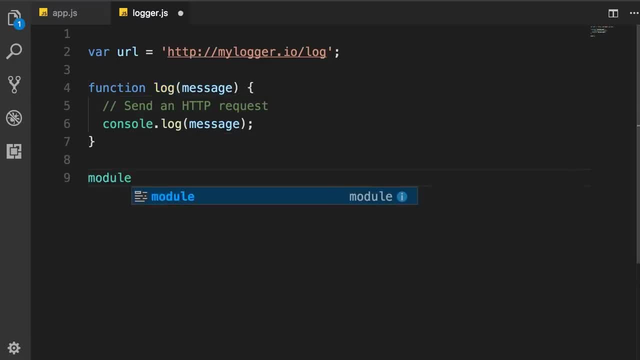 Exported from this module and it will be available outside of this module. So back in our logger module I'm gonna set module dot exports, dot log. so I'm adding a method called log to this exports object and Simply setting it to this log function We have defined here. 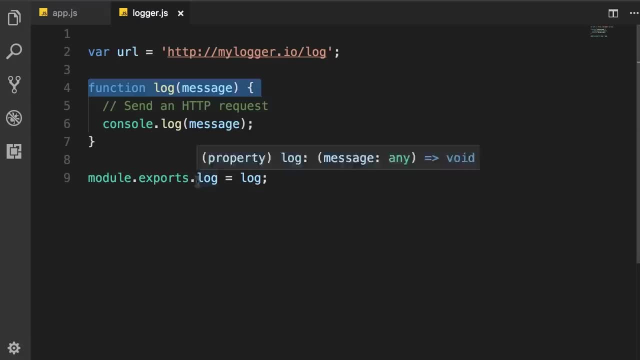 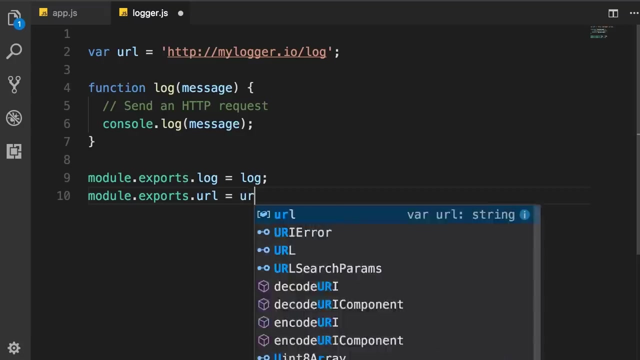 Okay, In other words, the object that we're exporting here has a single method Called log. now, similarly, if you want to export this URL, we could do something like this: so, module that exports that URL, we set it to URL and, Of course, we could change the name that is exported to the outside. For example, internally, we may call this variable URL. 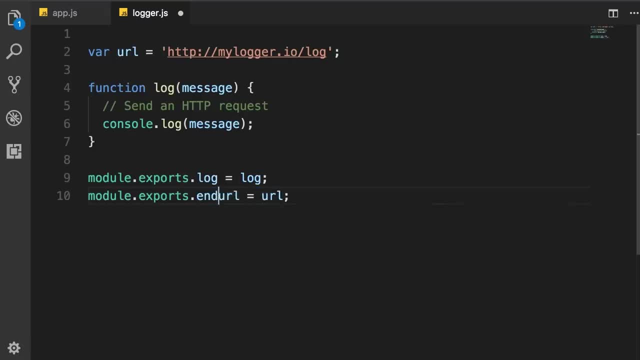 But when we export it, we may call it Endpoint. Okay now, In this case we don't need to export this URL variable because this is purely Implementation detail. so in real world applications, every module might have several variables and functions. We only want to export a subset of these members to the outside because we want to keep this module easy to use. 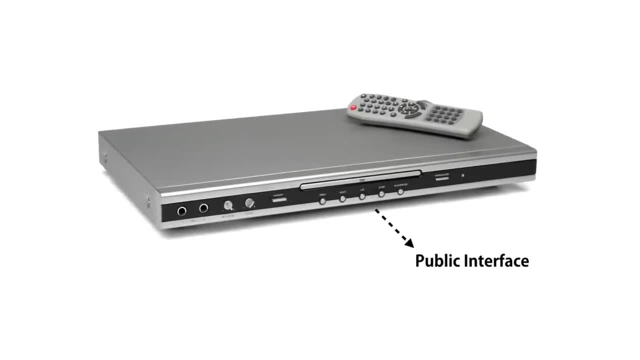 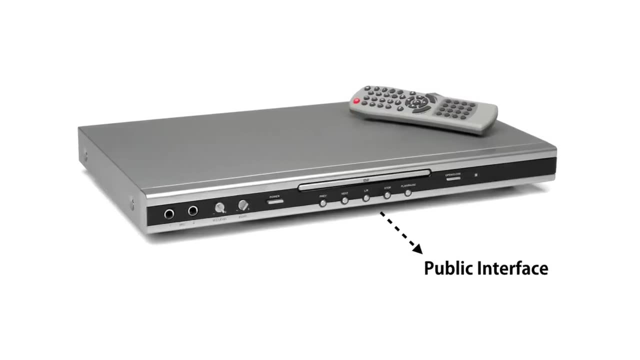 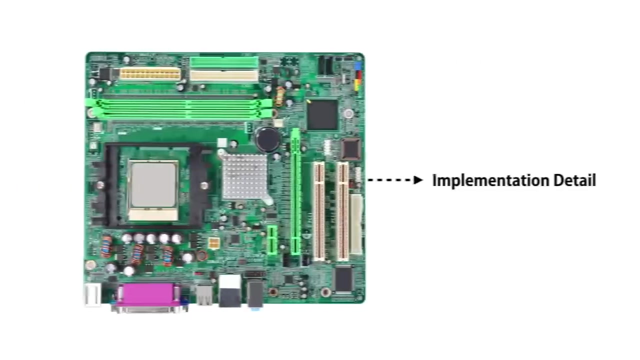 Let me give you a metaphor. think of a DVD player. a DVD player has a few buttons on the outside, and these are the buttons or objects that we interact with. So these objects represent the public interface of a DVD player. Okay, but inside the box there are lots of other objects or complex objects. 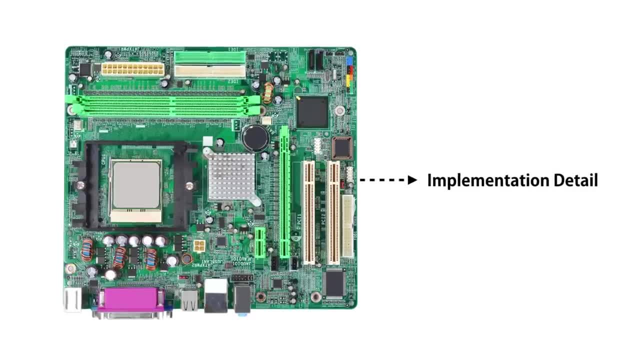 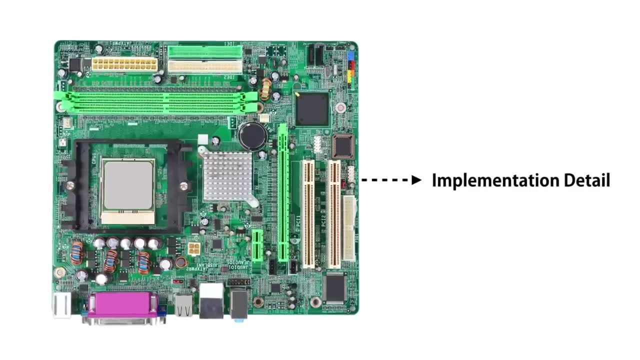 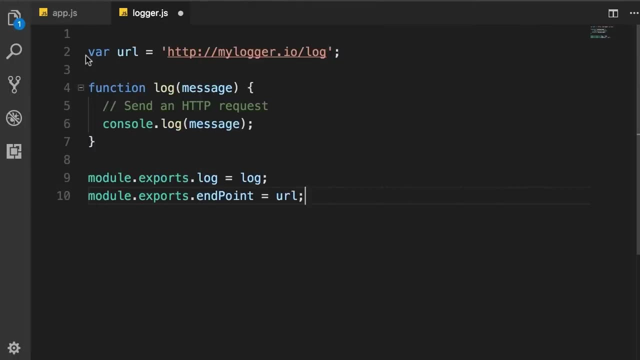 We don't need to know anything about these objects, their implementation detail and they can change significantly from one model to another. But what we see on the outside is almost stable or static across different models. so in our logger module this URL is Implementation detail. other modules don't need to know anything about this. 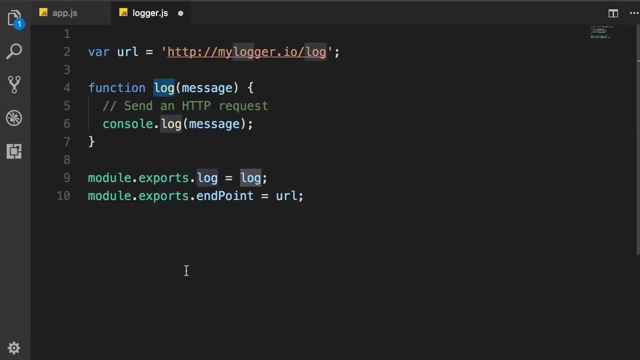 They only need to call the log function. so we export this, make it public, but keep the URL private. So I'm gonna delete this last line. Okay, so we are done with our logger module. Now We need to load this module and use it inside appjs. 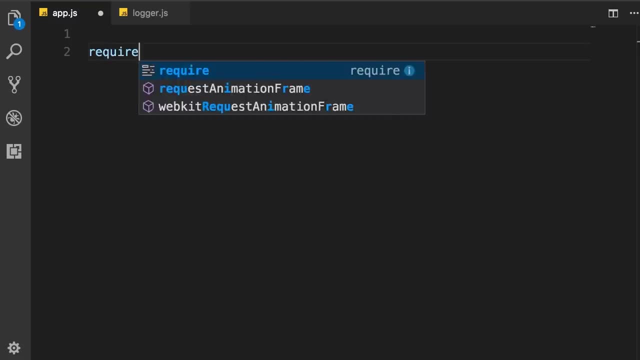 To load a module, we use a require Function. this is one of the functions in node. We don't have this in browsers. this function takes one argument and that's the name or path of the target module We want to load. So Here we want to load the logger module now. 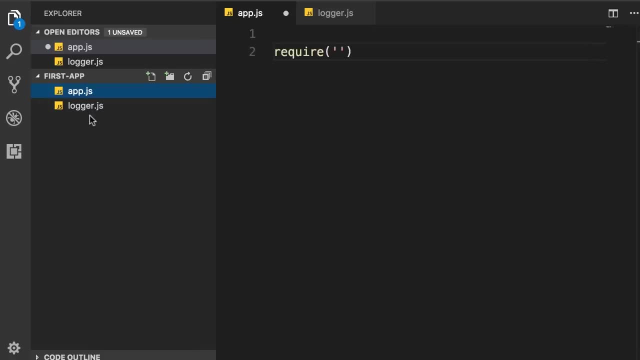 We can see both the app module and logger module are in the same folder. so we use period-slash to indicate the current folder and then we add the name of our module, that is, logger a. or we can make it shorter and just use logger, because node assumes this is a javascript file. 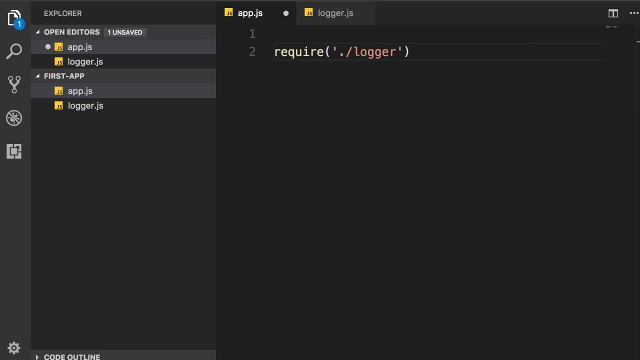 and it automatically adds the js extension. now if this logger was in a subfolder, we could add that subfolder here. or if it was in the parent folder, we could use dot dot slash. so here we're using the relative path to the target module. in this case that module is in the same folder. 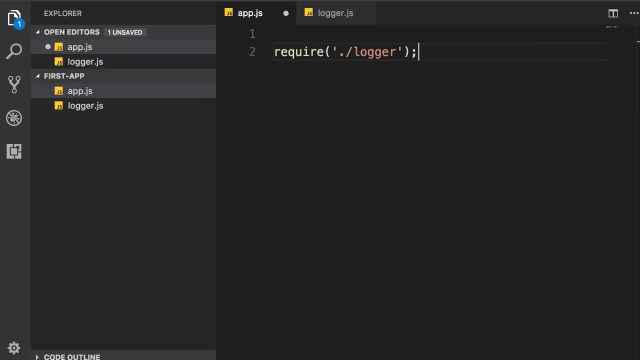 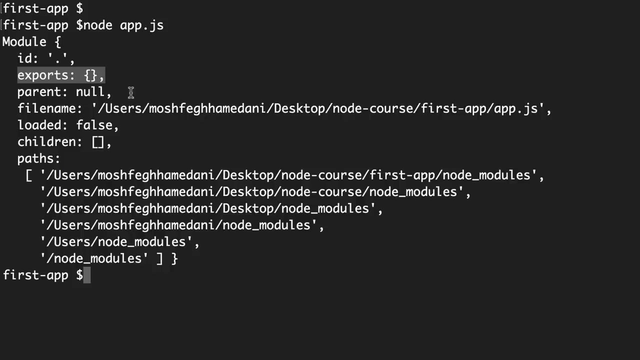 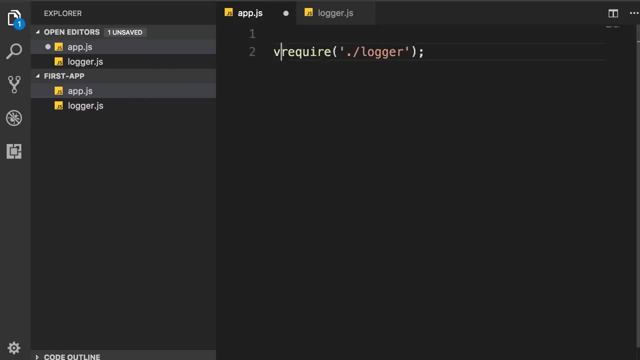 now, this require function returns the object that is exported from this target module. so this exports object here. this is what we get when we call the require function. let me show you. so i'm going to declare a variable, call it logger the name of the module and set it to the return. 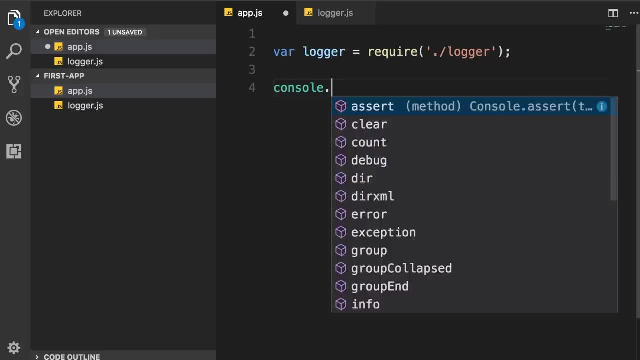 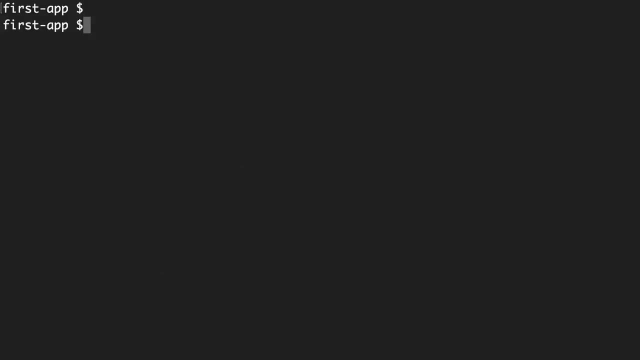 value of the require function. now let's log this logger and see what we get. so node appjs. look, we get an object. this object has a single method called log. you can see that's a function. so we can call this function or this method in appjs. so back here we call logger. 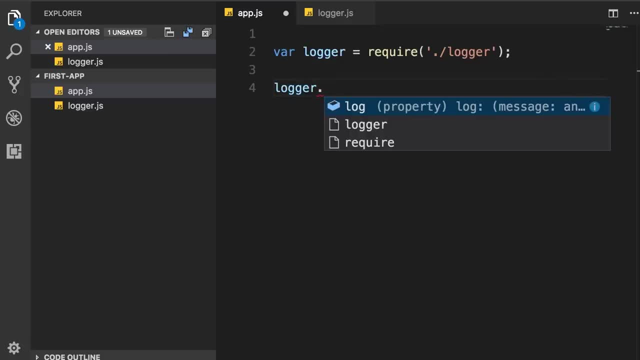 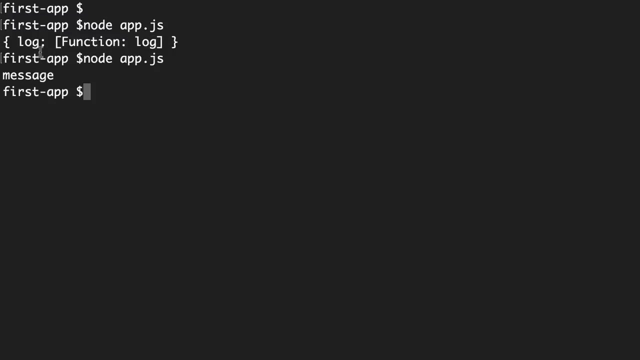 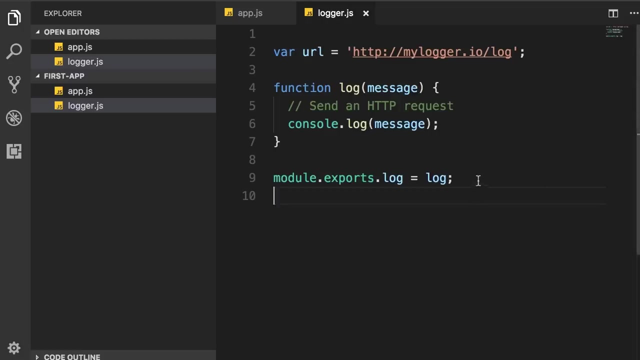 dot and look here we have intellisense in vs code. so we call log and pass a message. now back in terminal, let's run this app and we get message on the console. so this is how we work with modules in node: when we define a module, we export one or more members and then to load the 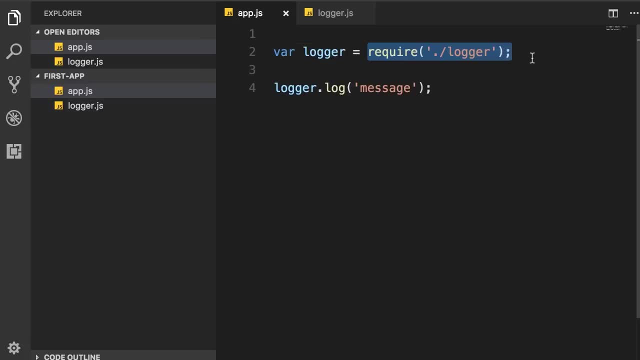 module, we use the require function. now, in the recent versions of javascript, we have the ability to define constants. so, as a best practice when loading a module using the require function, it's better to store the result in a constant like this. the reason for this is because we don't want to accidentally 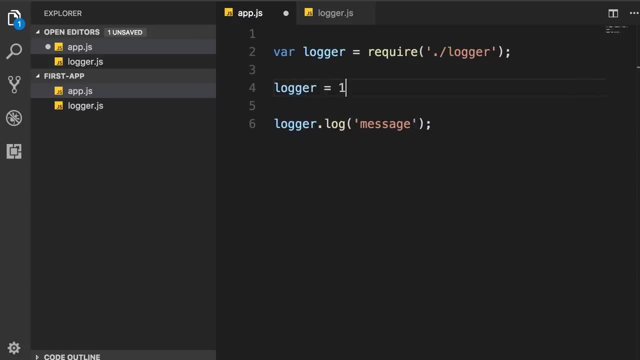 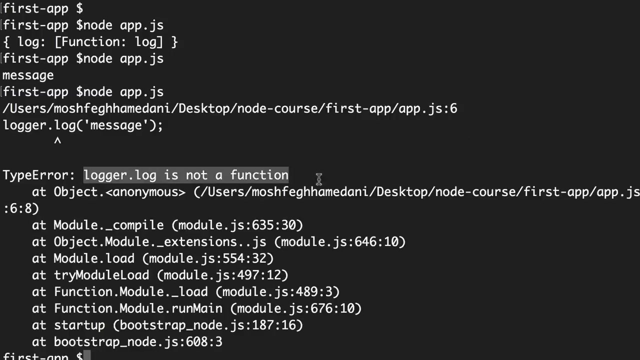 overwrite the value of logger like this here. if we set this to one, then when we call the log method, we're going to get an exception. let me show you so one more time. look, we've got. loggerlog is not a function now. in contrast, if we define this as a constant. 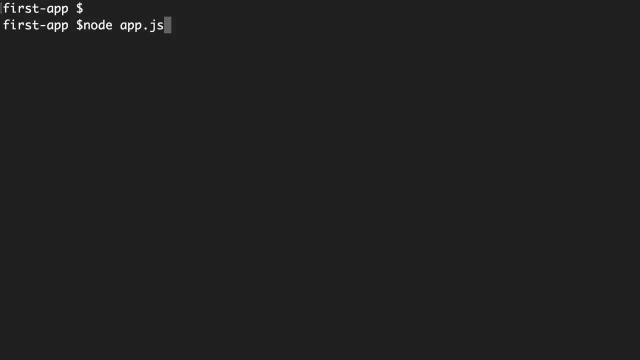 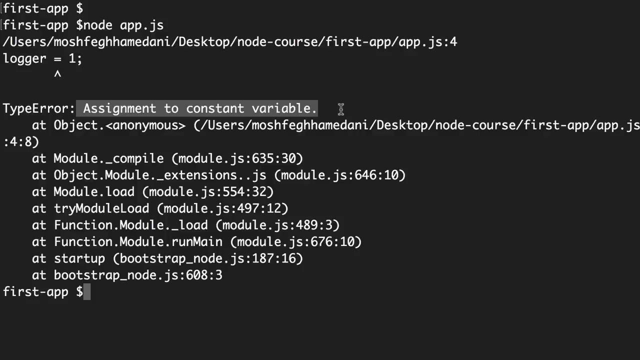 now back in the terminal. let's run this program one more time. look, we got a different kind of error: assignment to constant variable. now there are tools out there that check our javascript code for errors like that. so by using these constructs properly, we can prevent these errors from happening at runtime. 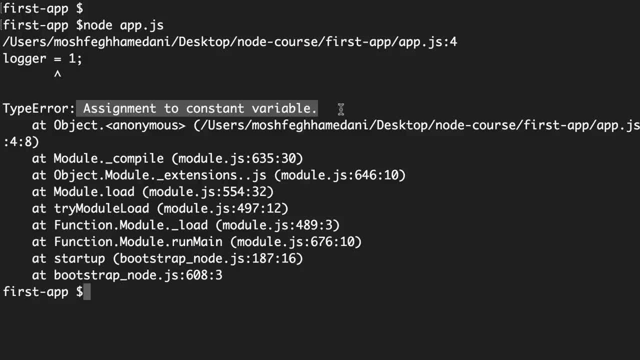 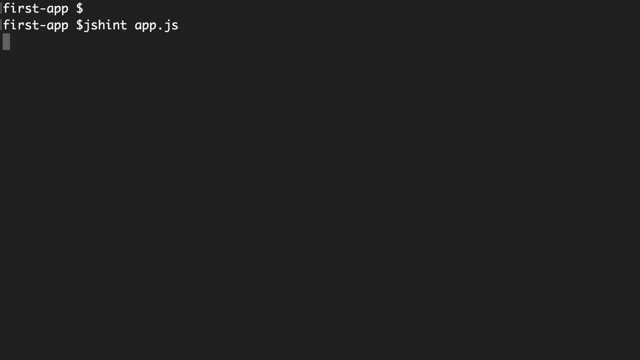 one of these popular tools is jshint. if you have never used it before, don't worry, i'm just going to show you a quick demo. so if you run jshint appjs, we get this error attempting to overwrite logger, which is a constant. so with tools like jshint, we can scan all. 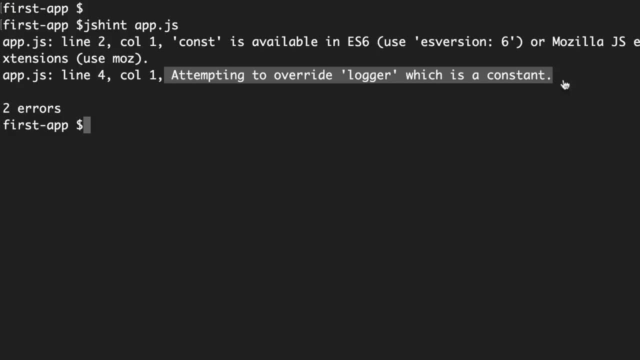 our javascript code for errors like that. so that's the benefit of using a constant as opposed to a variable here. if you accidentally reset this object, then we're going to get an error. instead of random fame variables, we need to자. let's make this goes to the localholesría, as we are high enough, so we canweias see this changes. 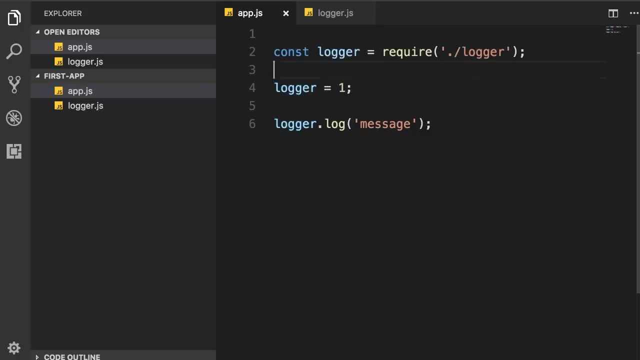 then we're going to win the time. use these files and 3 are not exactly at compile time instead of at runtime. okay, and one last thing before we finish this lecture. sometimes, instead of exporting an object from a module, you may want to export only a single function. 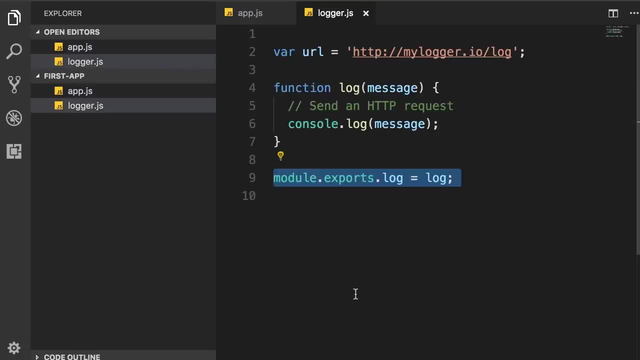 for example, here in our logger module, we don't necessarily need an object because we have a single method. an object would be useful if we had multiple methods or properties here. but in this case instead of exporting an object, we can export a single function, so we can reset this exports to. 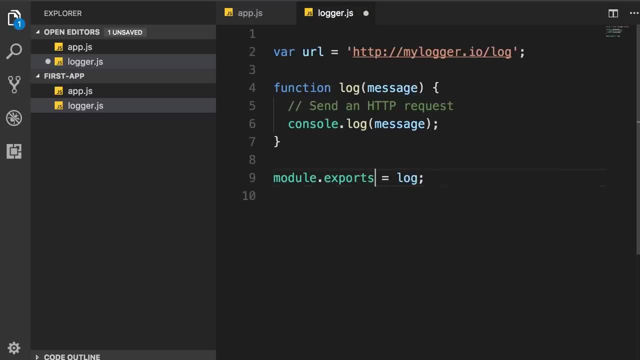 the log function. so initially it was an empty object, but we reset it to just a function. with that I can have J's. so logger is no longer an object, it's a function that we can call directly, like this: so logger, we call it an. give it an argument. Now, a better name for this function is: 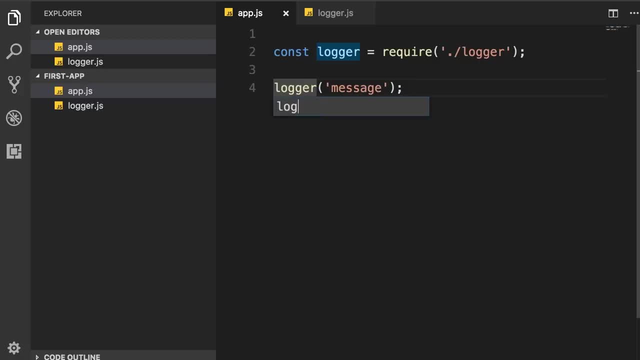 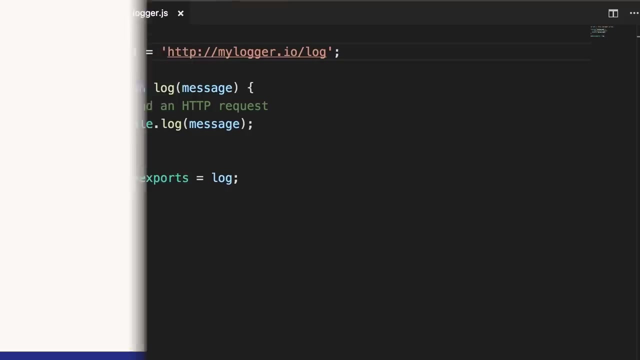 log. So I'm going to press F2 to rename this Log like this: Now back in terminal, let's run node appjs and we get the same result. So in your modules you can export a single function or an object. So now you know the variables and 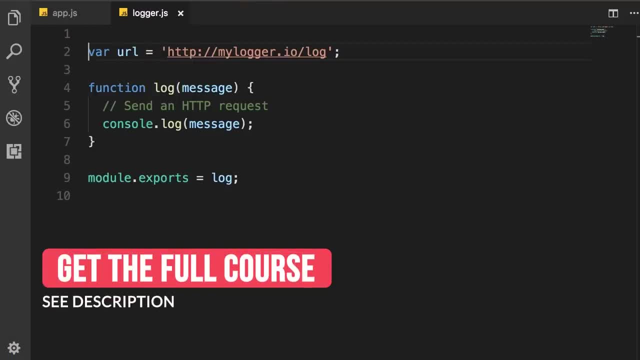 functions we define in a module are scoped to that module. They're private and not visible from the outside. But you might be wondering: how node does this? So let me show you. On the very first line of the loggerjs module, I'm going to create a syntactical 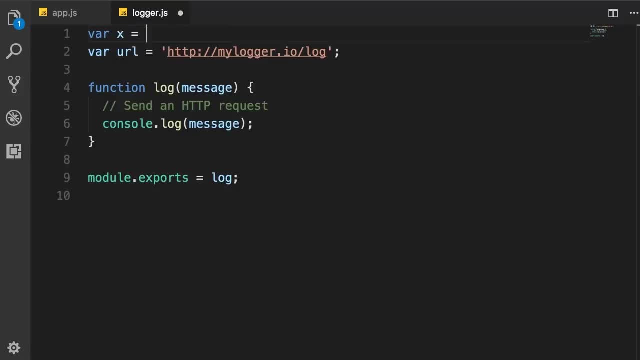 error. So define a variable x and set it to nothing like this. So make sure to write this code on the very first line. In other words, if you have a line break here and do this on the second line, you're not going to see what I'm going to show you now. So put this back. 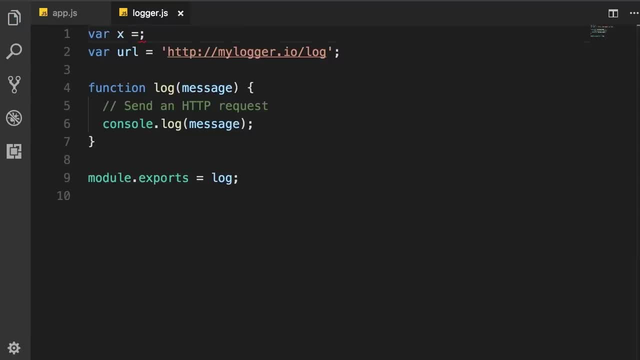 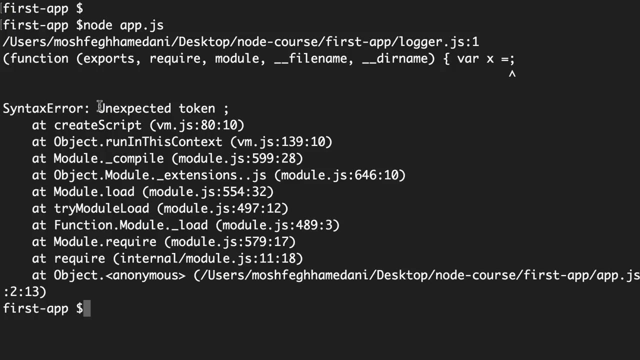 on the first line. Here we have a syntactical error. Now back in the terminal, let's run the application again. Okay, we got unexpected token semicolon. But look above this line. You see this function declaration. So this function has a few parameters. Exports require. 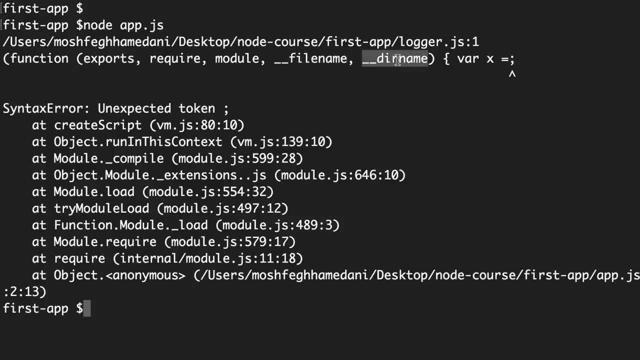 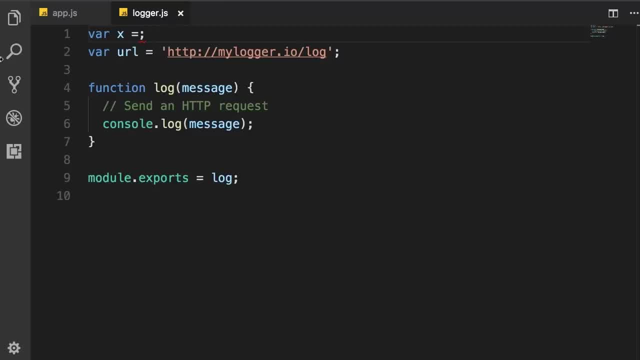 module, File name and their name. So let me copy this code here Now. basically, what happens under the hood is that node does not execute this code directly. It wraps it inside of a function And that's the function you saw. So at run time, our code. 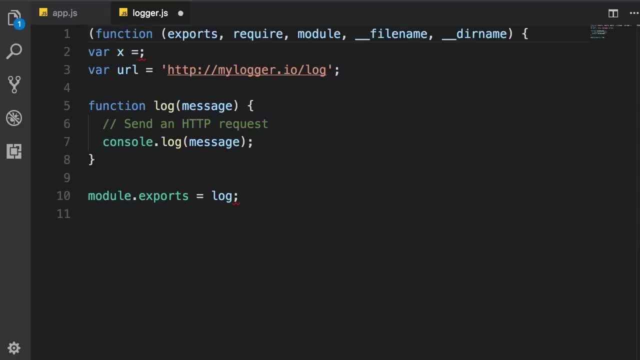 is going to be converted to something like this: So we have this function declaration. Here's the body of that function. Now for now, I'm going to remove this error here. So this is our code, And then we have the end of this function. 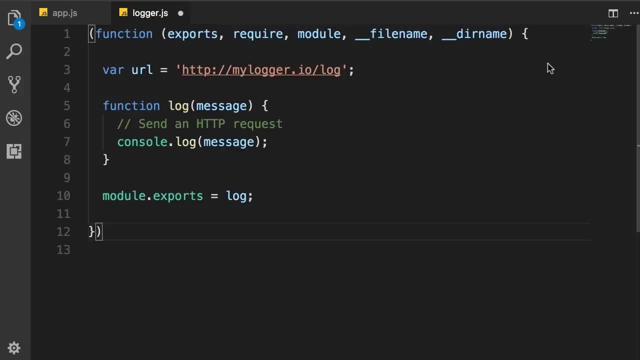 Now the actual code is slightly more complicated than this, But we don't want to get distracted with that complexity. If you're a more advanced JavaScript developer, you probably know this is an immediately invoked function expression or iffy. If you don't know that, don't worry. 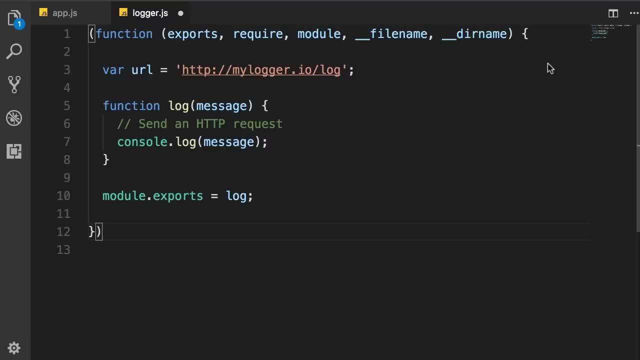 that's not really the scope of node. What I want you to take away here is that node does not execute this code. So if you don't know that, don't worry, that's not really the scope of node. What I want you to take away here is that node does not execute this code. 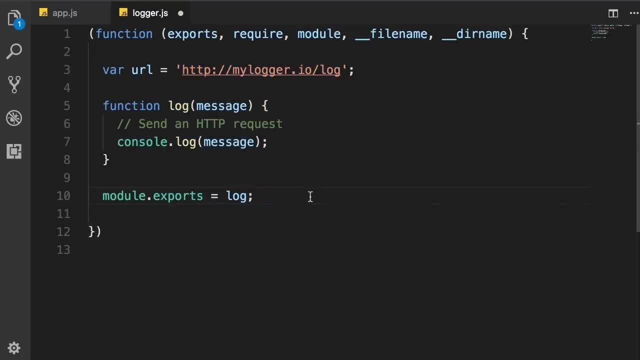 execute our code directly. It always wraps the code inside each module in something like this: Inside of a function. Now look at these arguments to this function. So you have seen the require function. I told you that this require function appears to be global, but actually it's not global, In fact. 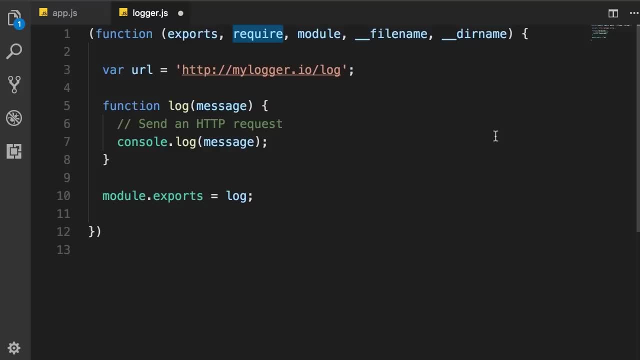 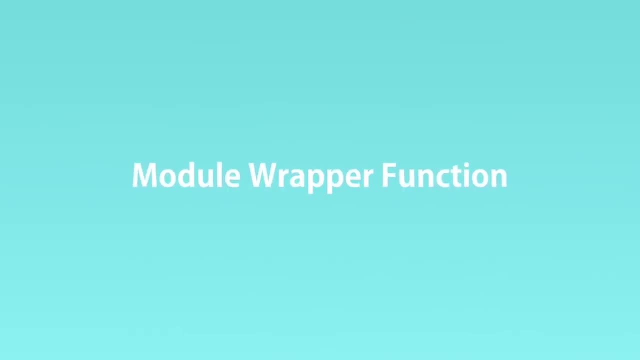 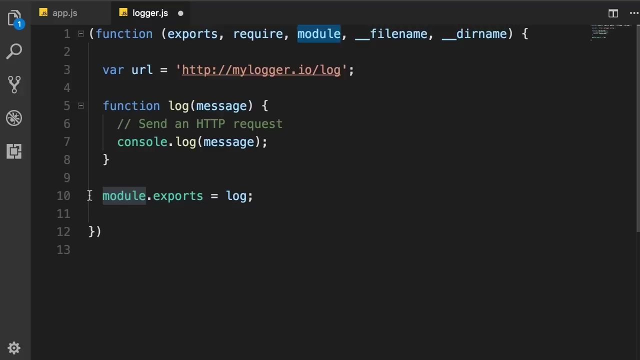 it's local to each module. So in every module, require is one of the arguments that is passed to this function. We call this function the module Wrapper function. So you have seen the require function. You have also seen module. That is what we're using. 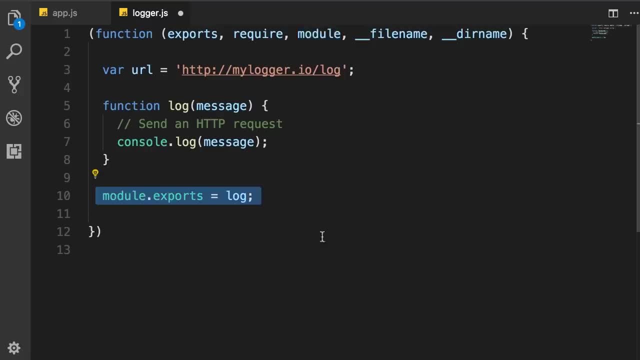 here. So we have moduleexports. We also have exports, which is a shortcut to moduleexports. So if you want to add a function to moduleexports object, you can either write moduleexportslog equals log or you can write exportslog equals log, But you cannot reset this exports. 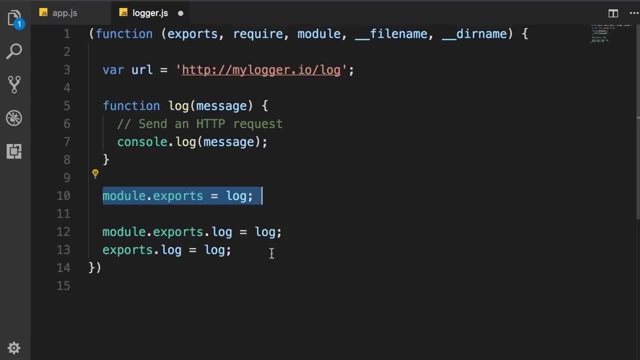 like what we did earlier. In other words, you cannot write exports equals log, Because this exports is a reference to moduleexports. You cannot change that reference. These are the first three arguments. We also have filename and dirname, which represent the name of this file. 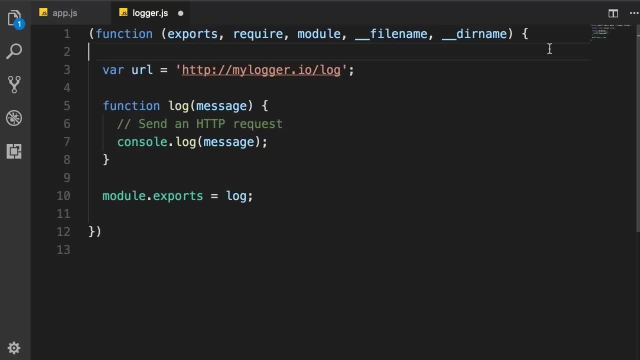 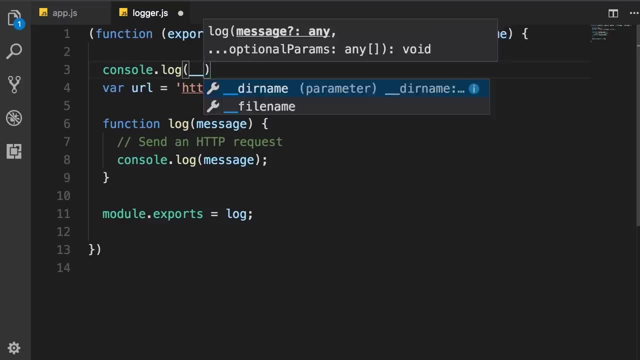 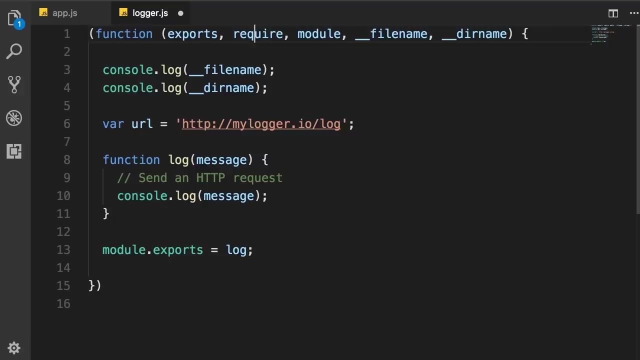 And the path. So let's have a quick look at these arguments On the top. I'm going to do a consolelog of underline- underline filename and also underline- underline dirname. Now we're not going to have this function, this module wrapper function. This was purely for demonstration, So I'm going to 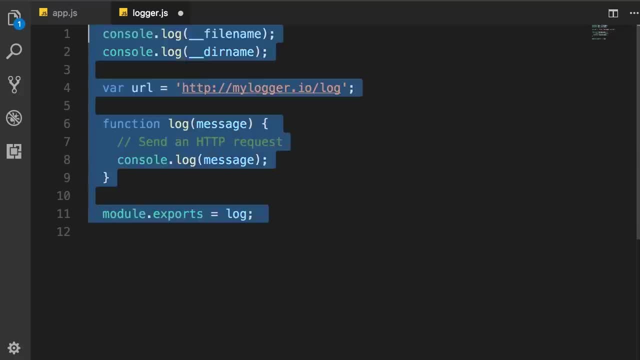 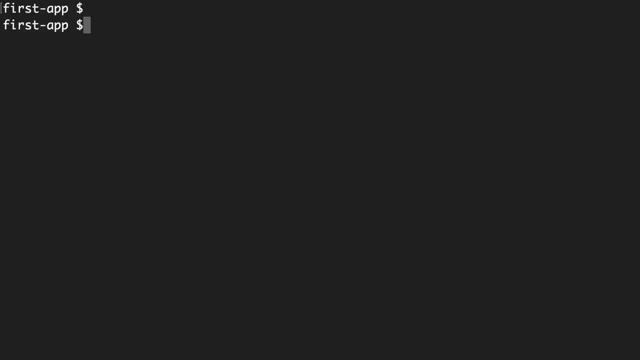 revert the code back to what we had before. Okay, So now we don't have any error. We don't have any errors in this module. Let's go back to the terminal and run this program. So, node appjs. So here on the first line we have filename, which is the complete path to that file, that is. 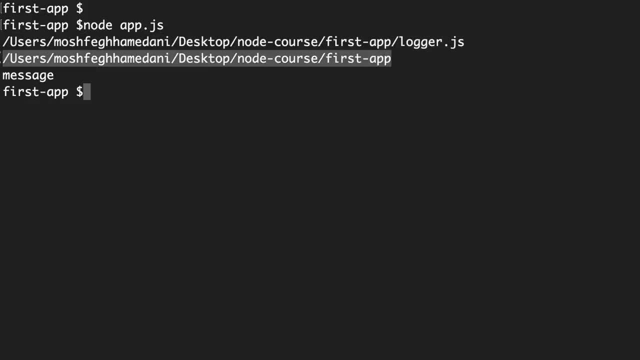 loggerjs, And on the second line we have the path to the directory that contains that module. So now you have a basic idea about node modules and how they work. You know how to create them, how to load them, But node itself comes with a bunch of useful modules. 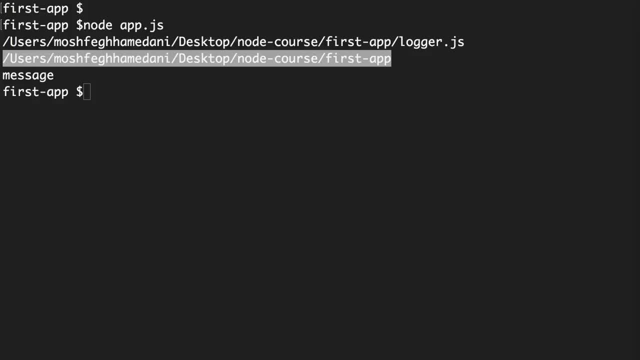 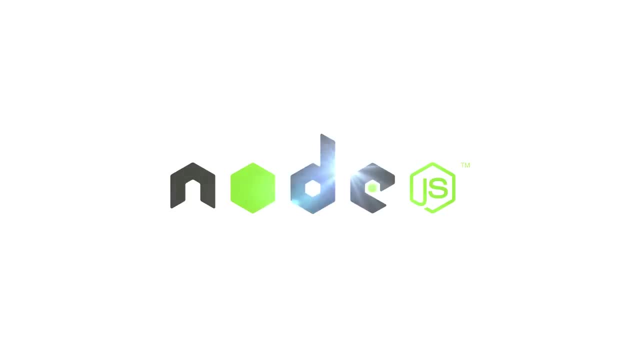 that we can use in a lot of applications, And that's what we're going to look at in the next lecture. Hi guys, Thank you for watching my node tutorial. I wanted to let you know that this tutorial is the first hour of my complete node course, where you will learn how to build. 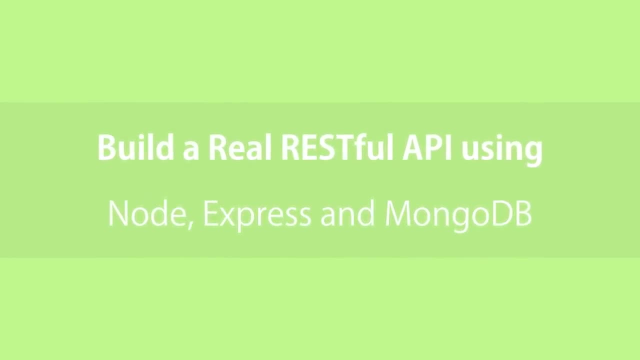 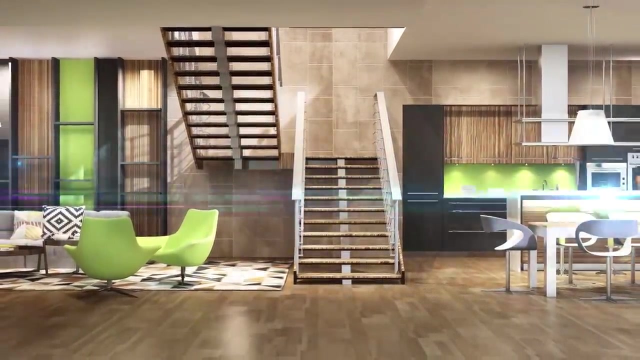 a real RESTful API using node express and MongoDB, All of that recorded with the latest version of node and modern JavaScript. So you will learn the new and modern ways of building applications with node, Unlike other courses that only show you simple dummy examples like how to build. 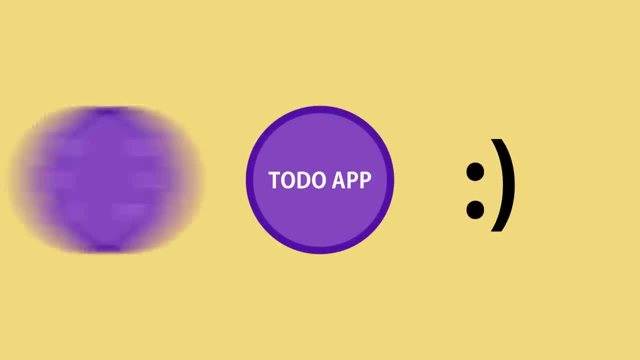 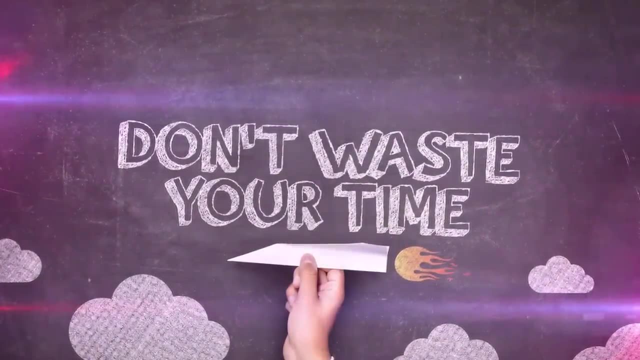 a to-do app. we're going to work on a real world project: A RESTful API for a video rental application. If you have taken any of my courses, you know I don't waste your time by explaining the obvious, like what a code editor or command prompt is. We're going to get straight to. 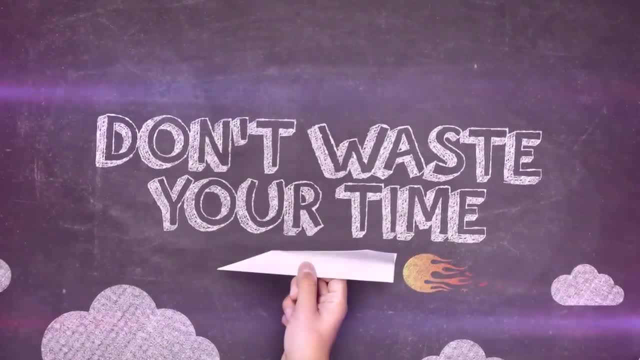 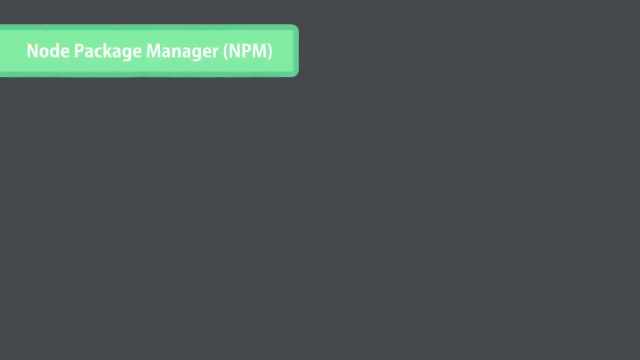 the business And, as part of this, I'll be touching on various important topics that you need to understand Really well, including working with node package manager or NPM. asynchronous JavaScript, including callbacks, promises, async and await. implementing CRUD operations data. 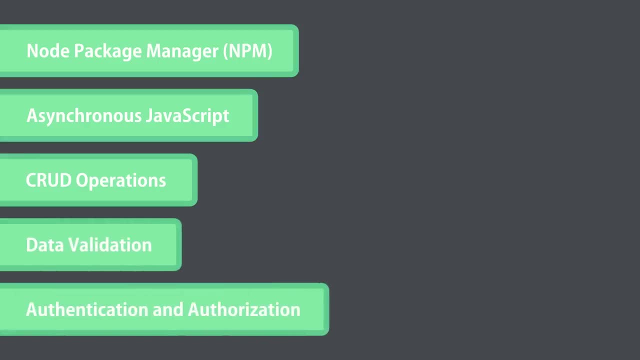 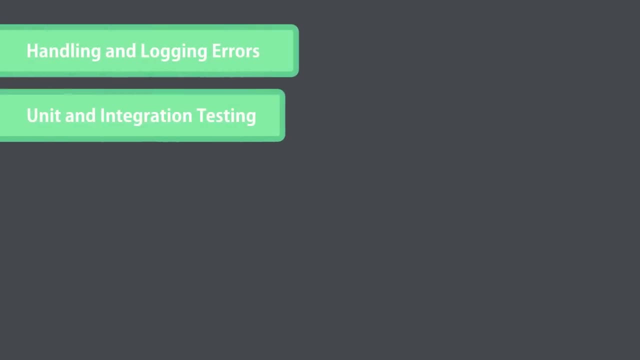 validation, authentication and authorization using JSON web tokens, including role management, handling and login errors, unit and integration testing, test driven development. So you will see, I will build a feature from A to Z using test driven development And finally, we will deploy this application to the cloud Throughout. 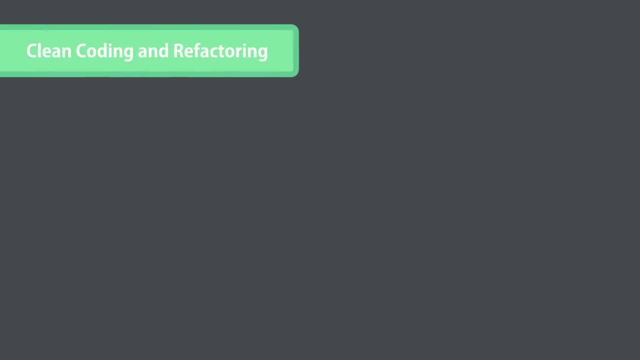 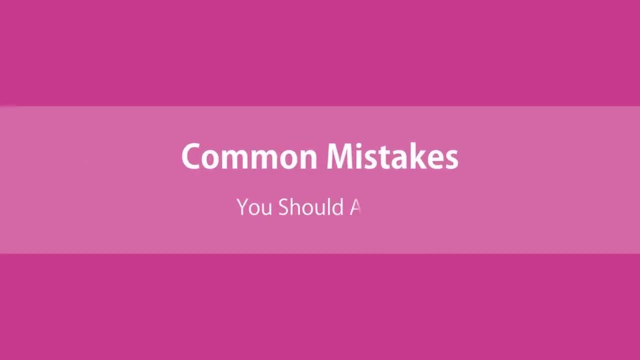 the course, I will share with you lots of clean coding and refactoring techniques, security, best practices, useful libraries to use as part of your development, common mistakes that many node developers make, and much, much more. The course is currently 14 hours long and I'm 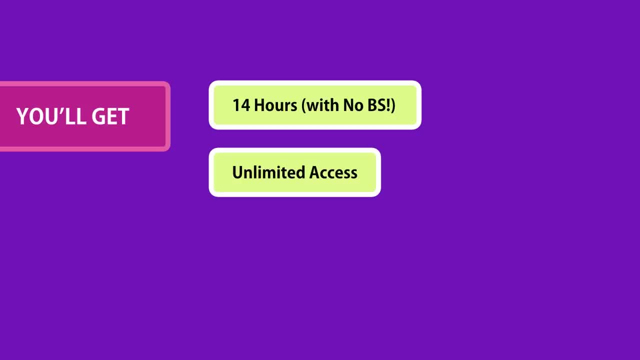 planning to add more content to it in the future. You can watch this course as many times as you want And if you watch it to the end, you will get a certificate of completion that we can add to your resume. So if you are serious about adding note to your resume, I highly encourage you. 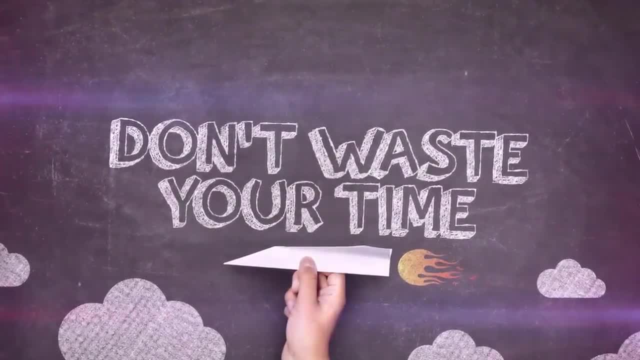 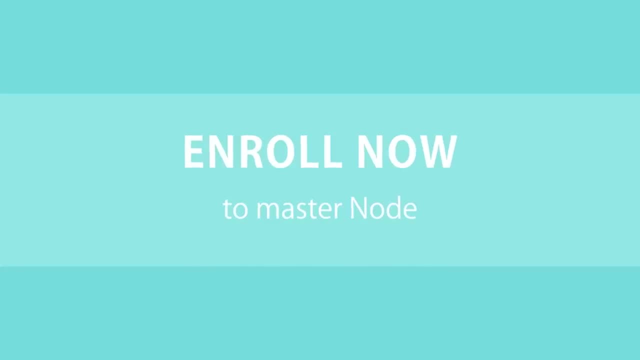 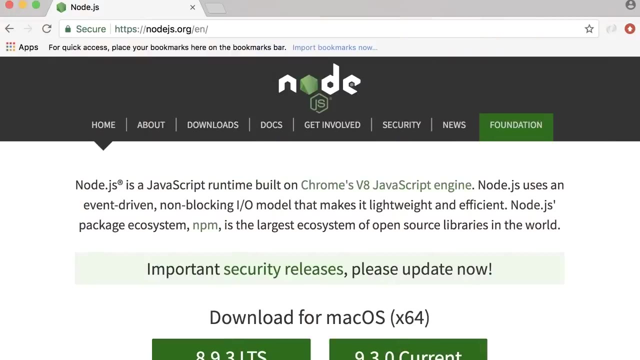 to enroll in the course and don't waste your time jumping from one tutorial to another. So click on the link in the video description to enroll. I hope to see you in the course. so in the last lecture I told you that in node we have a few useful 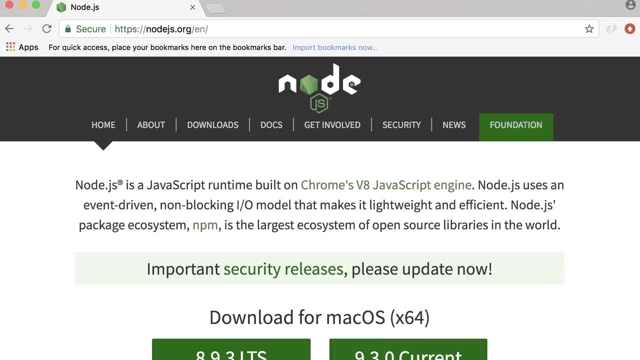 modules that are built into the core of node. I have been working on a bolts database and now I know how to build one of these 야. With these modules, we can work with files, with the operating system, with the network and so on. 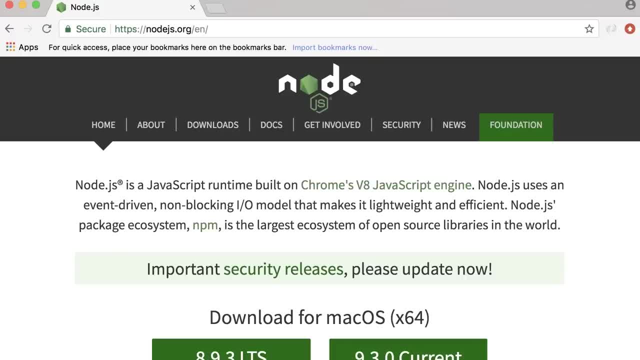 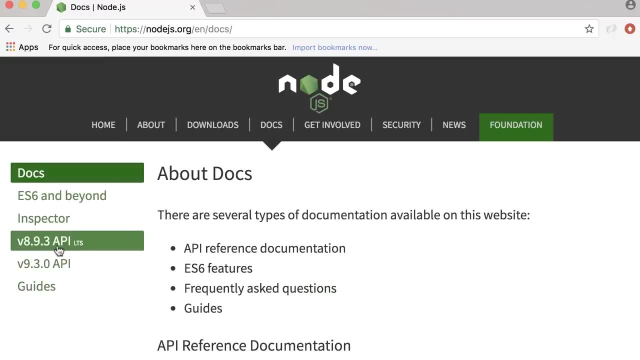 So let's have a quick look at these built-in modules. Head over to nodejsorg, Then go to Docs On the left side. go to version 8.9.3.. That's the current stable release. Chances are, by the time you're watching this video, this version might be different. 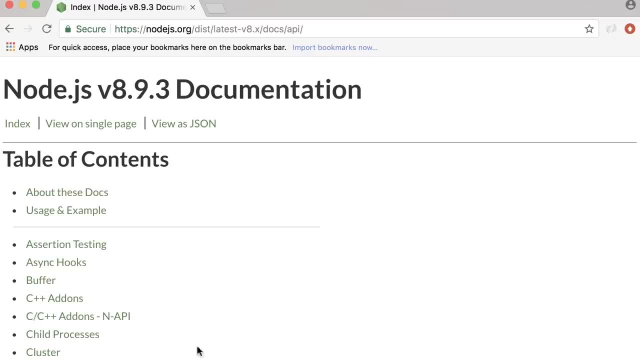 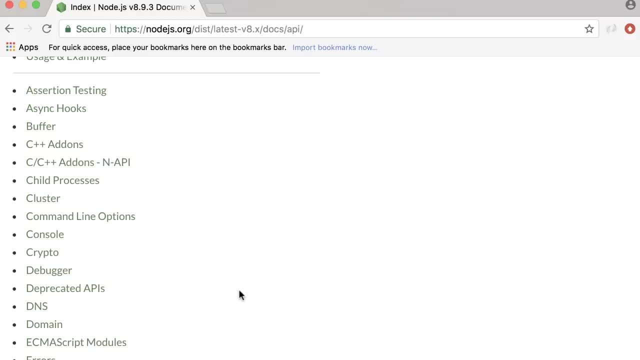 So that doesn't really matter, Just pick that version. Now here in the table of contents we can see the built-in modules. Of course, not everything you see here is a module. For example, we have console, which is our console object. 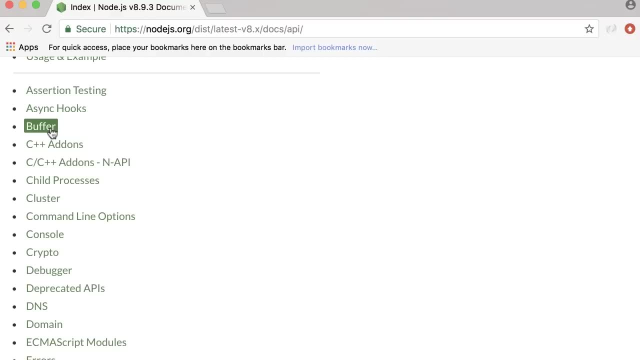 We have buffer, which we are going to learn about in the future in this course. Again, that's a global object, But you can see that this is a fairly short list And some of the items in this list are built-in modules in Node. 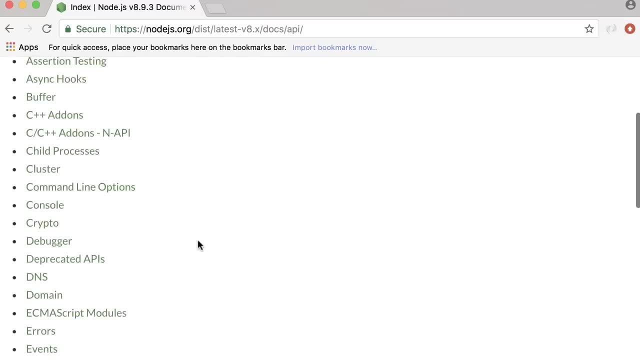 So just that You can see, there are not many modules built into Node. I'm going to highlight a few very useful modules that you should be aware of. For example, we have file system to work with files. We have HTTP that you're going to learn about later in this section. 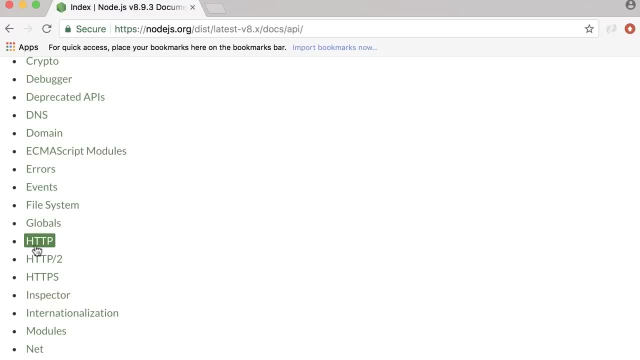 So with this we can create web servers that listen for HTTP requests. We have OS to work with the operating system. We have path, which gives us a bunch of utility functions for working with paths. We have process that gives us information about the current process. 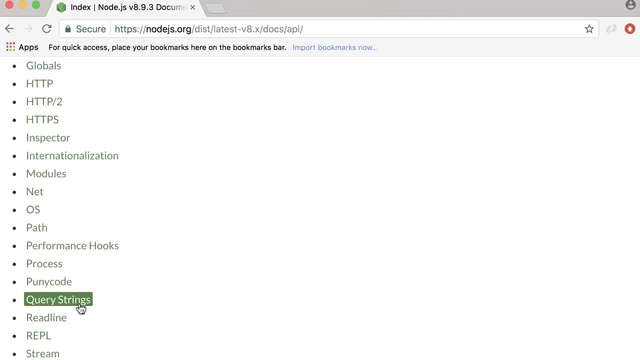 We have query strings, which is very useful in building HTTP services. We have a stream which allows us to work with streams of data- Again, you're going to learn about this in the future- And a bunch of other modules. Now in this lecture, we're going to look at this path module. 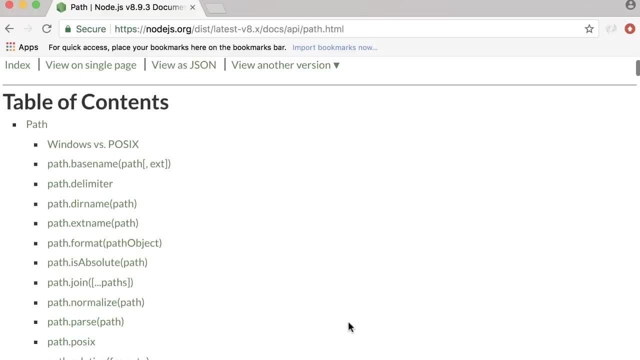 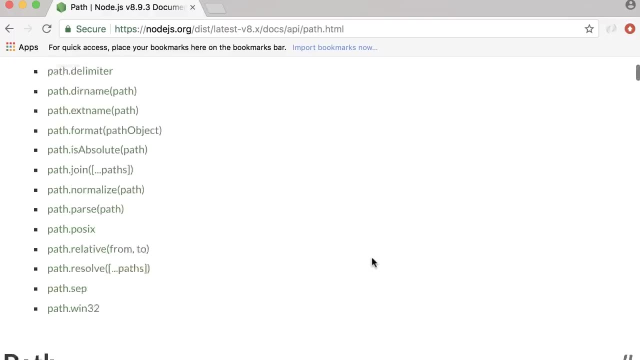 So on the documentation you can see all the functions defined in this module. In this lecture we're going to use the parse method. Now if you scroll down you can see that we have a lot of functions defined in this module. 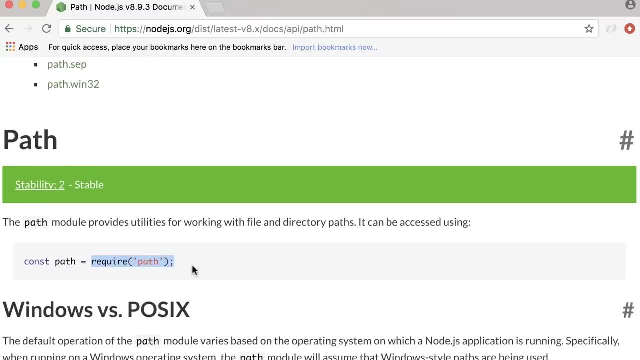 Now let's see how you can use this module. So you have seen the require function. before We call the module, using the require function get the result, which is an object, and store it in a constant. So back in VS Code, in appjs, let's call require. 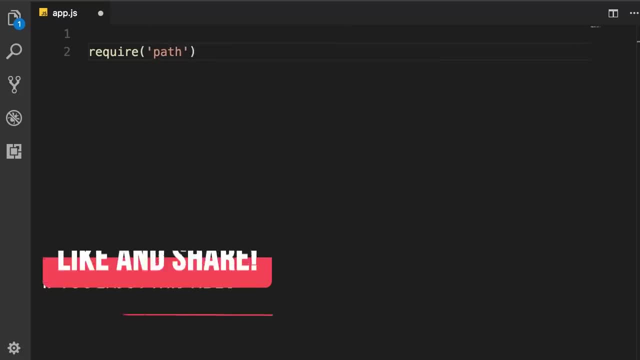 and as the argument use path. Now the argument that we give to this require function node assumes that this is a built-in module. So if there is no built-in module, if there is no built-in module, if there is no built-in module by the name specified here, 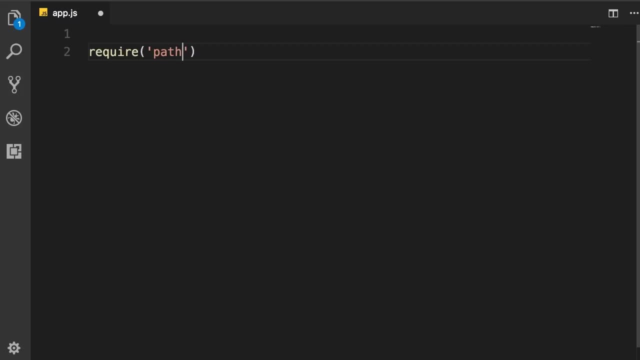 then node looks for the existence of a relative path to a file in this application. So if we have period slash or period period slash, whatever, then node assumes that this is a file in this application. Now, in this case, we're going to load the built-in path module. 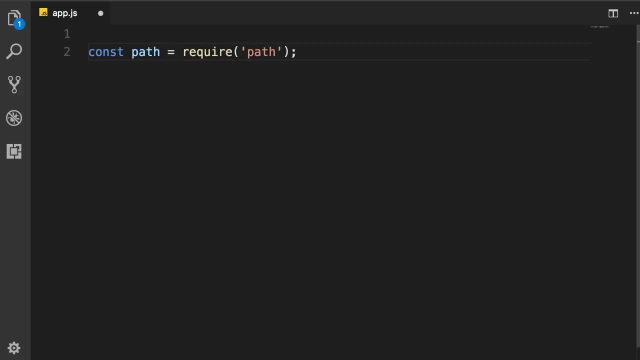 and store it in a constant called path. So this is an object with a bunch of useful methods. The method we're going to use is a built-in path. going to use is the parse method, so i'm going to give it this. underline: underline file name. 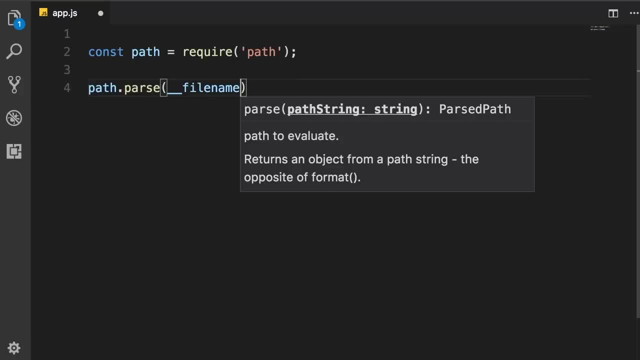 which is one of the arguments in the module wrapper function that you saw in the last lecture. so let's call this and store the result in path object and then finally log it on the console path object. now back in the terminal, let's run this application. so this is the path object it. 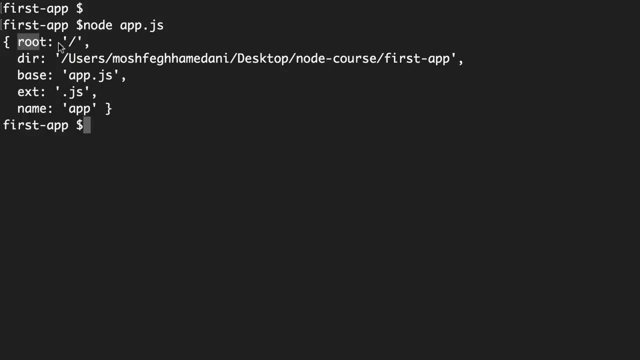 has a few useful properties. we have root. we have dir, which specifies the path to the folder containing this file. here's the name of the file: appjs. here's the extension and here's the name of the file without the extension. so if you want to work with paths, it's much easier to do this. 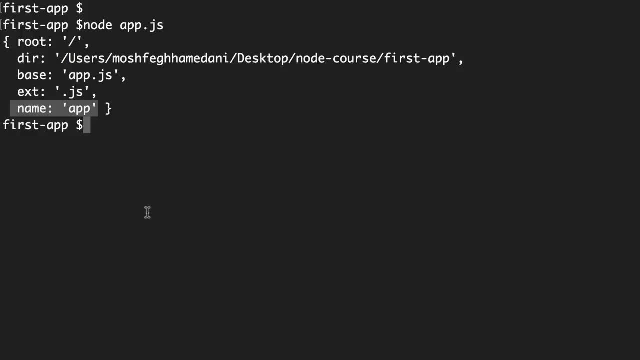 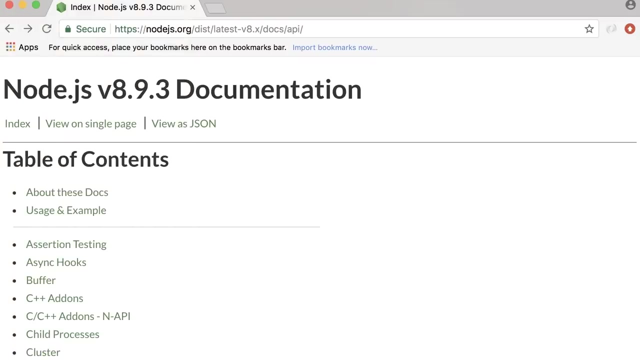 with the path object. so let's run this application. in the next lecture we're going to look at another built-in module that gives us information about the operating system. in this lecture i'm going to show you how to get information about the current operating system. so back in node documentation in the list of modules. 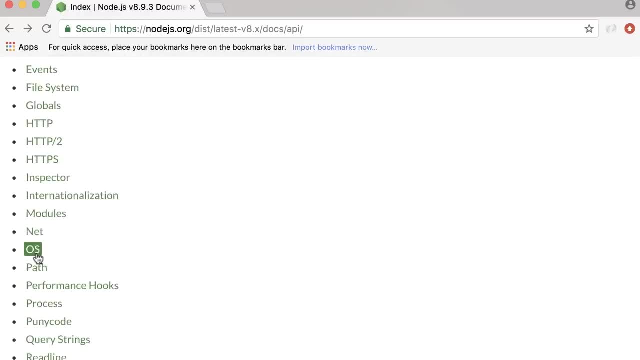 if you scroll down, you can see this os module. let's have a quick look here. so these are the methods that are available in this module. for example, we have free mem, which returns the amount of free memory on this machine. we also have total mem, which is the total memory. 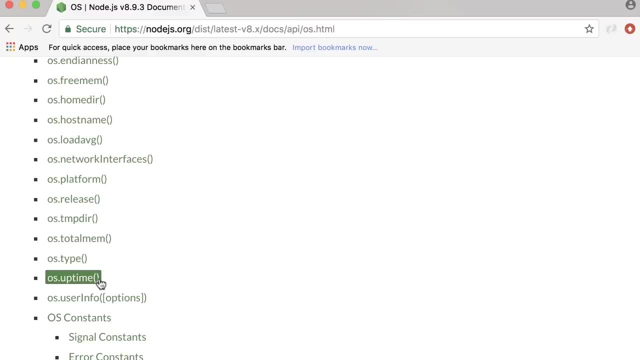 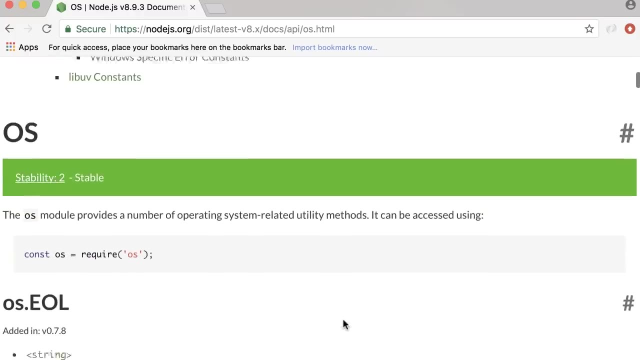 we can get information about the current user, we can get the uptime of this machine and so on. so let's use a couple of these methods here. so if you scroll down, you can see. this is how we load this os module, just like loading other modules. we call the require function. 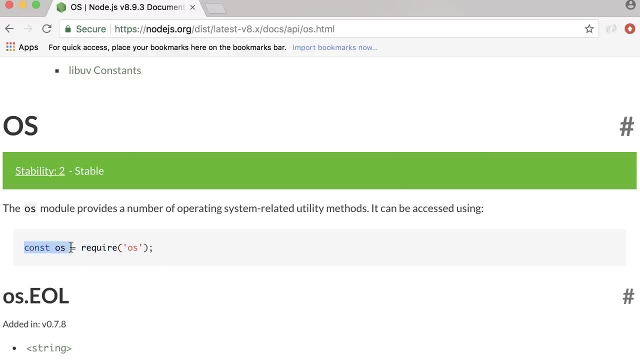 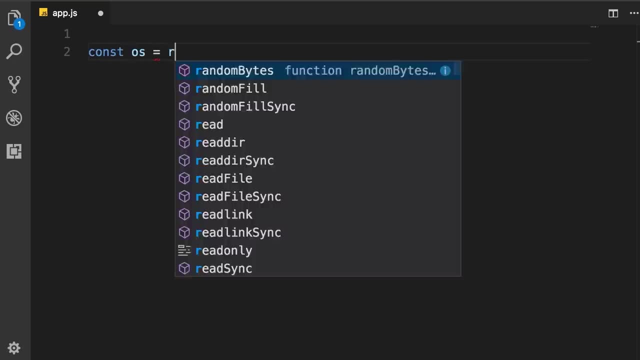 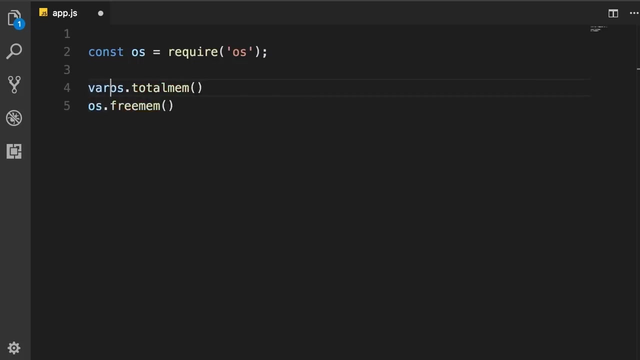 and this is how we load the result in a constant called os or anything. so back in vs code, i'm going to delete all the code here and define a new constant, os, and set it to require os. now we can call total mem method or free mem or other methods. so let me declare a variable and 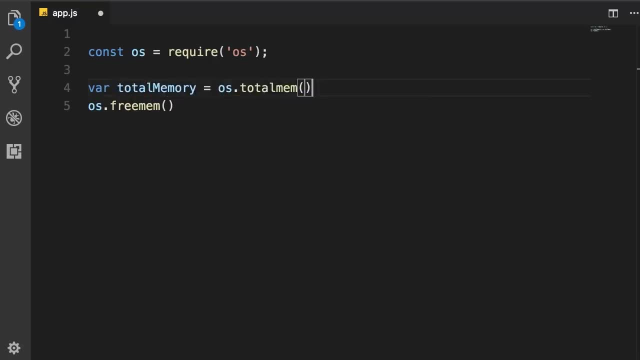 store the result here and similarly for the free memory, free memory. and finally, let's log these values on the console. so console dot log, single quote: we add total memory and append this total memory here. now we can simplify this expression by using a template string which is available in more recent versions. 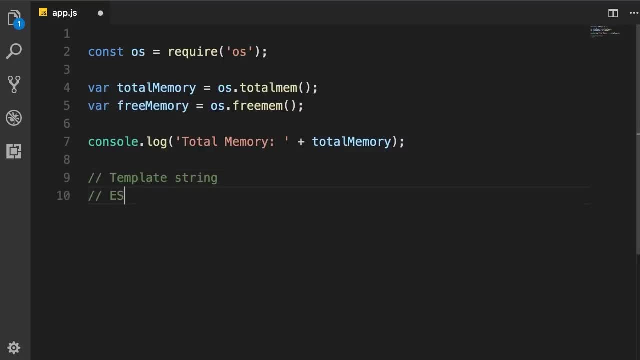 of javascript, and we are going to use this template string to create a more recent version of javascript that we refer to as ES6 or ES2015, which is short for ECMA script 6 or 2015.. That's the specification that defines what features are available in JavaScript. So every year, ECMA. 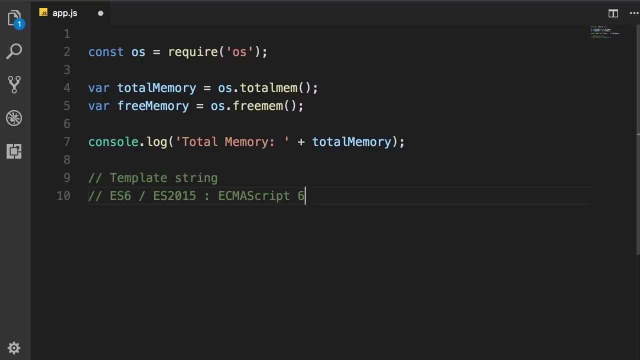 defines new features that should be added to JavaScript And, as you know, different browsers implement different set of these features. But the V8 engine that we have inside of node that's pretty up to date and it implements a lot of new features of JavaScript that is. 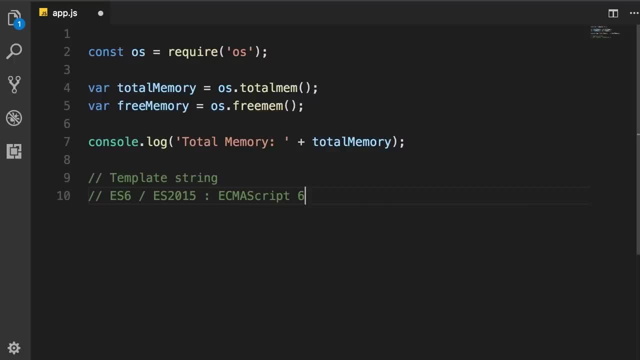 defined in ECMA script. So in ECMA script 6 or ECMA script 2015,. we have a feature called template string, which helps us build a string without concatenations. Let me show you how that works. So consolelog Now. instead of a single quote, we use the backtick character: Backtick. 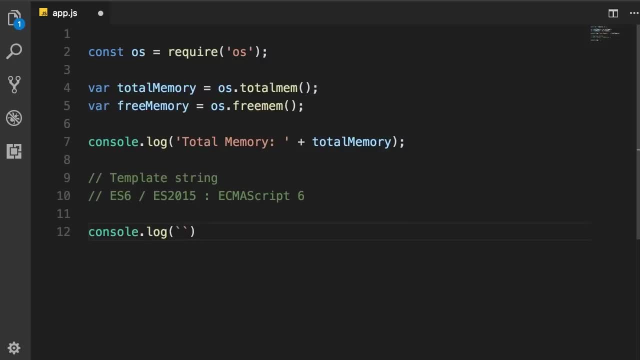 is the character before number one on your keyboard. So here we add some static text like total memory. Now we want to add something here dynamically, So we use dollar sign and curly braces to add a placeholder for an argument. In this case, our argument is this: total memory. 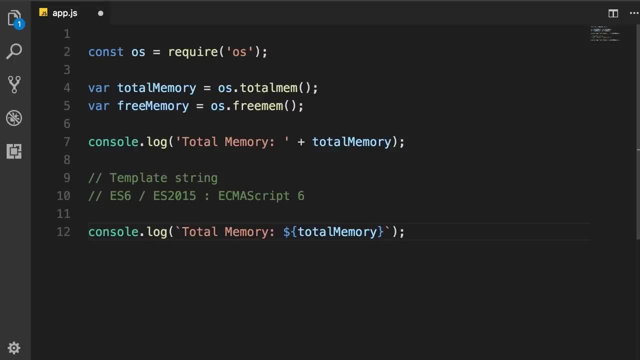 variable. So you can see, with a template string we don't have concatenation. Okay, now I'm going to duplicate this line and change total to free, And here let's add free memory. Okay, now we don't need this first console log. we're done with this. Let's go back to the terminal and run. 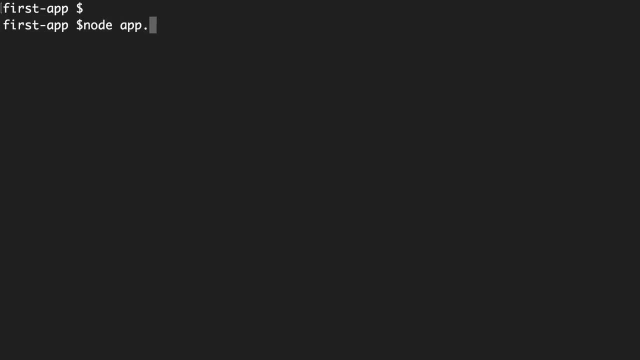 this application, So node appjs, And you can see the total and free memory on my machine. Now what is interesting here is that before node, we could not get this kind of information using JavaScript. JavaScript used to run only inside of a browser And we could only work with the window or document. 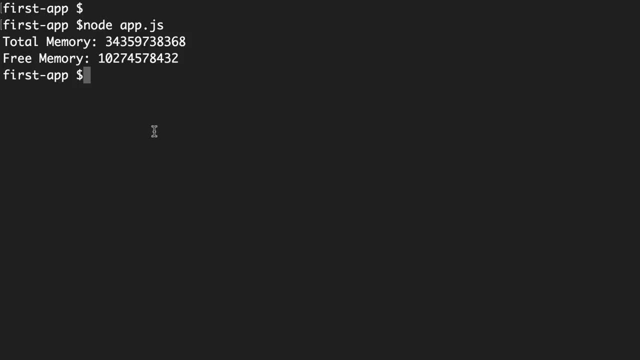 objects, we couldn't get information about the operating system. But when using node, our JavaScript code is executed outside of a browser or, as some people say, on the server. With this we can get information about the operating system. we can work with files. we can work with the. 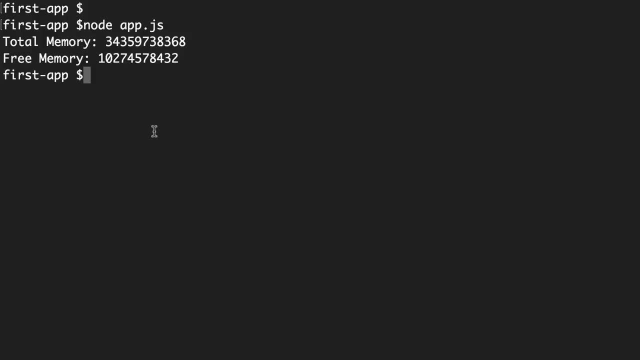 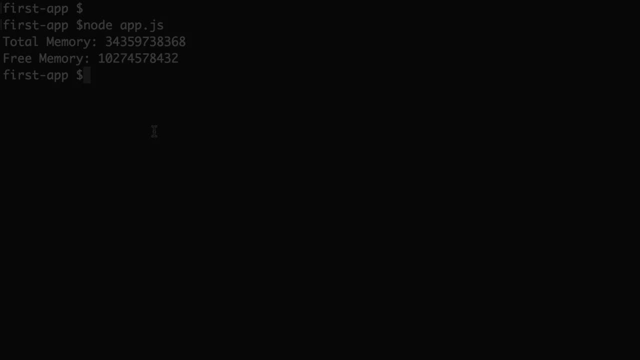 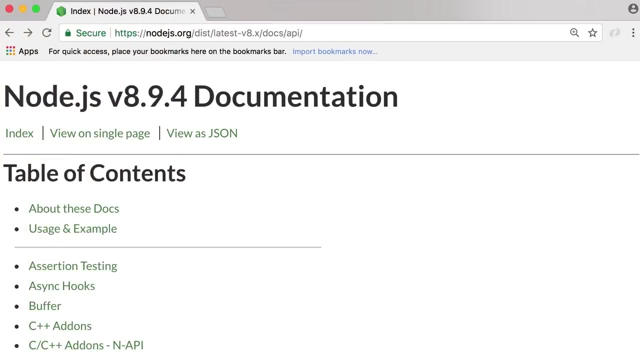 network. For example, we can build a web server that listens for HTTP requests on a given port, And I'm going to show you all the different ways that we can do this. So let's go ahead and start all this. later in this section, In this lecture, I'm going to show you how to work with files in 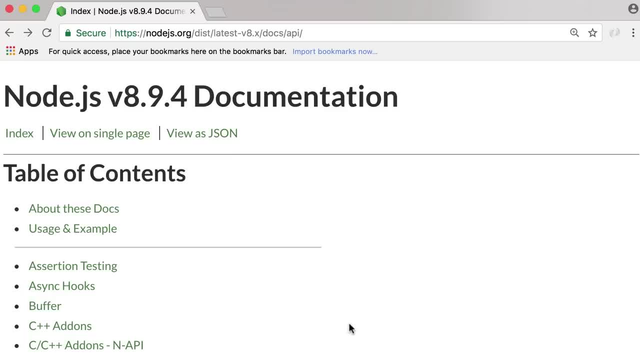 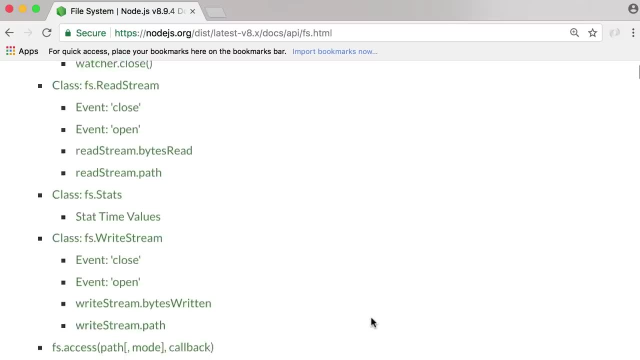 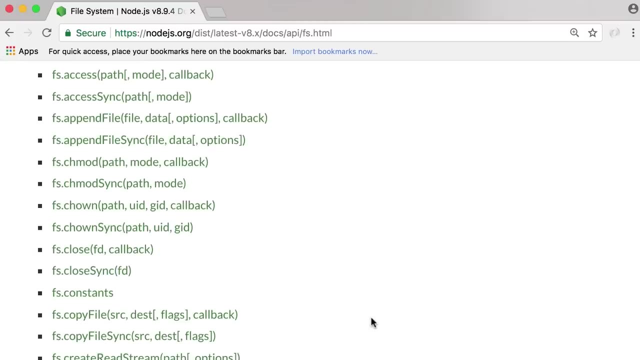 node. So back in node documentation and the list of modules. Here we have a module called file system. In this module we have a comprehensive set of methods for working with files and directories. Now, in this course, I'm not going to waste your time showing you every single. 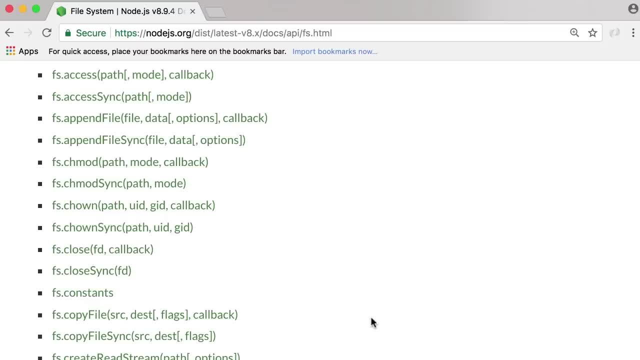 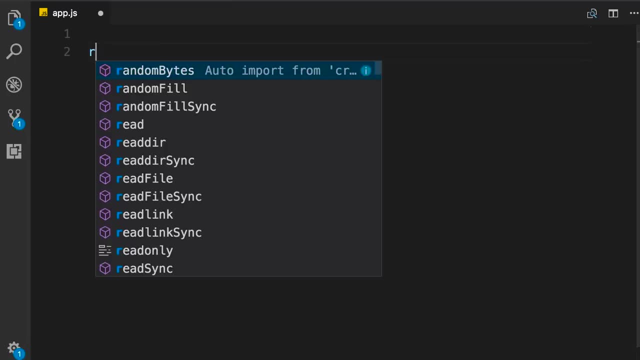 method here, because that will be very repetitive. But let me show you an example So you see how to work with files in node. So back in VS code. first we need to require the FS module, we get the result and store it And this constant. Now fsdot. look almost every operation defined. 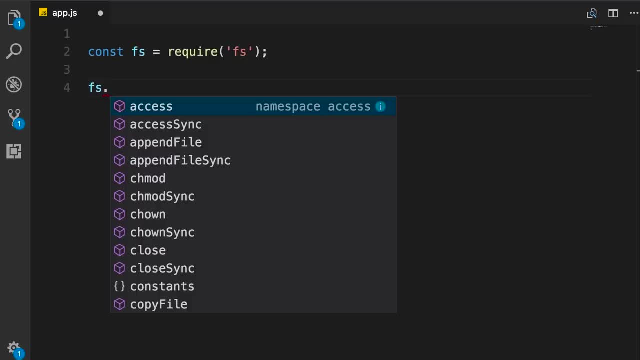 here comes in two forms: synchronous or blocking, and asynchronous or non blocking. For example, look, we have access, which is an asynchronous method. We also have access sync, which is a synchronous method. Now, even though we have these synchronous methods here, you should avoid using them. 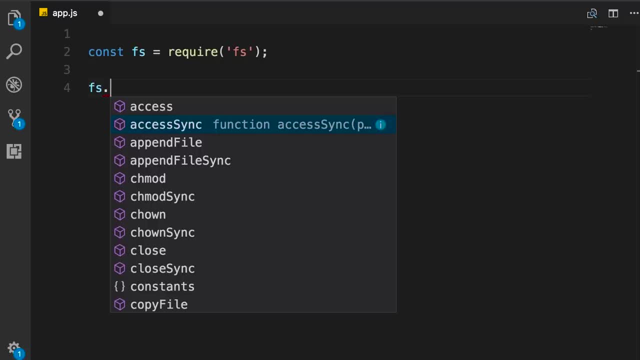 These are there purely for simplicity. in a real-world application, You should use asynchronous methods because these are Non-blocking. so, as I told you in the last section, a node process has a single thread. If you're using node to build the backend for your application, You might have several hundreds or thousands of clients. 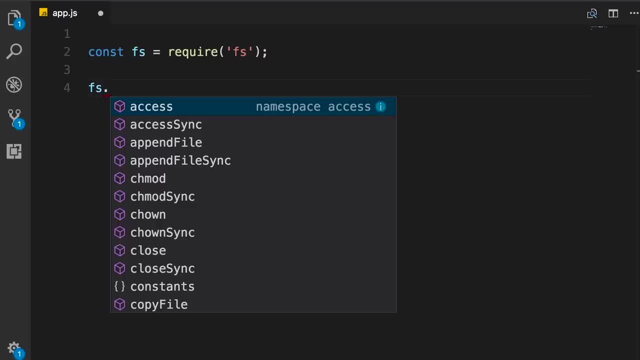 Connecting to that backend. if you keep that single thread busy, you won't be able to serve many clients. So always use asynchronous methods. now that aside, Let's take a look at an example. We're going to look at raid, Dir or directory method. first. I'm going to show you the synchronous form because that's easier to understand. 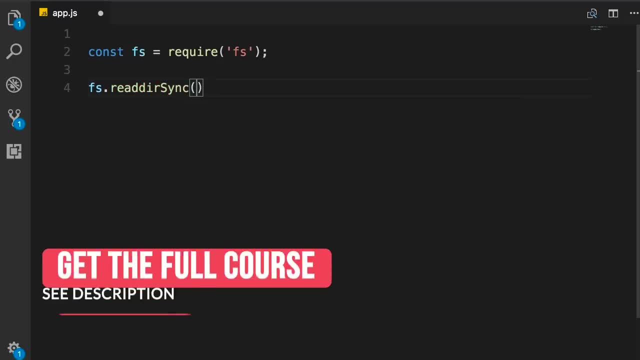 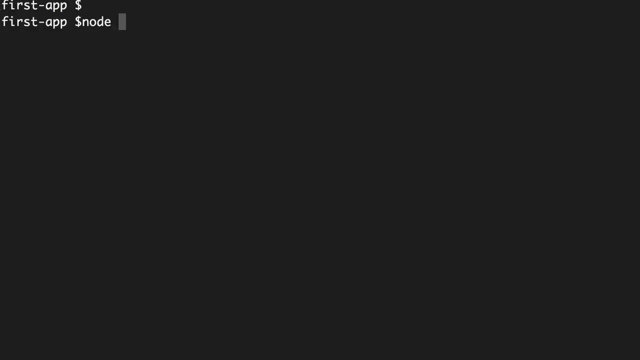 so As the first argument we specify the path Period, slash represents the current folder and this will return all the files and folders in the current folder. So Files will be a string array. now we can display that on the console Very simple, So node appjs. so we can see we get an array of strings and these are the files and 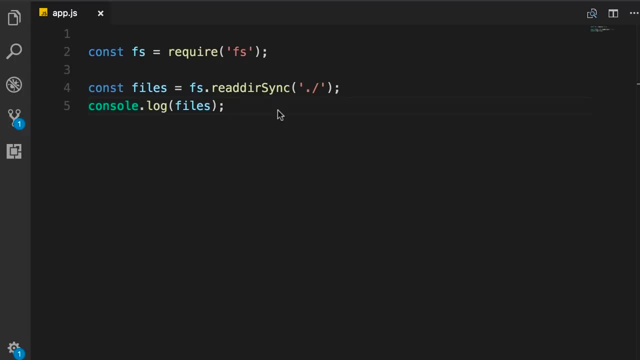 This folder on my machine. Now let's take a look at the asynchronous form of this method. so if s dot read directory, Just like before, the first argument is the path, So the current folder. now all these asynchronous methods take a function as their last argument. Note will call this function when that asynchronous operation completes. We call this function a callback. 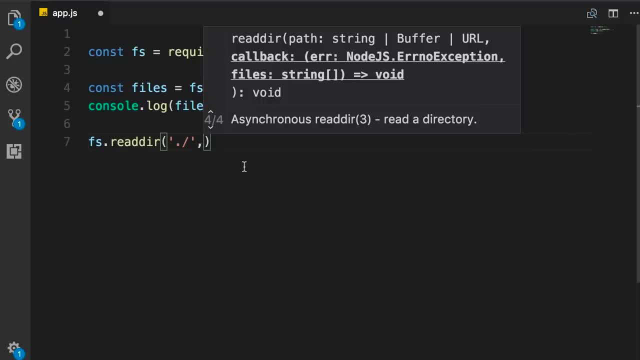 So here look in the intellisense. the second parameter is a callback, and this is a function with two parameters: an error and Result, which is in this case a string array. so here we need to pass a function or a callback function with an error and 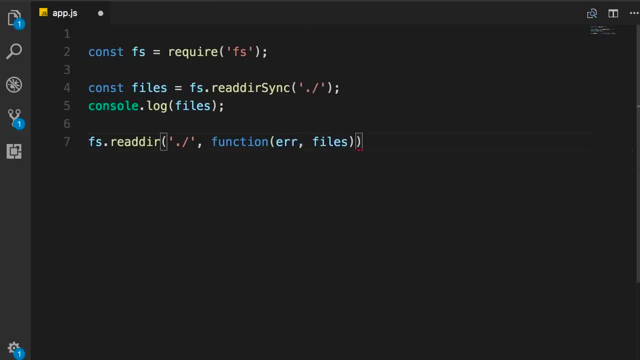 The result, which is a string array. we can call that files. So here we need to check if we have an error or the result. only one of these Arguments will have a value and the other will be null. So if we have error, we're gonna display it on the console. 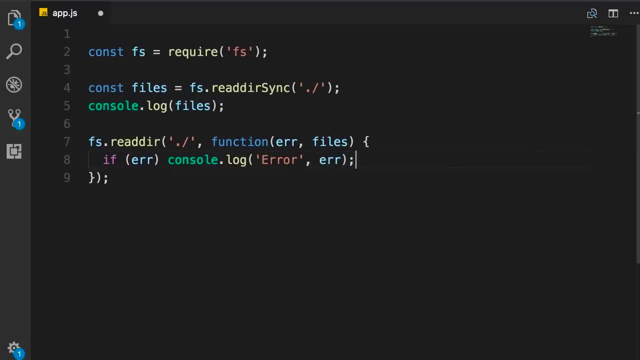 Error error. now, this is not how we handle errors in a real world application. But don't worry about this. later in the course We have a complete section about error handling in note. for now We just want to display this error on the console. So if you have an error, we displayed, otherwise we display the result. So console dot log. 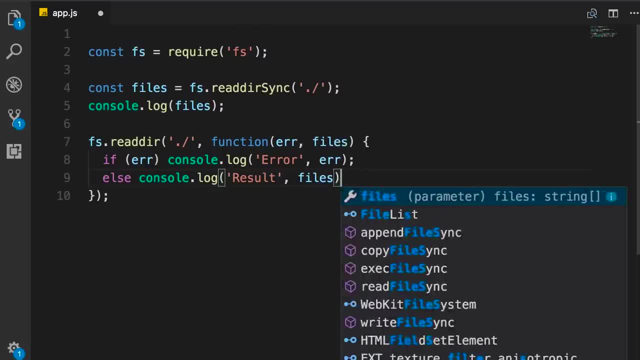 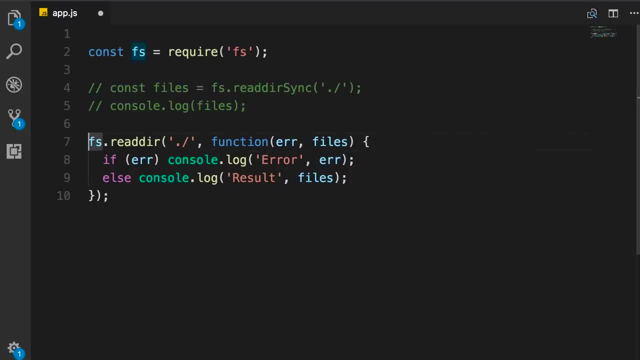 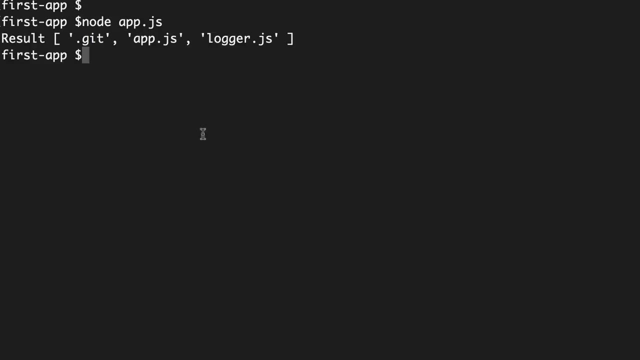 Result and we can display this string array. So I'm going to comment out These two lines so we can only look at the result of this asynchronous read directory note: appjs. So we got result and this is exactly the string array that we had before. now Let's simulate an error. 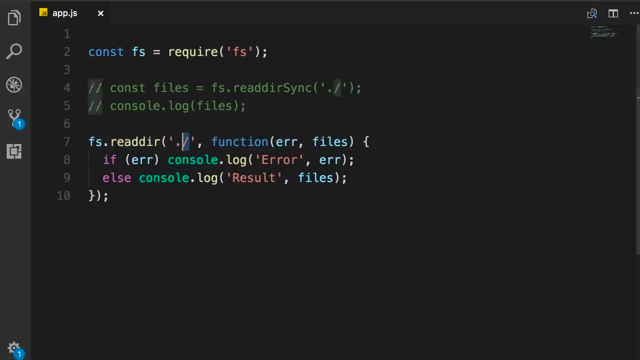 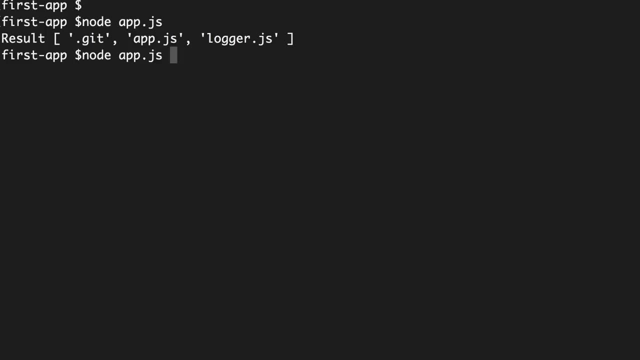 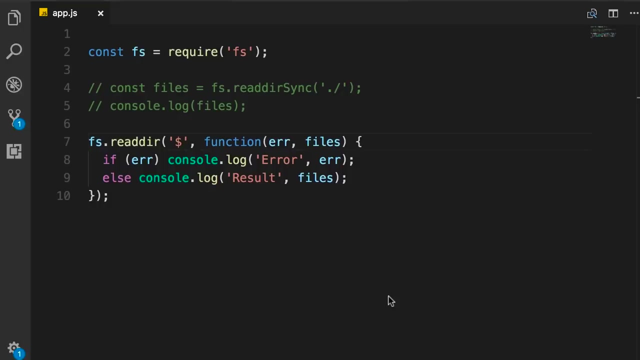 so I'm going to go back in the code and change this argument to, Let's say, a dollar sign. save back in the terminal Note appjs. this time we got an error: No such file or directory. So to recap, in order to work with files and directories in note first, 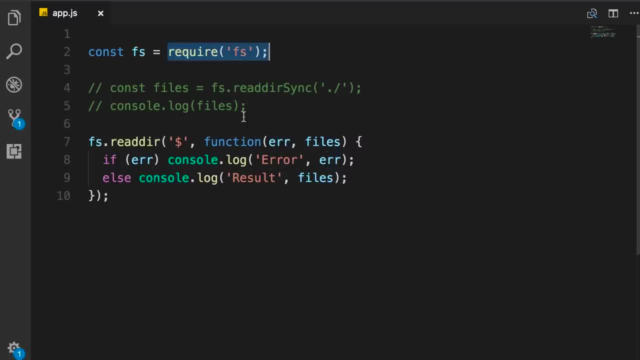 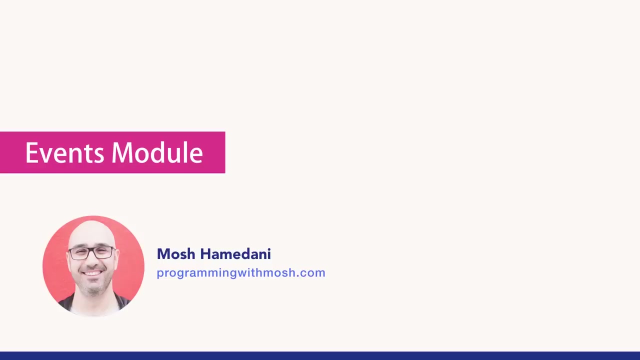 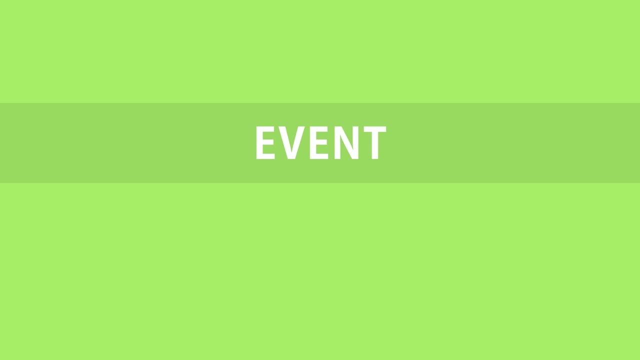 You need to require the FS module and then use one or more of the methods defined in this module. all these methods come in pairs, asynchronous and synchronous. always prefer to use a synchronous methods. One of the core concepts in node is the concept of events. in fact, a lot of nodes core functionality is based on this concept of events. an 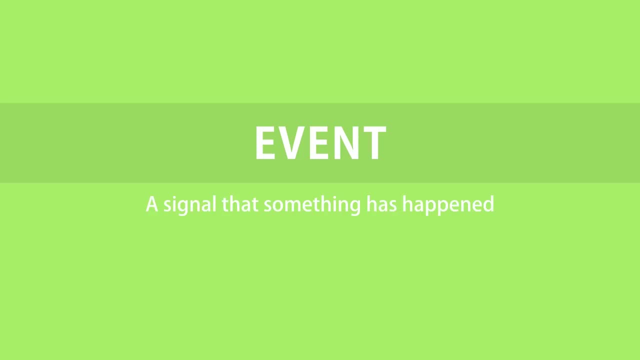 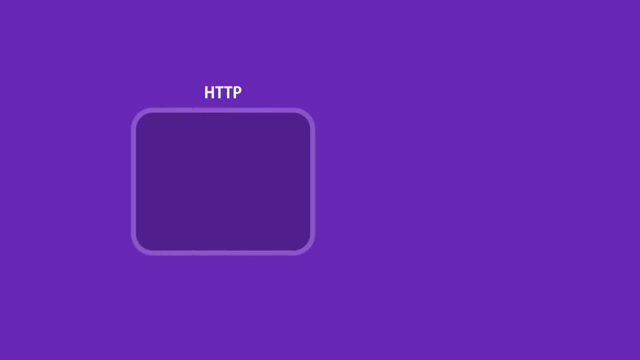 Event is basically a signal that indicates that something has happened in our application. For example, in node We have a class called HTTP that we can use to build a web server. So we listen on a given port and every time we receive a request on that port, that HTTP class. 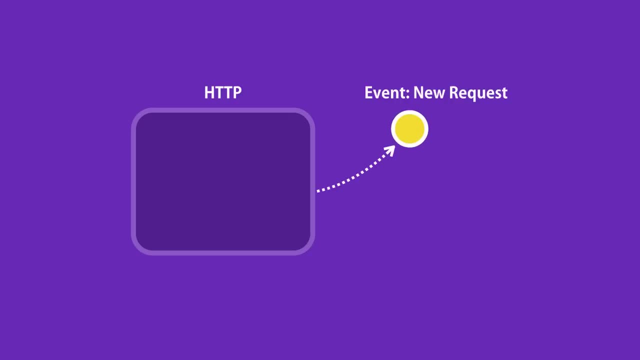 Raises an event. now our job is to respond to that event, which basically involves reading that request and returning the right response. So as you go through nodes documentation you can see that several classes in node raises different kinds of events and in your code You might be interested to respond to those events. 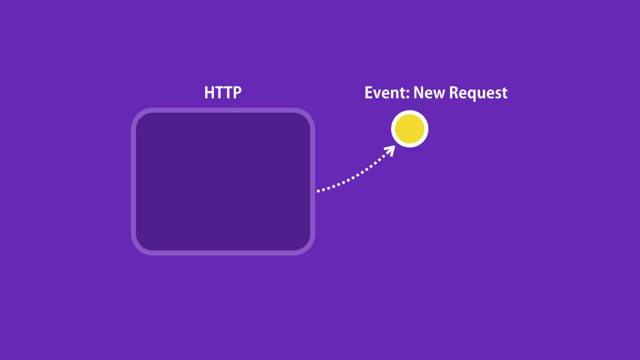 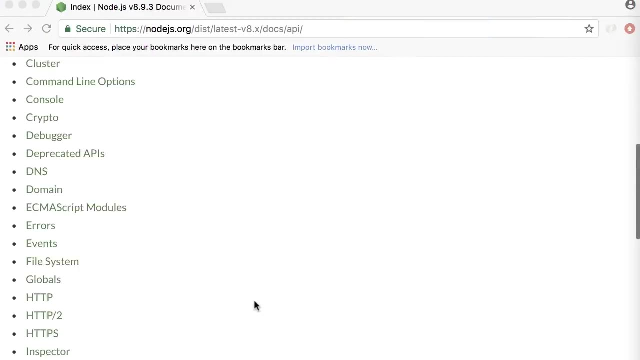 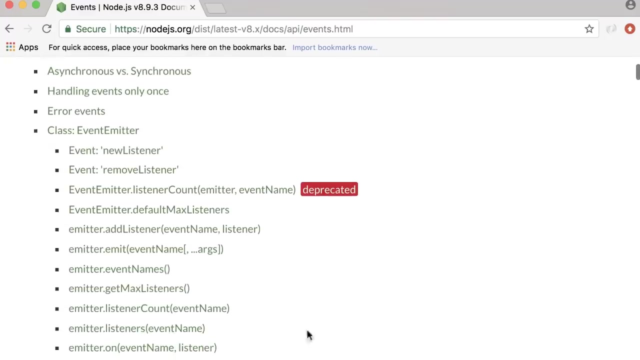 So in this lecture I'm going to show you how to work with the events module. Now back in nodes documentation once again. in the list of modules you can see here we have this events module. So in this module we have one class that is called event emitter. 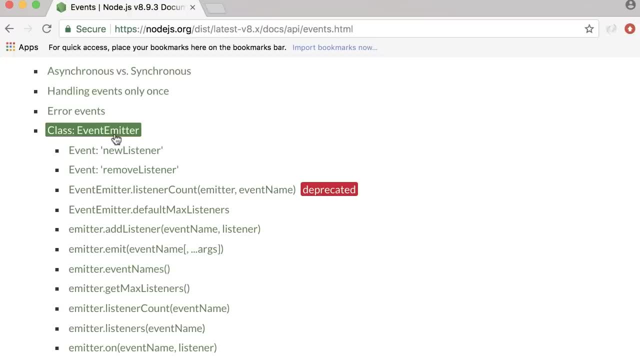 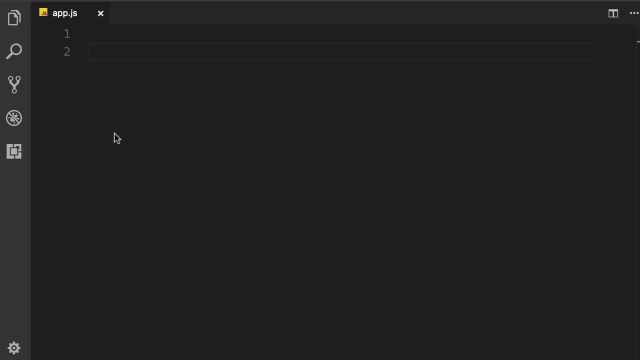 It's one of the core building blocks of node and a lot of classes are based on this event emitter. So let's see how we can work with this event emitter. I can vs code. first, Let's load the events module, So require events. Now, here, when we call the require function, we get the event emitter class, So constant. 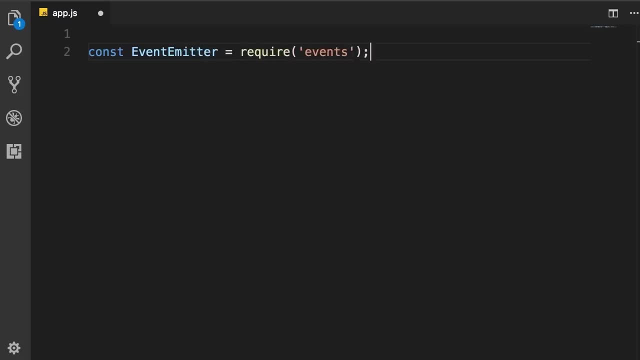 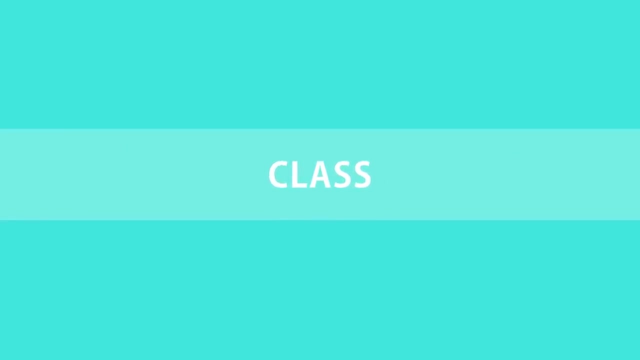 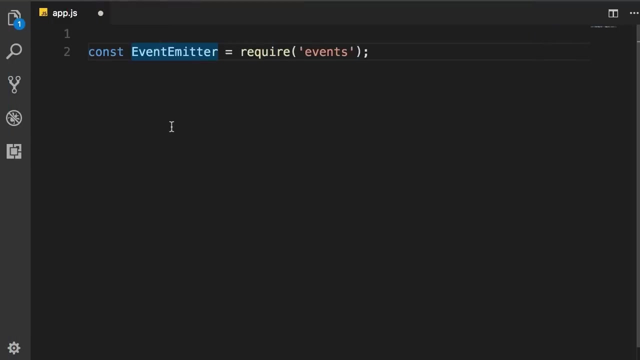 event emitter. Note that here, in terms of the naming, the first letter of every word is uppercase. This is a convention that indicates that this event emitter is a class. It's not a function. It's not a simple value, It's a class. a Class is container for properties and functions, which we call methods. So in this event, emitter class. 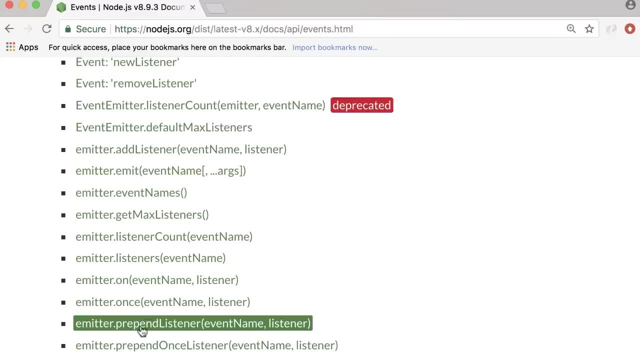 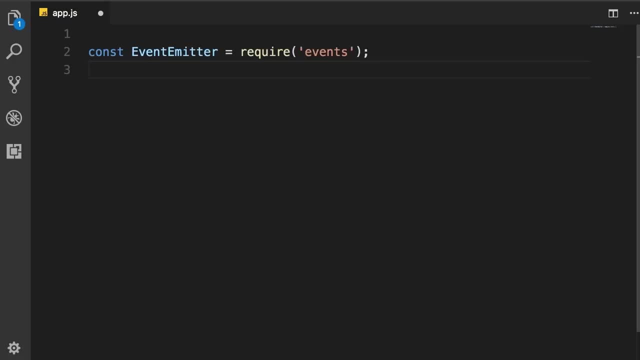 We have these methods that you see here in the documentation, So a class is a container for a bunch of related methods and properties. Now here, in order to use this event emitter, first we need to create an instance of this class, so constant, and Emitter. We said this to new. 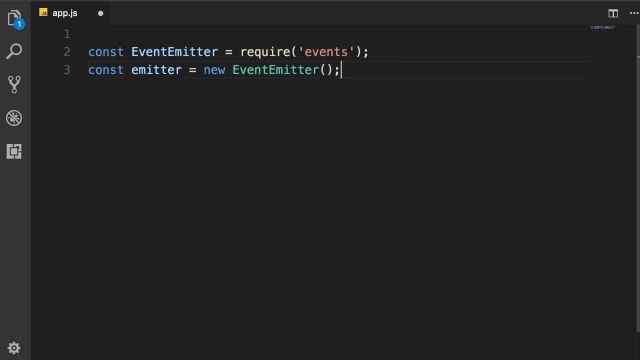 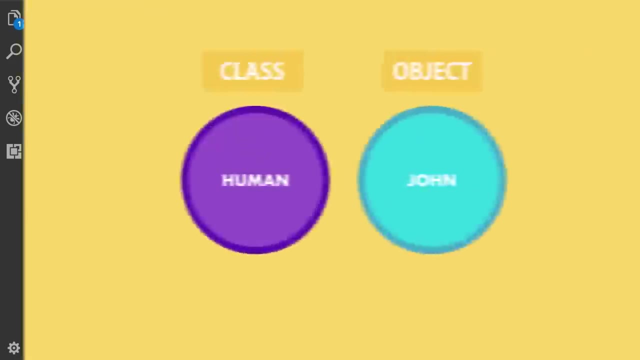 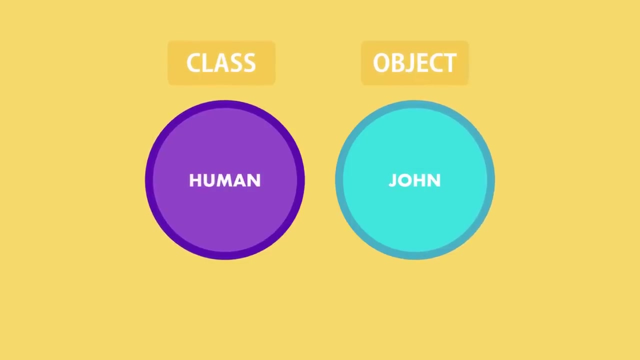 event emitter. So here this emitter is an object. in case you don't know the difference between a class and an object, let me give you a metaphor: a Class is like human and an object is like an actual person, like John, Mary and so on. so a class defines the properties and 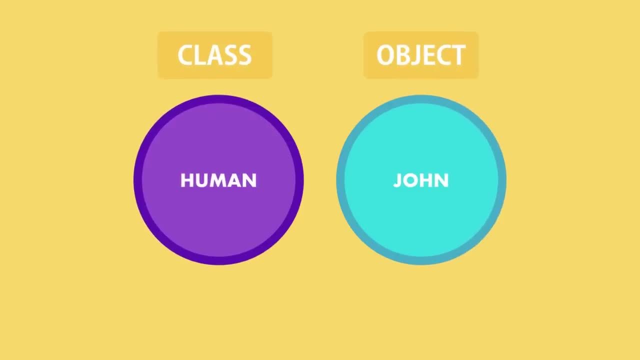 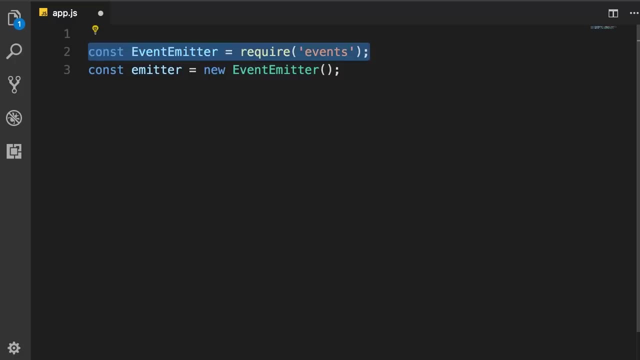 behavior of a concept, like a human, but an object is an actual instance of That class. Okay, So here, this first event emitter is a class. It's a blueprint and defines what an event emitter can do. But this second emitter is an actual object. This is the one that we're going to use in our application. 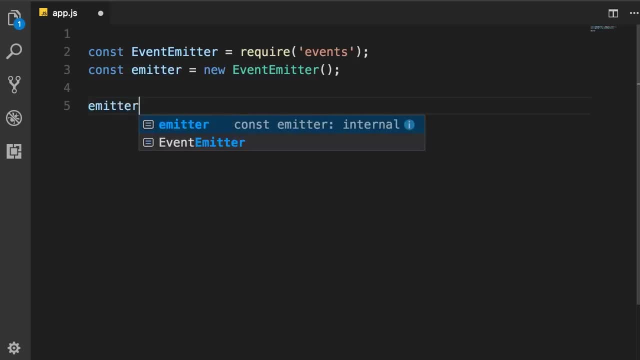 so This emitter has a bunch of methods. Look, these are all the methods that you saw in the documentation. Now, even though here we have more than 10 methods, most of the time we use only two of these methods. one is emit That we use to raise an event. 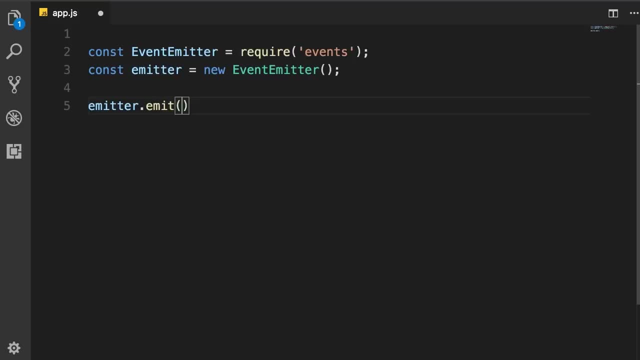 The first time I saw this method, it didn't make sense to me because English is my second language And I didn't know what emit means. So if you're in the same boat and it basically means making a noise or produce something, in this case You're making a noise in our application. 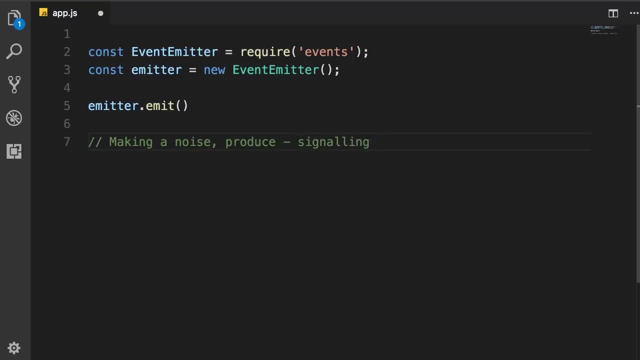 We're signaling that an Event has happened. Okay, so that's the meaning of emit. now, here We pass an argument that is the name of the event, Let's say message logged. In the future we're going to extend our logger module and every time we log a message, 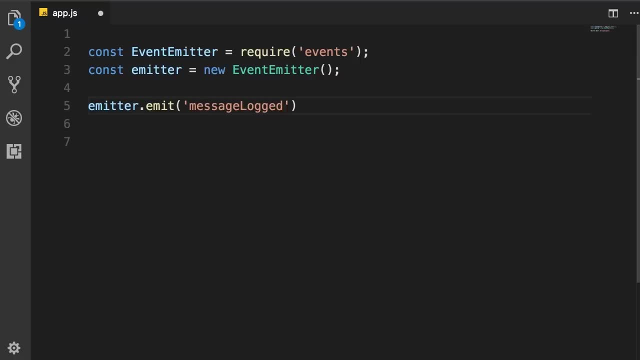 We're going to raise an event called message locked. Okay, Now if you run this application, nothing is going to happen. Let me show you back in the terminal node appjs. Look, nothing happened, Because we have raised an event here but nowhere in our application we have registered a listener that is interested in that event, a. 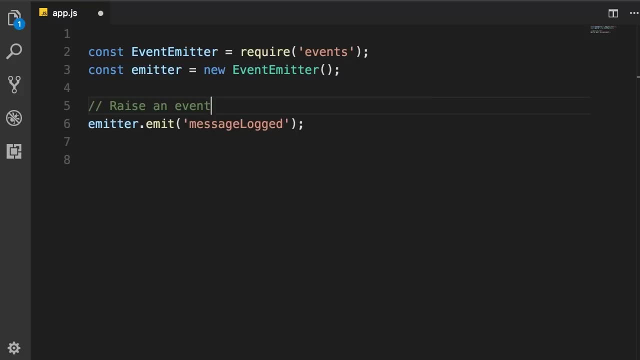 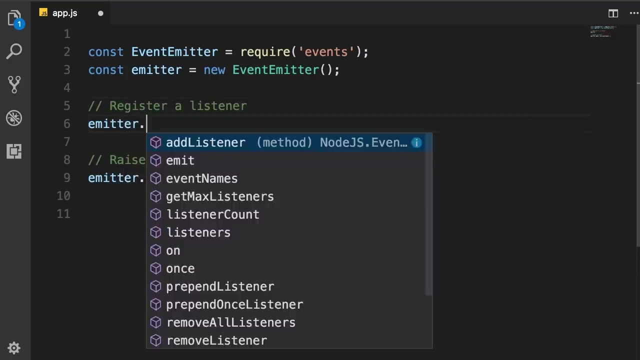 Listener is a function that will be called when that event is raised. Okay, so let's register a listener. that will be called when the message log event is raised. so register a listener. so emitter dot. Look, here we have this method at listener. Well, we have an alias for this that we use more often. that is on, if you have worked with J query. 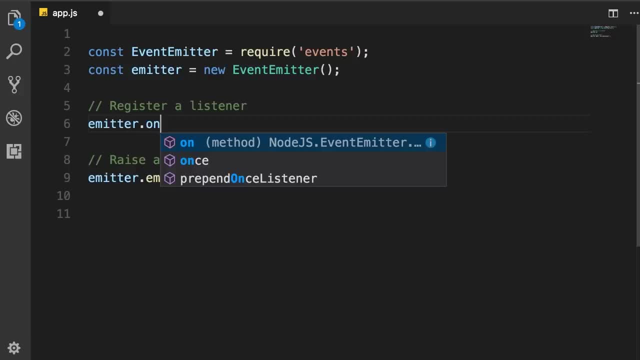 You have seen this before. so on, or at listener. They're exactly the same, but quite often we used on method. Now this method takes two arguments. The first one is the name of the event, in this case message logged, and The second one is a callback function or the actual listener. 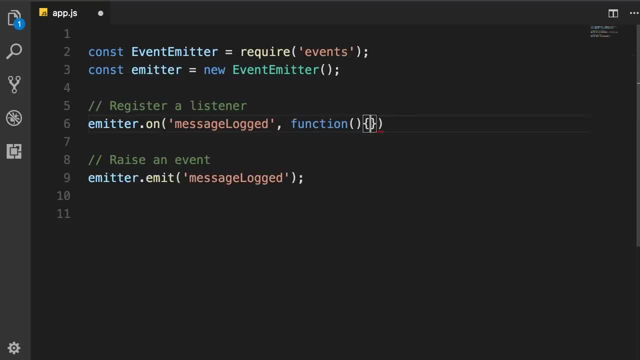 So here we have one argument and then one long message have been created and that point in the comment line is: findn a callback message had login a function, and this function will be called when that event is raised. okay, now for now, I just want to lock a message in the console. so, console, let's. 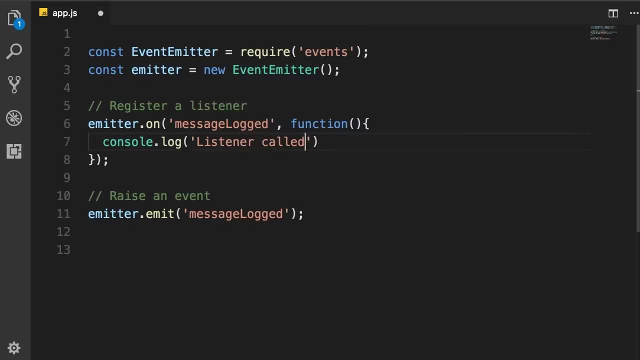 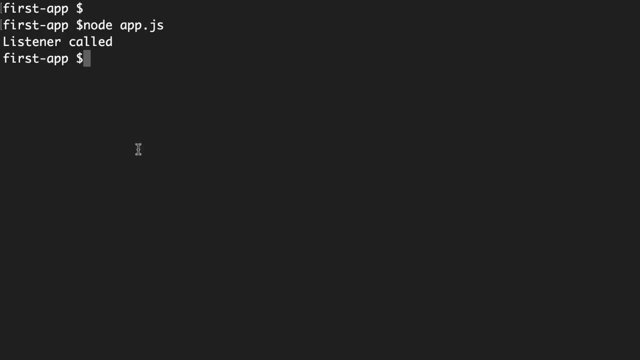 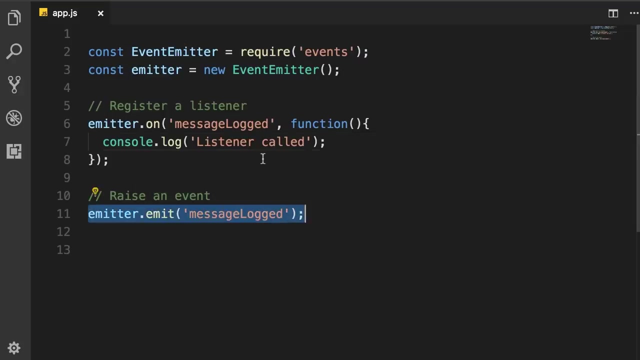 say, listener called like this: now let's run this application, so node appjs, and we got this message: listener called. so this indicates that when we raise this event, this callback function or listener was called. okay, and of course the order is important here, if you registered this listener after calling the emit method. 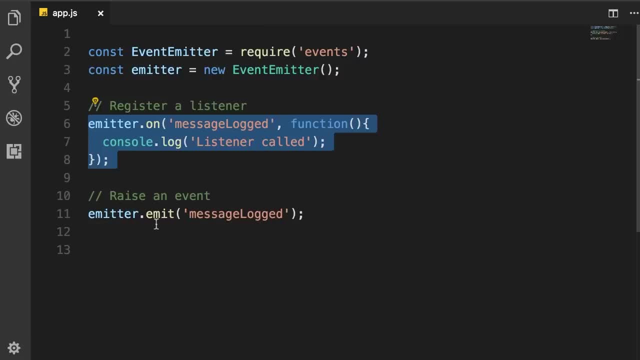 nothing would have happened, because when we call the emit method, this emitter iterates over all the registered listeners and calls them synchronously. okay, so this is the basic of raising events and handling them using the event emitter class- you. but quite often, when we want to raise an event, we also want to send some data. 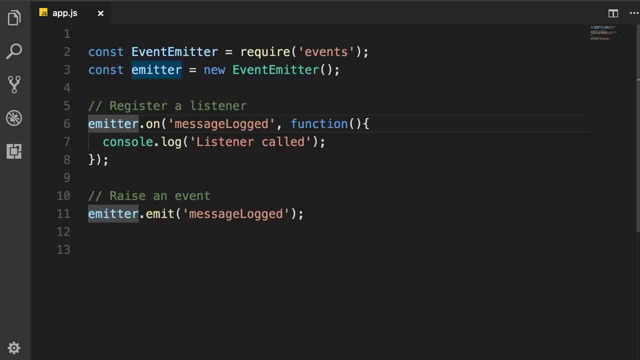 about that event. for example, in our logger module, when we log a message, perhaps our remote login service will generate an ID for that message. perhaps we want to return that ID to the client, or it may give us a URL to access that logged message directly. so here is our login message. so I'm going to access some of those messages and I'm going to 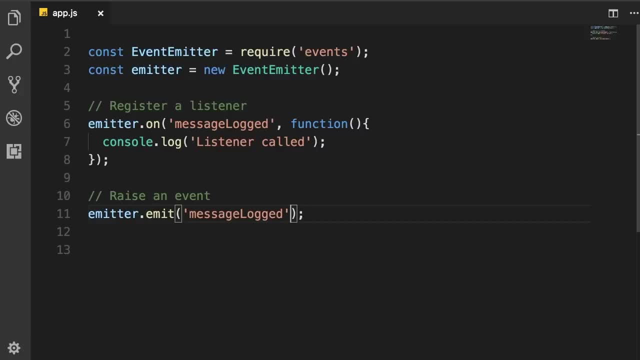 raising an event, we can add additional arguments, which were referred to as event arguments. so we can add an ID like one, and we can add a URL. but, as you can see, these magic values here are a little bit confusing. if you want to send multiple values about an event, it's a better practice to encapsulate those. 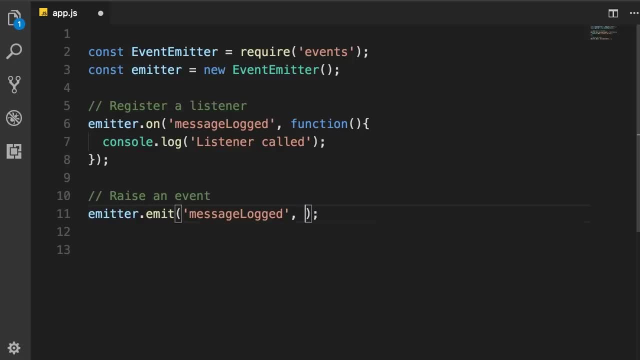 values inside an object. so here we had an object. we give it a couple of properties like ID- we set it to ID of this message that is logged- and another property URL like this: okay, so we refer to this object as event argument. now, when registering a listener here, this callback function, this actual listener, 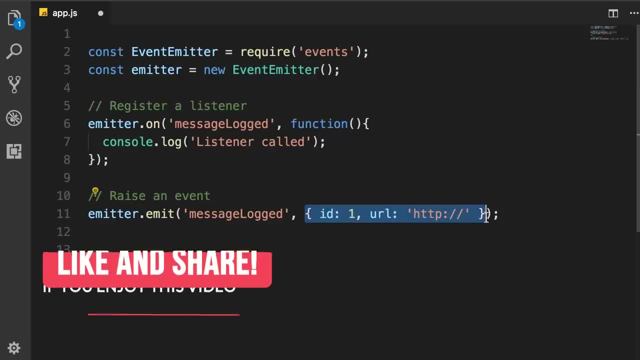 can also receive this event argument. so here we add a parameter called arg. you can call it anything, the name doesn't matter, but by convention we often use arg, or some people use e to refer to the event or event, arg- whatever you prefer is perfectly fine. so here we have arg. now let's log in on the console. very simple. 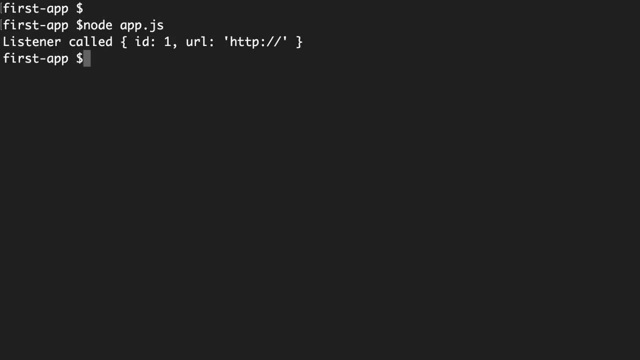 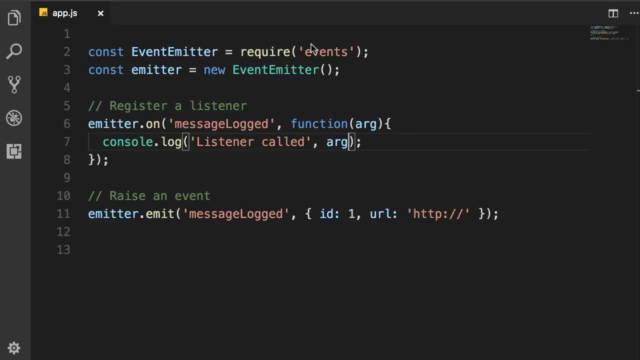 let's run this application, so note: okay, look, listener called and here's our event arg and with this technique we can pass data about the event that just happened. now one last thing to make this code a little bit simpler. in ES6 or ECMAScript 6 we have this feature called arrow function. 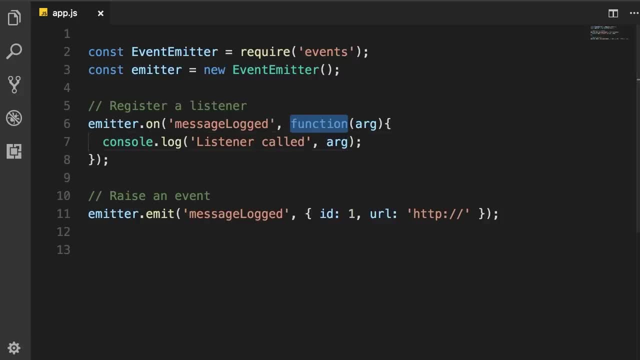 with an arrow function, we can get rid of this function keyword. so here we have the arguments and after that we have the body of that function. now, to separate the two, we use an arrow, and that's why we call this arrow function. you can see, this syntax is a little bit simpler and a lot of people prefer to use arrow. 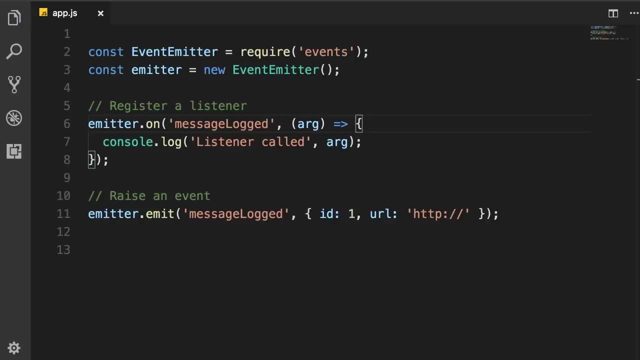 functions in ES6. now here's a simple exercise for you. let's imagine in our log, our module, just before calling our remote service to log the message, we're going to raise an event called logging, and while raising this event we also want to send some data. that is the message that we're going to log. so what? I want you to do is go with our widget and type here a command, drop down to our page and then the other bar desire do the feature here and casually we can do it. now we can write a simple code and that's what I we're gonna allow our 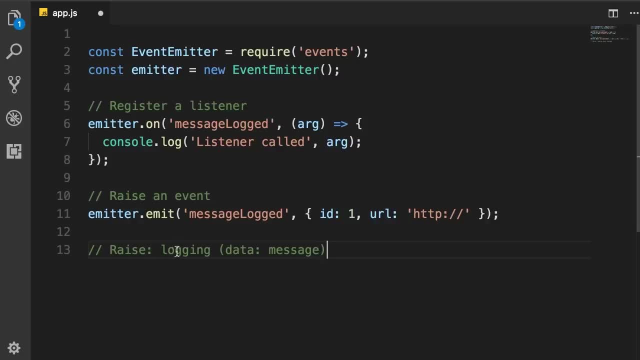 Is to use what you have learned in this lecture and raise and handle this logging event. It's a very simple exercise. I just want you to get used to this syntax Now. in the real world. it's quite rare that you would work with this event. emitter- object. 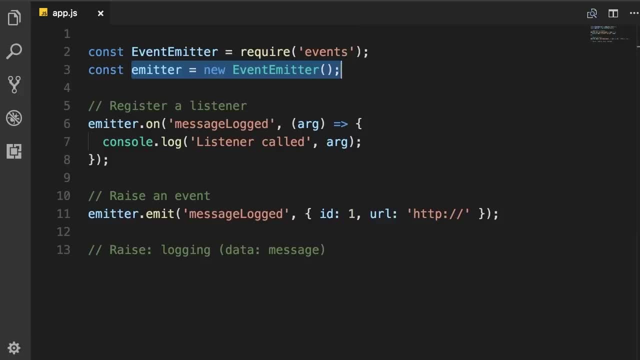 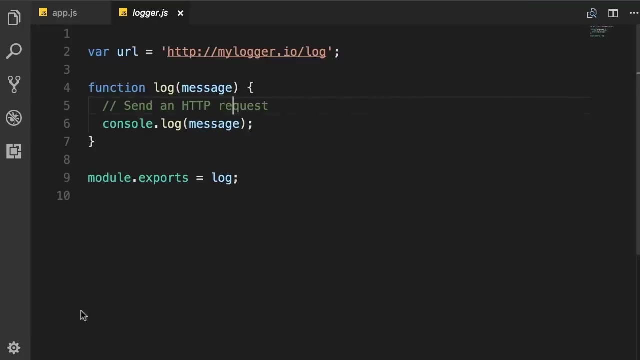 directly. instead you want to create a class that has all the Capabilities of the event emitter, and then you will use that class in your code. Let me explain what I mean by that and why. so let's open up our logger module. So in this module we're exporting a simple function- log right, and here we log that message on the console. 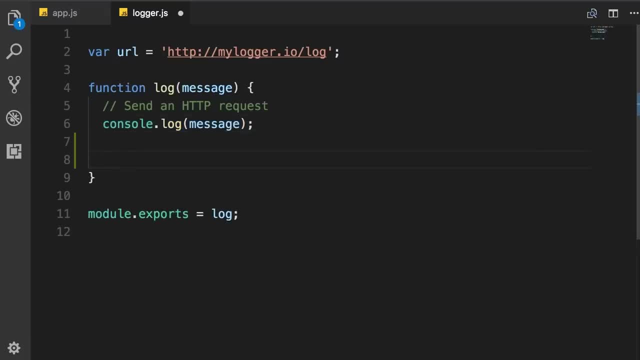 Now, after this, we want to raise an event and then later in app module We will listen for that event and do something. So let's go back to our app module And copy some code into the logger module. So on the top I'm going to copy these two lines: 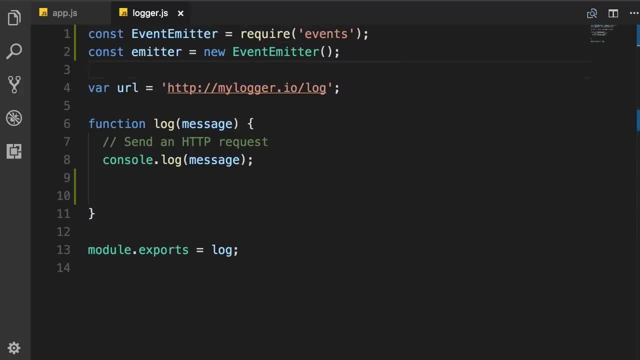 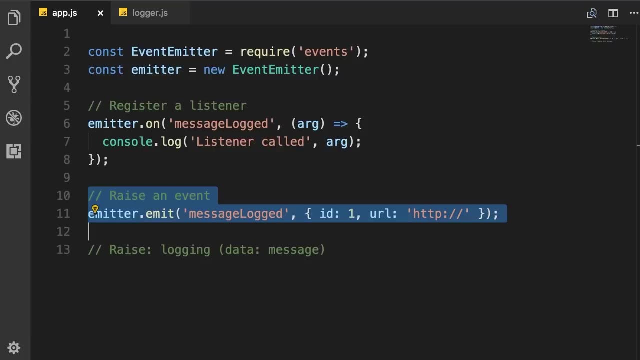 To bring the event emitter in this module. Okay, now back in app module. I'm also going to move these two lines for raising an event into the logger module, because this code should not be here. It's the logger module that emits or signals an event saying the message is locked, So cut. 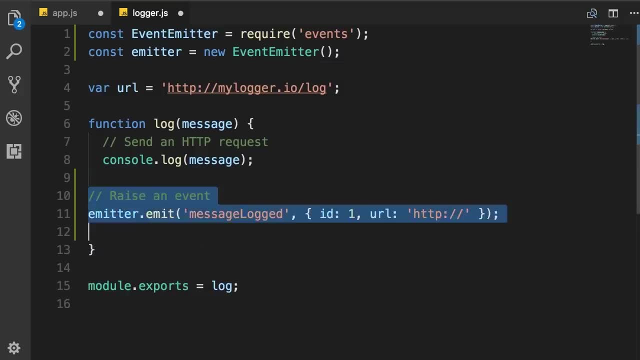 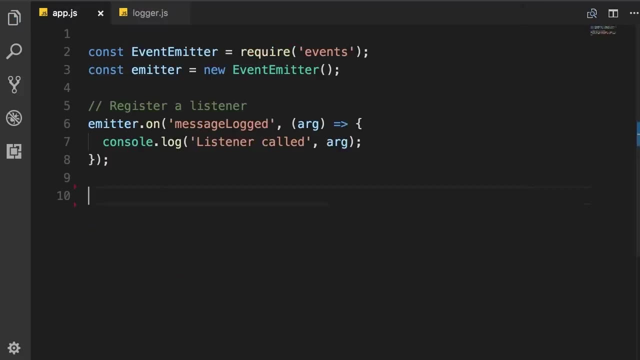 So here, after we log the message, we raise an event like this: Okay, now back in app module. We don't hit this comment here. We need to load the logger module and call the log function. So constant log. We call the required function and set the path to the logger module. 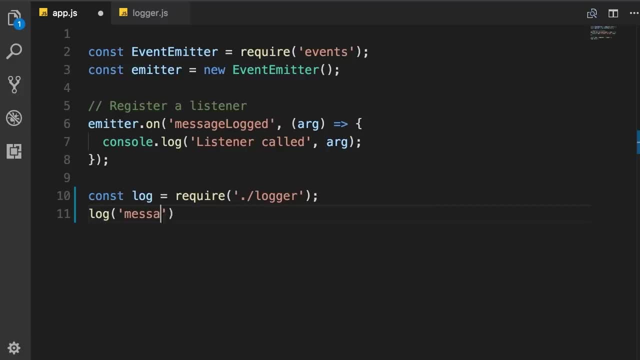 And here we simply call the log function with a message. Okay, Now when we run this application, we are only going to see this message on the console. In other words, this event listener will not be called. Let's verify that, and then I will explain why that happens. So back in terminal. 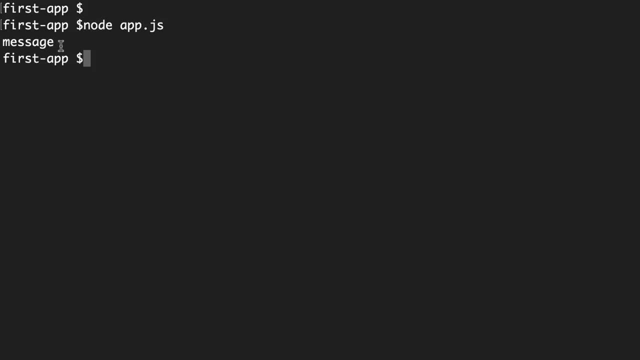 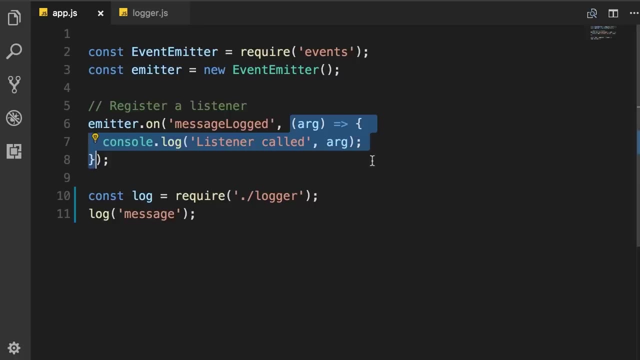 node appjs. Look, we only got the message on the console, So our event listener was not called. The reason for this is because here we are working with two different event emitters: In appjs we have this event emitter object and in logger module we have 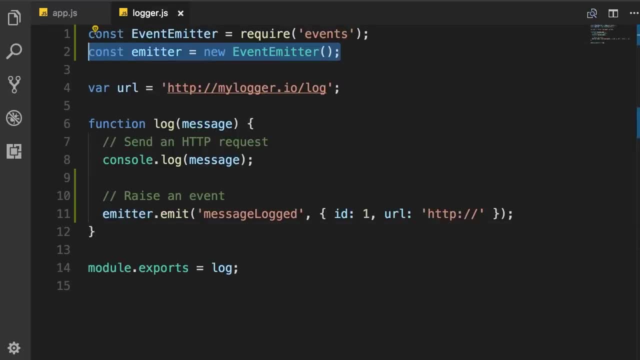 another event, emitter, object. So earlier I told you that a class is like a blueprint and an object is an actual instance. As a metaphor I said we could have a class called human or person, but the objects could be Jack, John. 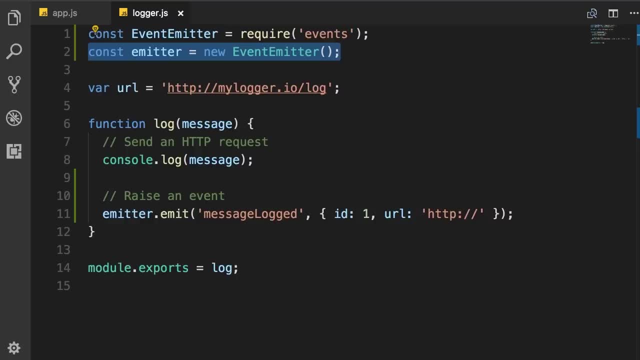 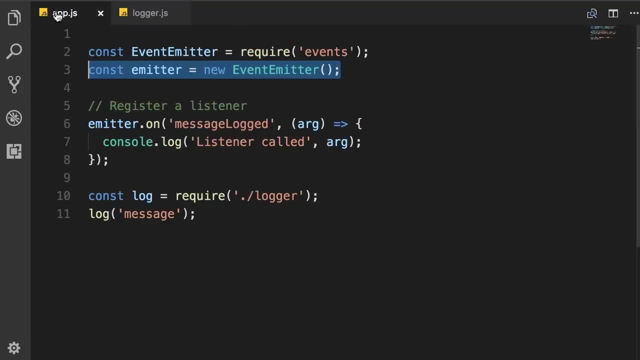 Mary Bob, whatever. So in this case we have two different objects. In the logger module, we're using this emitter object to emit an event, whereas in app module we're using another event emitter object to handle that event. These are: 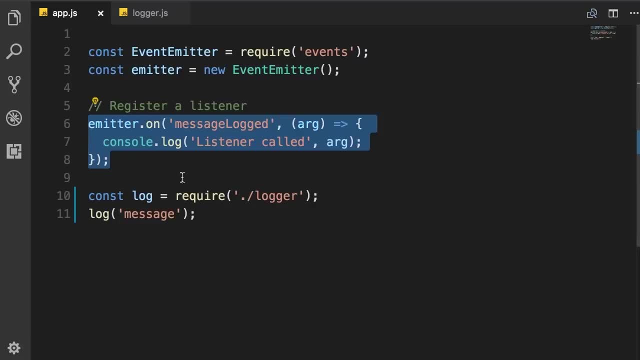 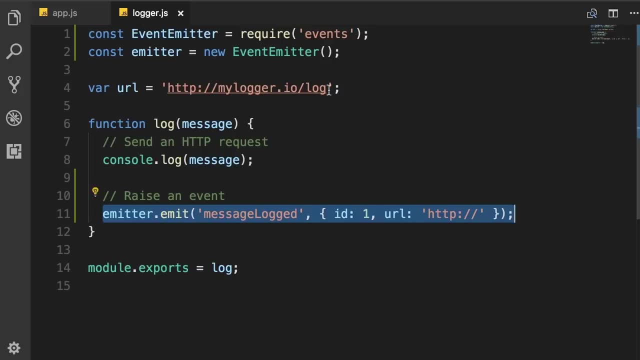 completely different. So when we register a listener here, that listener is only registered with this event emitter, which is completely different from the other event emitter. So that's why I told you in your applications- it's very rare that you would want to work with this. 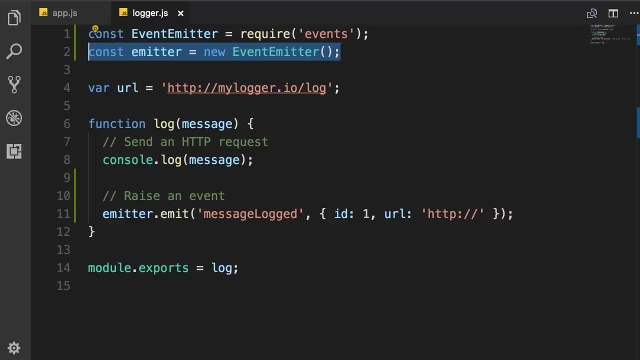 event emitter directly. Instead, you want to create a class that has all the capabilities of this event emitter, but it has additional capabilities. In this case, we want to create a class called logger that has this additional method: log. Okay, So the first thing we want to do here is to 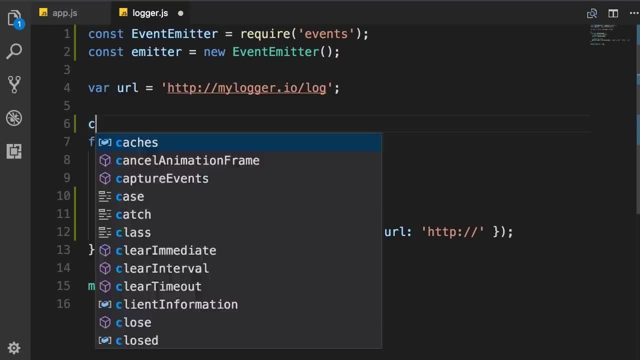 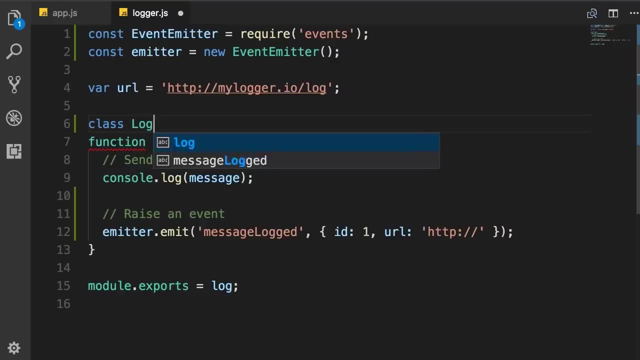 define a class. In ES6, we have this keyword class, which is a syntactical sugar. We're creating a constructor function. With this we can define a class logger. Note that the first letter of every word in a class should be uppercase. This is the Pascal case. 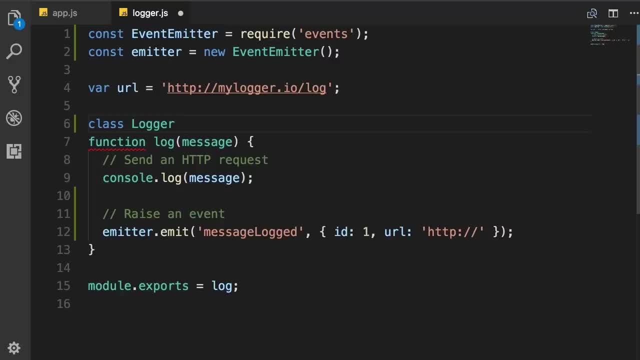 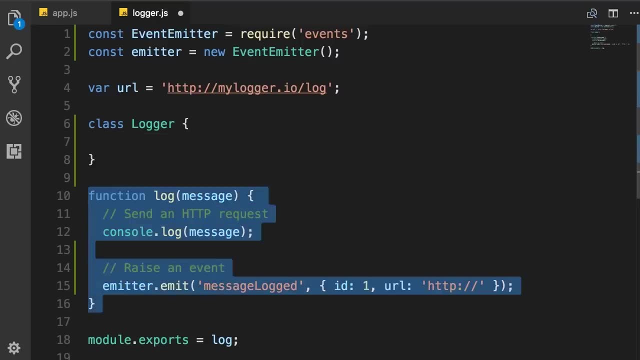 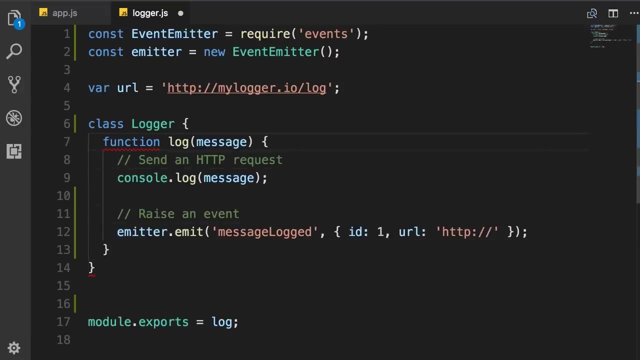 convention that we use for naming classes. So class logger. We have a code block. Now we need to move this log function inside this logger class. So cut Paste it here. Now we have an error because when we define a function, 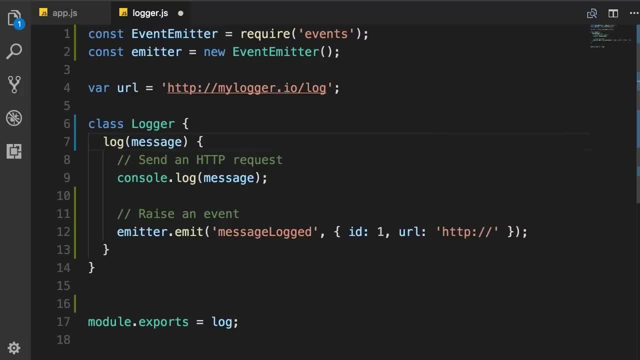 inside a class, we don't need this function keyword And from now on we refer to this function as a method. So when a function is inside a class, we say that's a method in that class. Okay, So here we have this logger class Now. 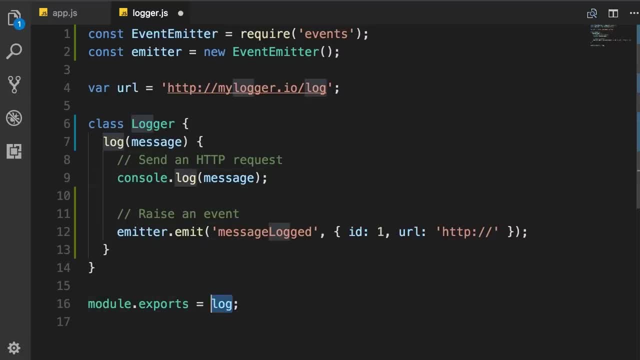 at the end. instead of exporting the log function, we're going to export the logger class. Okay, Now we want this logger class to have all the capabilities of this event emitter. The way we do that is by using the extends keyword that comes. 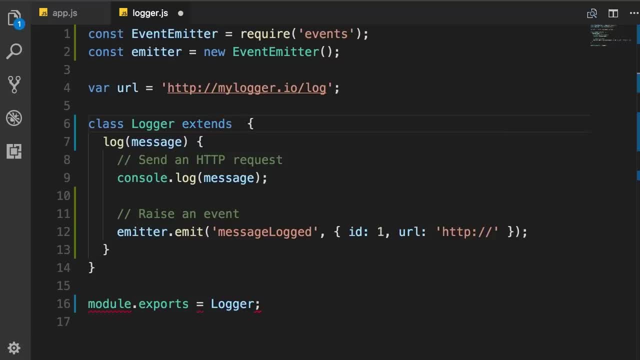 in ES6.. So extends, And here we add the name of the parent or the base class, So event emitter. And with this simple change this logger class will have all the functionality that is defined in event emitter. So here when raising, 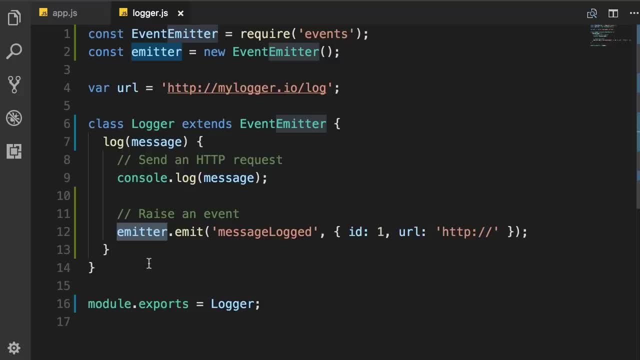 this event instead of using this emitter object. we're going to use this, So in this class we can directly emit or raise events. Okay, And now we no longer need this actual emitter object because we have not used it anywhere in this code, So delete. 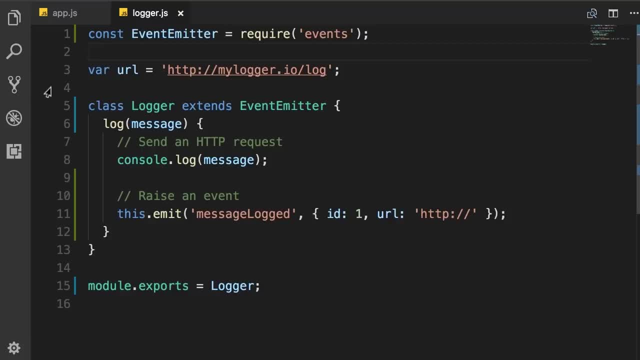 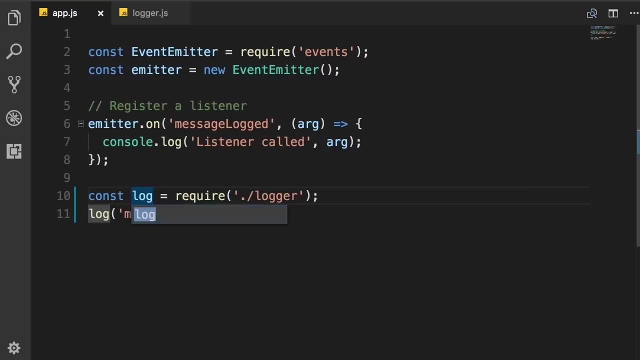 We're done with the logger module, Now back in the app module. So here, when requiring the logger module, we get a class. So I'm going to rename this to logger with capital L. That's a class. Now we create an object. 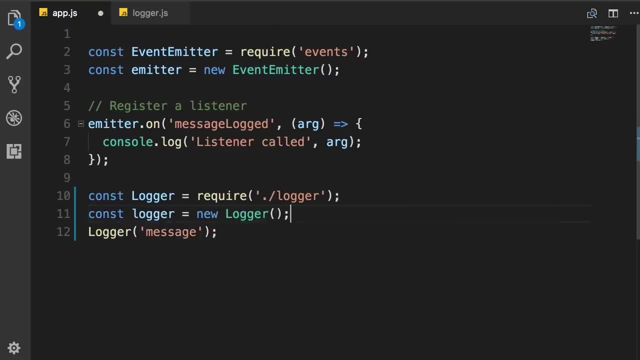 So new logger And then to log a message we call loggerlog. Now, similar to the change that we made in the logger module, we no longer need this event emitter object here. We want to work directly with this logger object, So we're going to register. 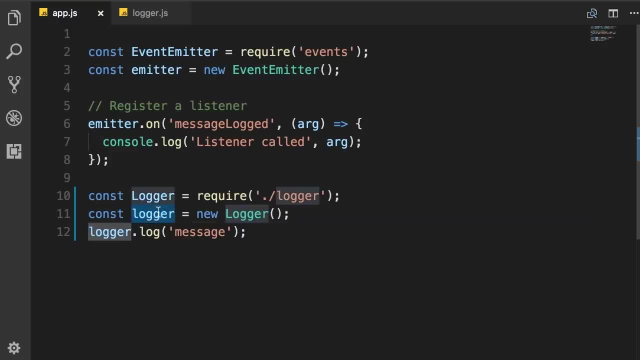 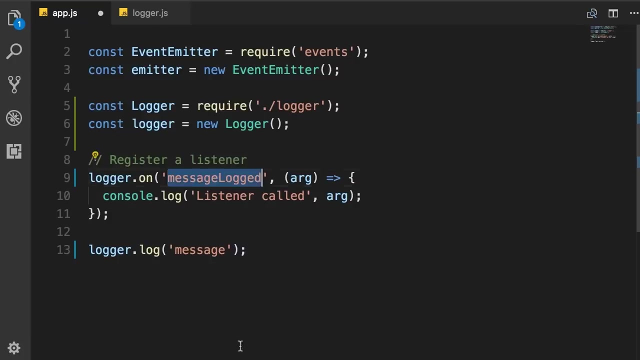 this listener on this logger object. Okay, So I'm going to move this code. after creating the logger, We say, hey, logger. when you raise this message- logged event- I want to execute this code. Okay, And finally. you can see. we no longer need. 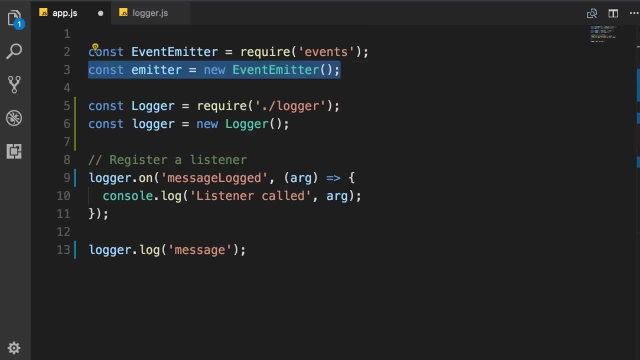 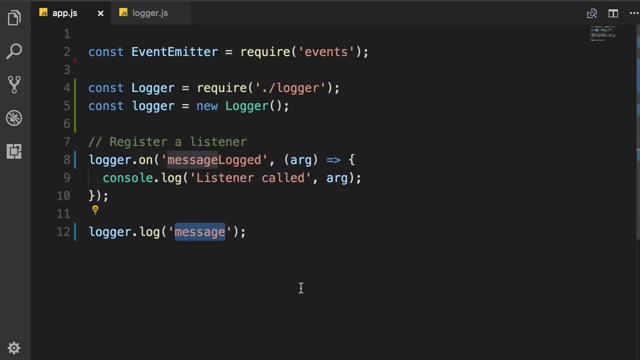 this event. emitter object: It's not used anywhere- Delete. Now, when we run this application, we're going to see this message on the logger object, So we're going to see this message on the console, But also because we're using 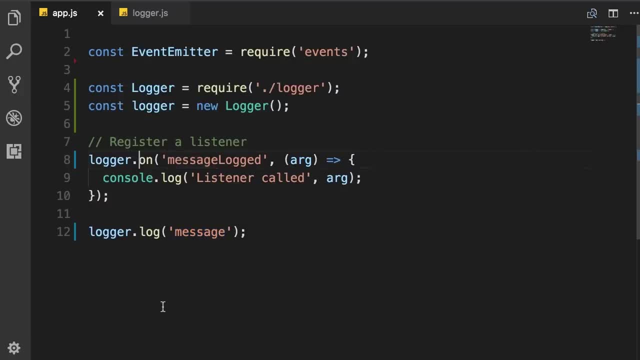 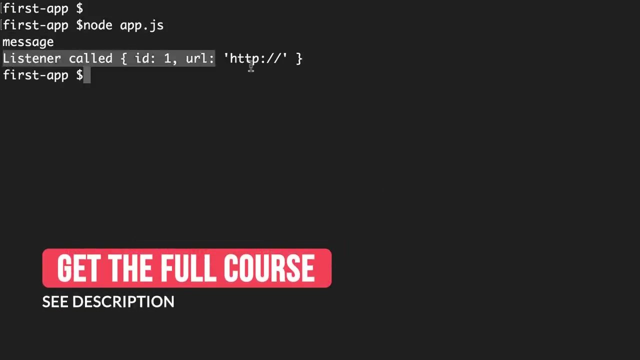 the same logger object for registering an event listener and also raising an event. we're going to see this message on the console, So node appjs. look, this is the message on the console and you can see our listener was successfully called, So let's quickly. 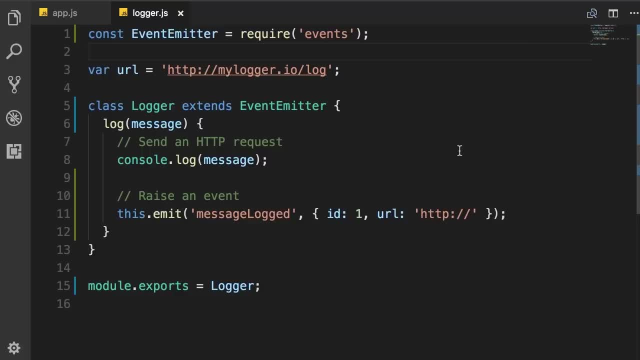 recap: If you want to raise events in your application to signal that something has happened, you need to create a class that extends event emitter. With this, that class will have all the functionality defined in event emitter, but you can also add additional functionality In. 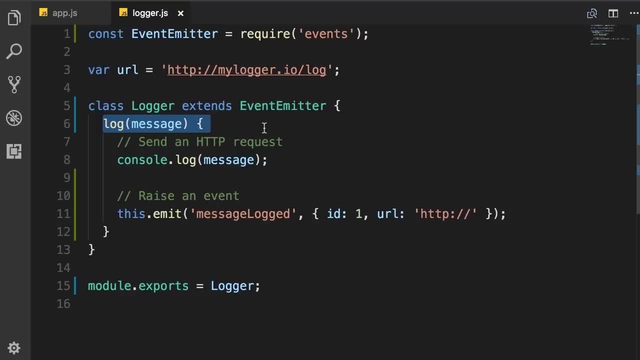 this case we have the ability to log a message And then, inside that class, whenever you want to raise an event, you use thisemit, because this references this logger class itself, which extends event emitter. So all the methods defined in event emitter will also be part of this class. Okay, 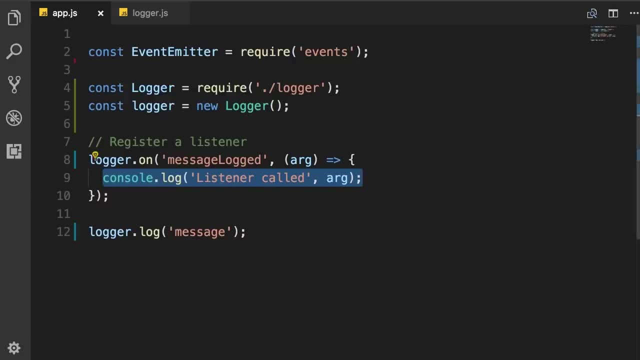 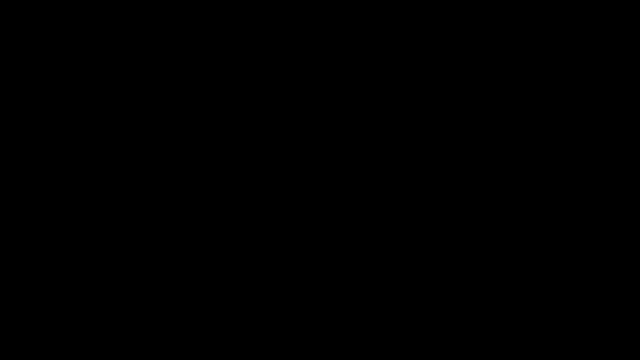 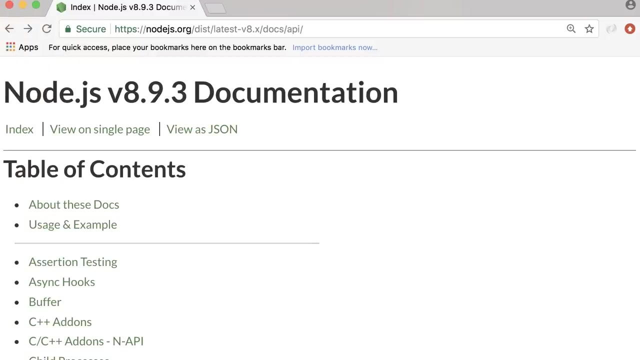 And finally, in app module, again, instead of using an instance of event emitter, you will use an instance of the custom class that you have defined that extends event emitter. One of the powerful building blocks of node is the HTTP module that we use for creating. 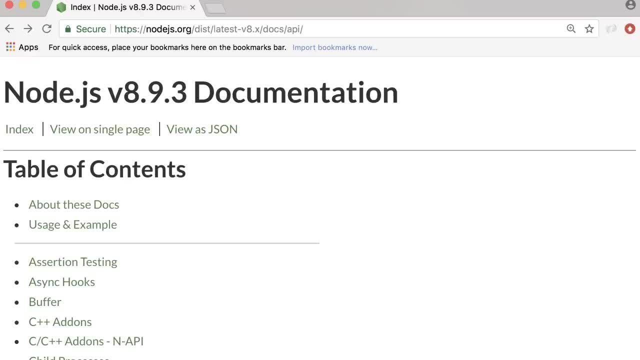 networking applications. For example, we can create a web server that listens for HTTP requests on a given port And with this we can easily create a backend service for our client applications, like a web application that we build with React or Angular or a mobile application running on a mobile. 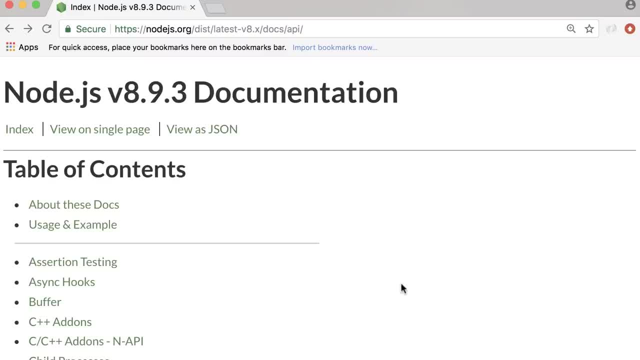 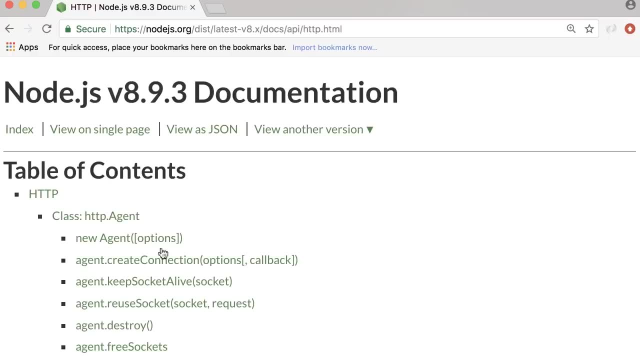 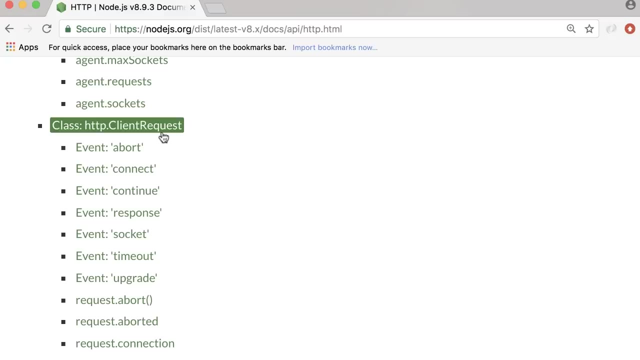 device. So once again back in the node documentation. in the list of modules you can find this HTTP module. In this module you can see various classes like httpagent, httpclientRequest and so on. Each of these classes has a bunch. 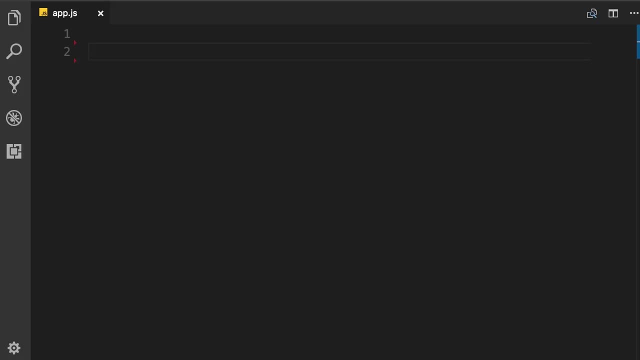 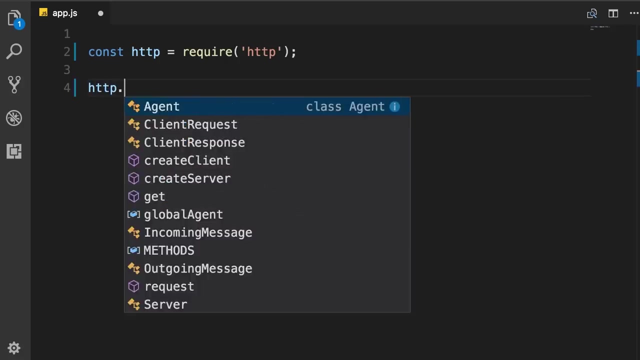 of properties, methods and events. So back in VS Code, let's load the HTTP module. So constant HTTP. We set it to require HTTP. Okay, Now here we can call httpcreateServer. This is one of the functions. 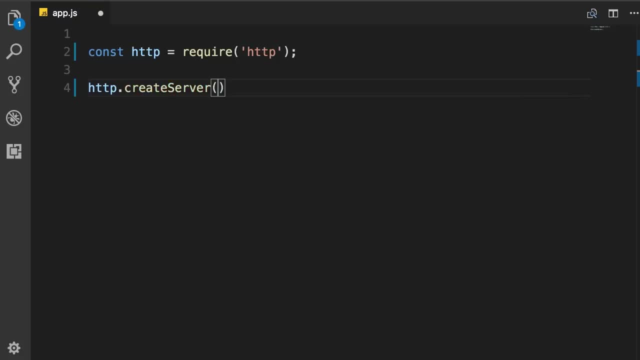 defined in this module, And with this we can create a web server. So let's store the result in a server object. Now what is interesting is that this server is an event emitter, So it has all the capabilities of event emitter that you saw earlier in this section. So look, server, We have the on method or add. 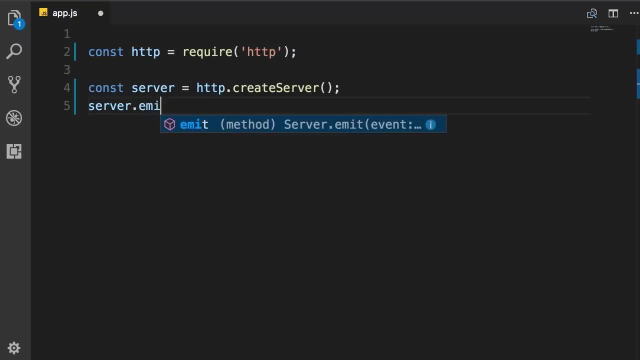 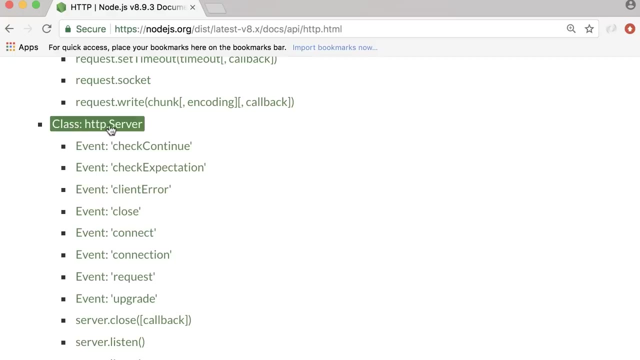 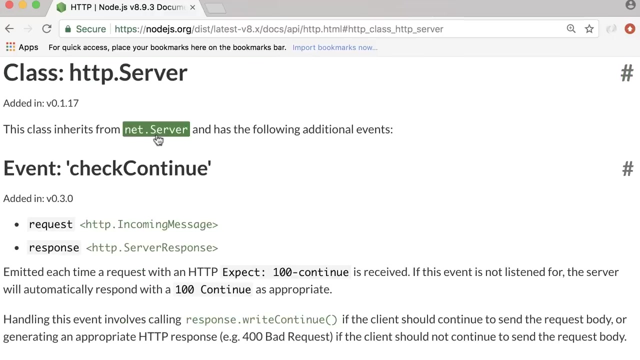 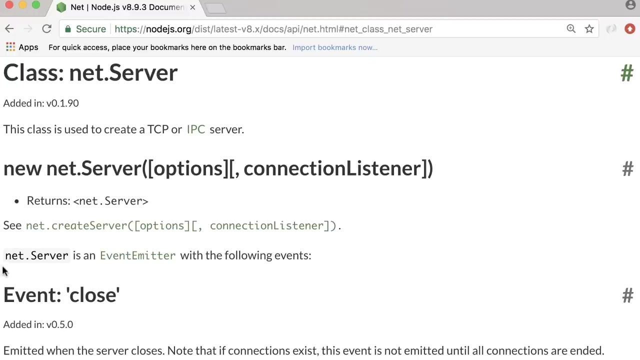 listener or emit and so on. If you look at the documentation for the HTTP module on this page, you can see httpserverclass. Here the documentation says that this class inherits from netserver. So this is another class defined in the net module. Let's have a look Now. here the documentation says that netserver is an event emitter. So that's why I said a bunch of nodes. core functionality is based on event emitter. 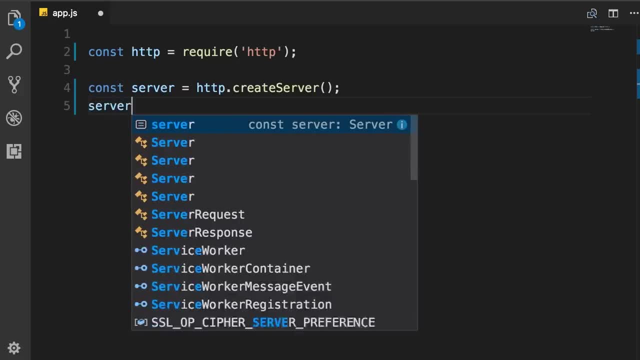 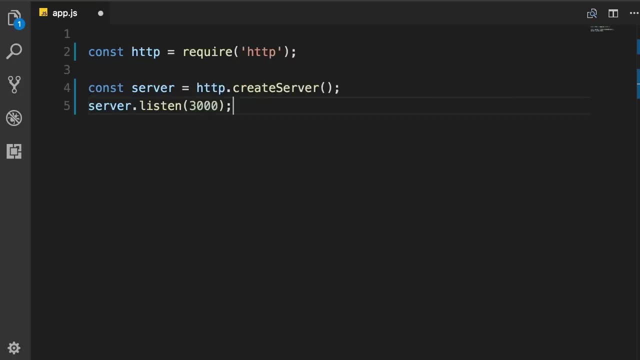 So back to our server object. Now we can call serverlisten and give it a port, Let's say port 3000.. Now, following that, I'm going to add a consolelog saying listening on port 3000.. Okay, Now when we run, 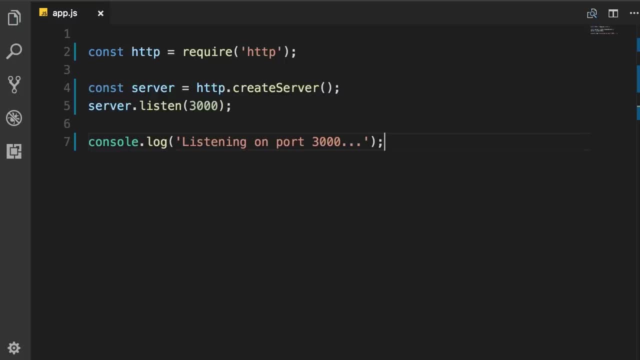 this application. this server will listen on port 3000.. As I told you before, every time there is a new connection or new request, this server raises an event so we can use the on method to handle that event. so before listening, we want to register a listener or a handler, so server dot on. 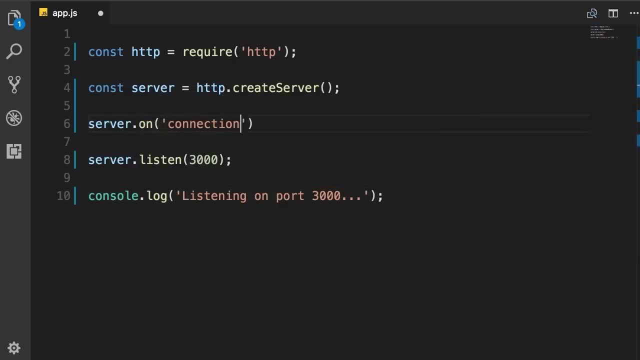 the name of the event is connection that you can find in the documentation, so you don't have to memorize any of this stuff. okay, and the second argument is a callback function, or the actual listener. as you can see in the tooltip here, this listener is a function with one argument, that is, socket, of type socket class, and. 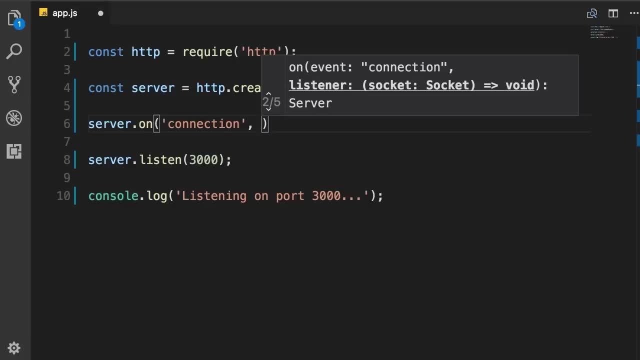 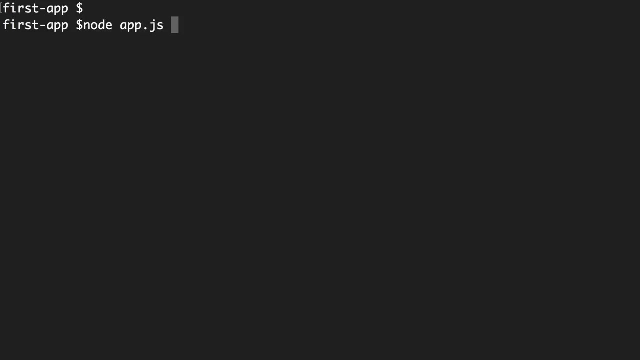 it returns void. so here we have the arrow function. syntax in es6. so let's add an arrow function that takes a socket and goes to this code block. now here we can simply lock something on the console. new connection- now back in the terminal. let's run this application. you can see we are listening. 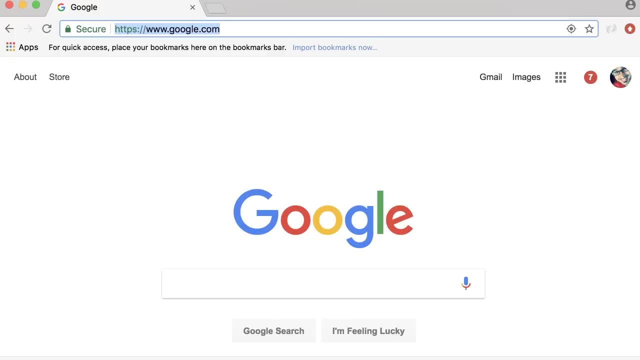 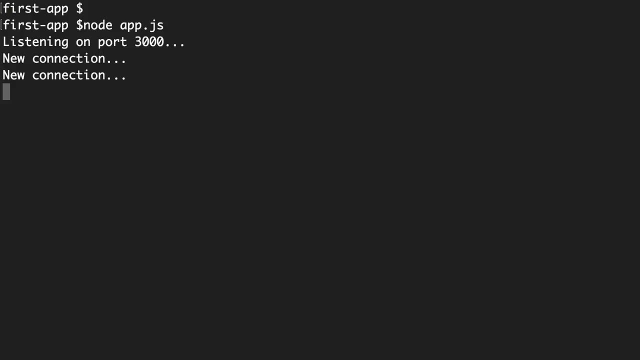 on port 3000. now, back in the browser, let's head over to local host port 3000. and now if you look in the terminal, you can see we have a new connection here. so you can see this server object raises different kinds of events that you can. 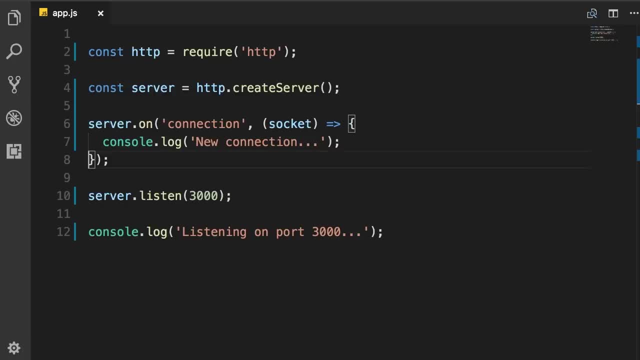 respond to now in real world applications. we are not going to respond to the real world applications. we are not going to respond to the real world applications. we are not going to respond to the connection event to build an H2TP service. this is very low level, so let's delete this. what we can only do is we 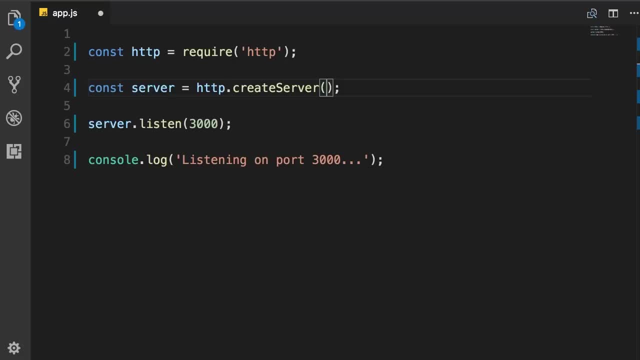 pass a callback function to this create server method. so function: this function takes two parameters: request and response. or we can use the arrow function syntax so we remove the function keyword and add this fat arrow. or we can use the arrow function syntax so we remove the function keyword and add this fat arrow here. 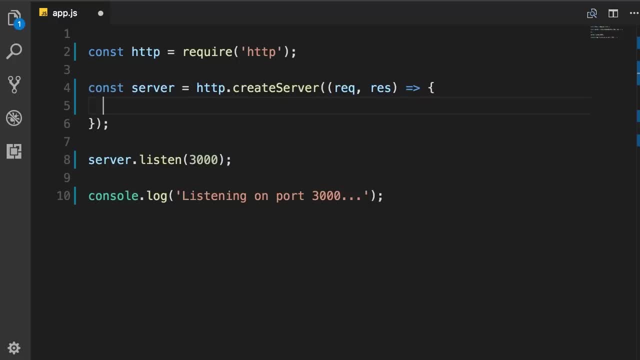 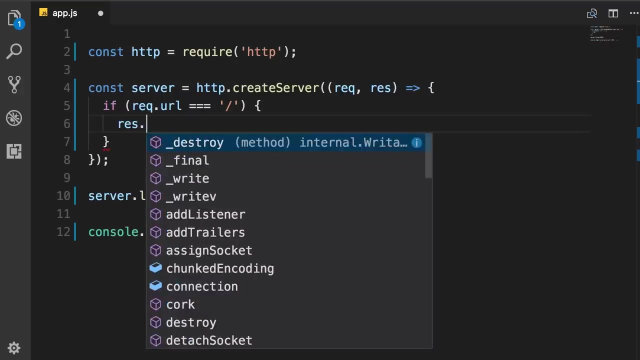 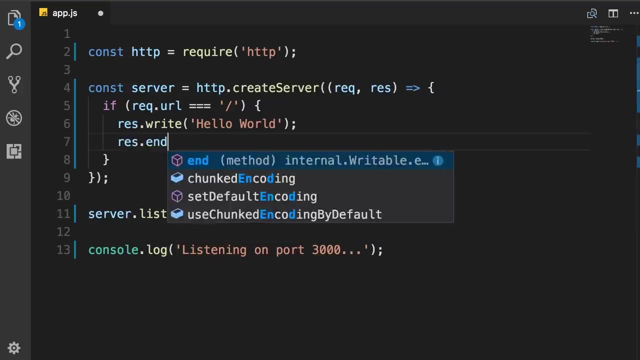 here Now in this function, instead of working with a socket, we can work with the actual request or response objects, So we can check if requesturl equals slash, Then we can send something to the client, For example, responsewrite hello world, And then we end the response. Okay, Now back in. 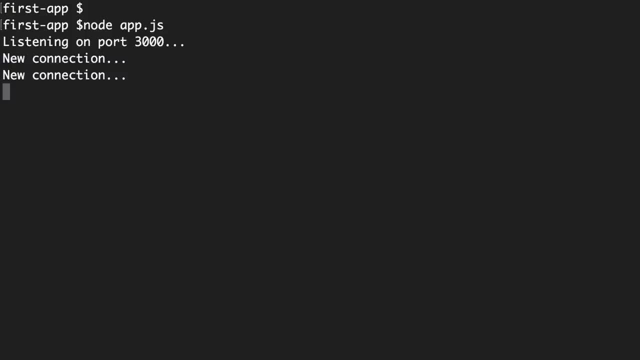 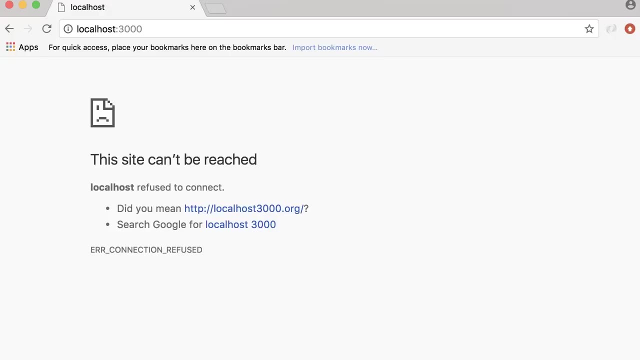 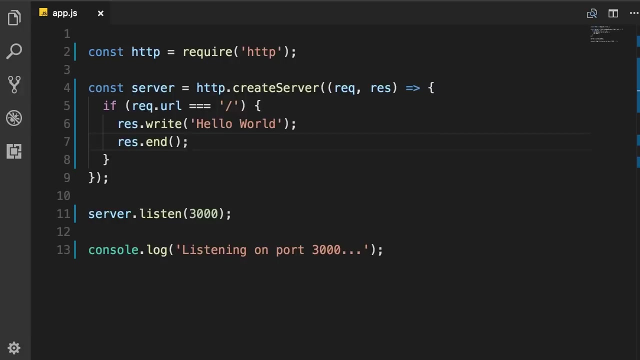 the terminal. we can exit here by pressing control and C and then run the application again. Okay, we're still listening on port 3000.. Let's refresh this page. So we got hello world on the homepage. Now, if you want to build a backend service for our web or mobile applications, we need to handle. 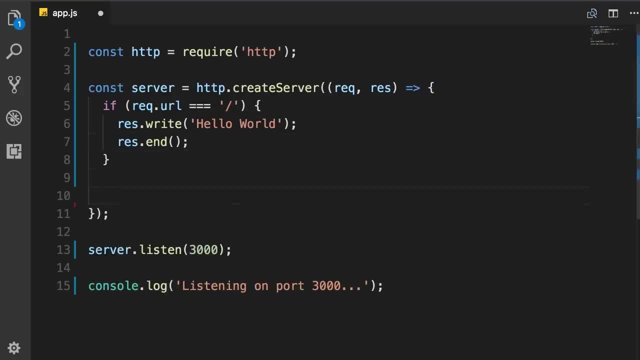 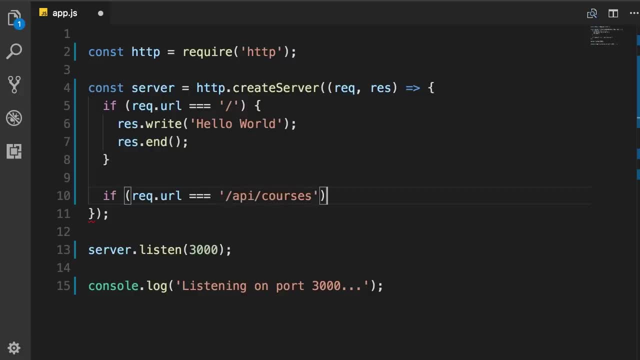 then we can add a requesturl, And then we can add a requesturl, And then we can add a requesturl. slash API- slash courses- Perhaps here we want to return the list of courses from the database, So we would do something like this response Right Now. here we want to return an array of objects. 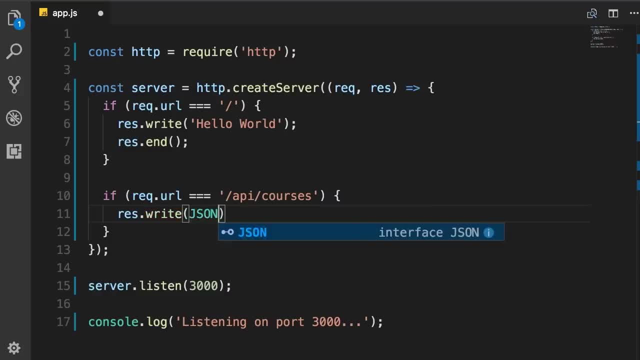 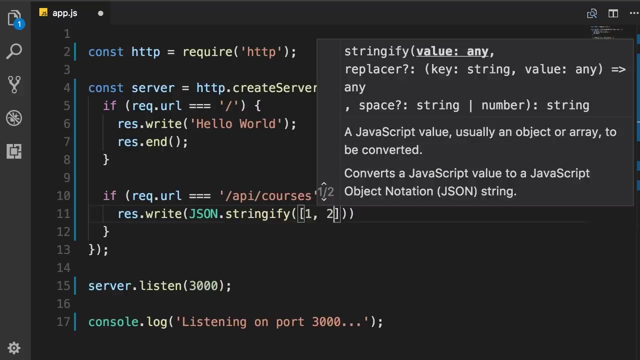 using JSON. So we use JSON dot stringify and give it an array of objects. Now for simplicity. here we don't have to worry about the database or complex objects. Let's just return an array of numbers One, two and three. So we pass this to JSON dot stringify. 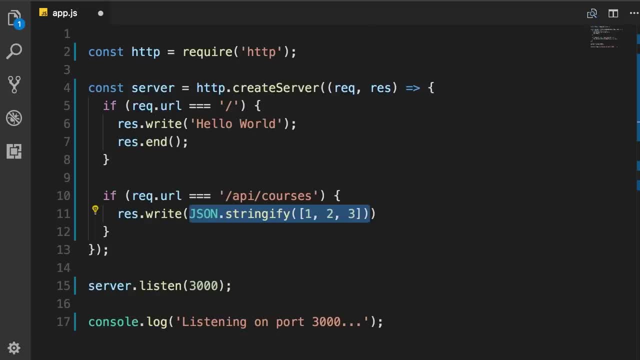 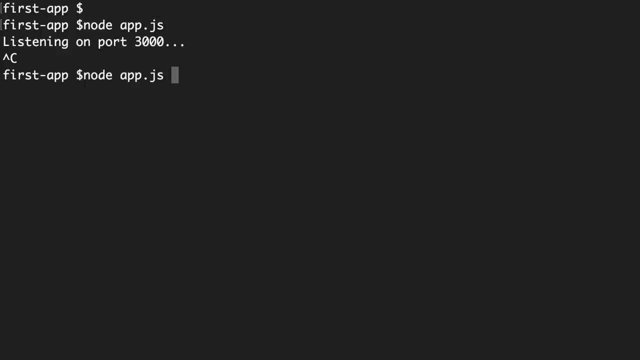 which will convert this array into a string using JSON syntax, And then we'll write it to the response And finally, response dot end. Now back in the terminal. we need to stop this process again and run it one more time Now. in the future, I will show you how we can automate this, So every 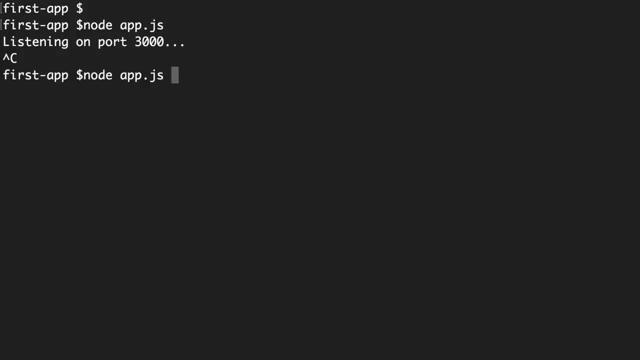 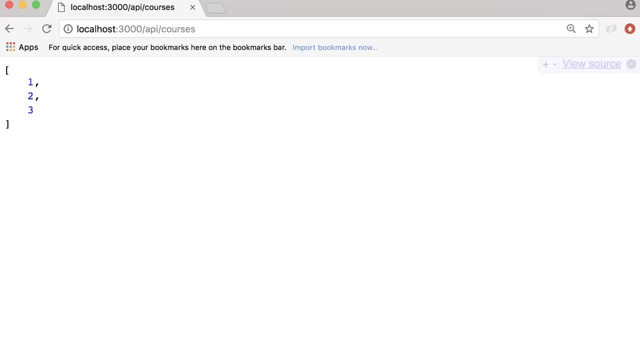 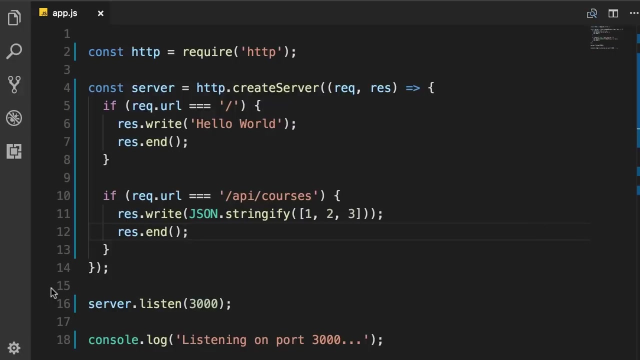 time we make a simple change to our application, we don't have to restart it. So now back in the browser. if we go to slash API, slash courses, we get an array with three numbers. So, as you see, building a web server, we know it is very easy. Now, in the real world, we are not going to use. 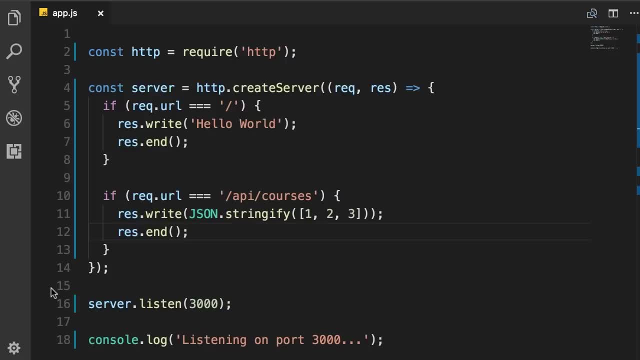 this HTTP module to build a backend service for our application. The reason for this is because, as you can see here, as we add more routes, this code gets more complex, because we add all of them in a linear way inside this callback function. So instead we use a framework called express, which gives our application a clean